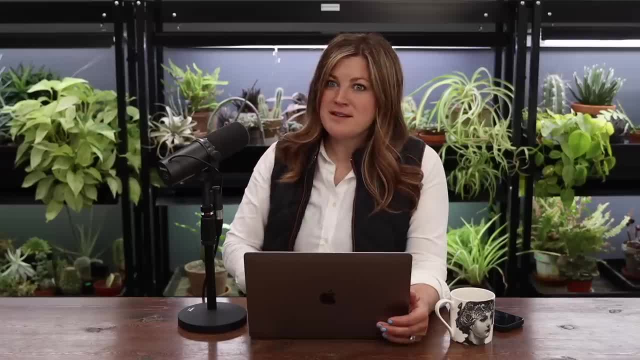 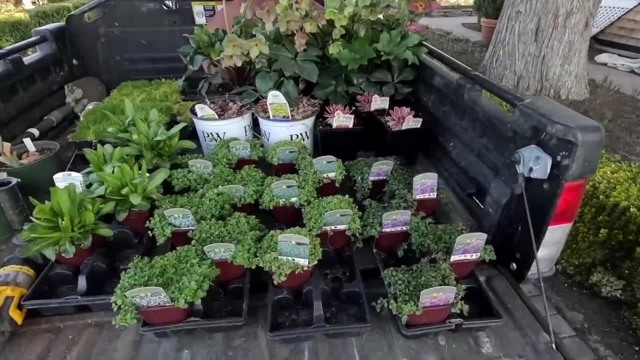 and money and fertilizer. It was perfect And we got a bunch of stuff done, which brings me to our first video, which was planting a bunch of ground covers and perennials. I just had a gator full of stuff, Some of the new ground covers we picked up down at the garden center Sedum. we had wintered. 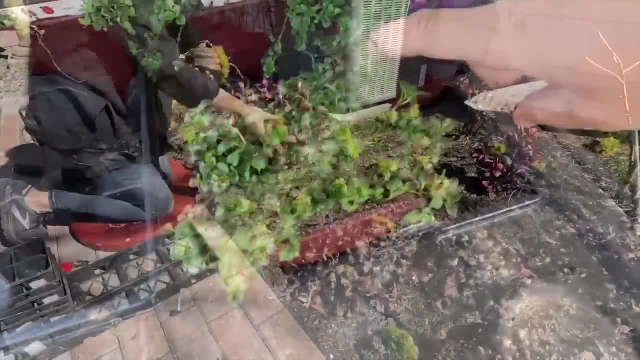 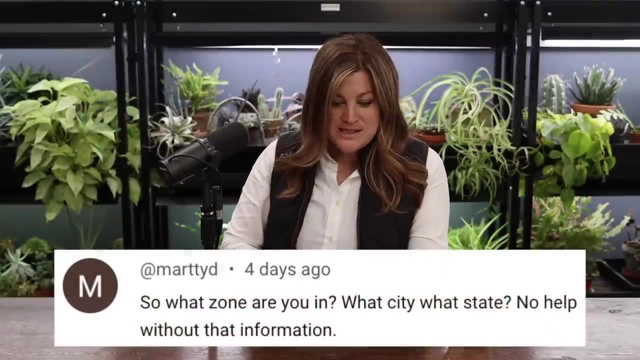 behind the greenhouse: some iris, uh, some sempervivums, I can't remember what else, but I felt like it was a really good load of stuff to get in the ground. Uh, so Marty said: so what zone are you, in What city? what state? No help without that information, which is probably true. I don't. 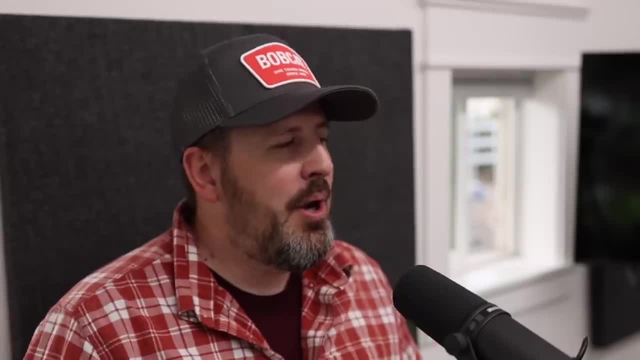 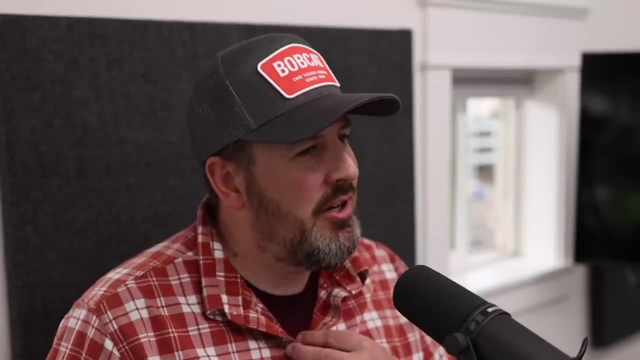 think to to add that in. We need to add it to the description of the videos somewhere. That is like kind of a legitimate thing, Cause I've watched videos where I've been curious, So I'm like I'm not a subscriber, I have no idea anything about that. 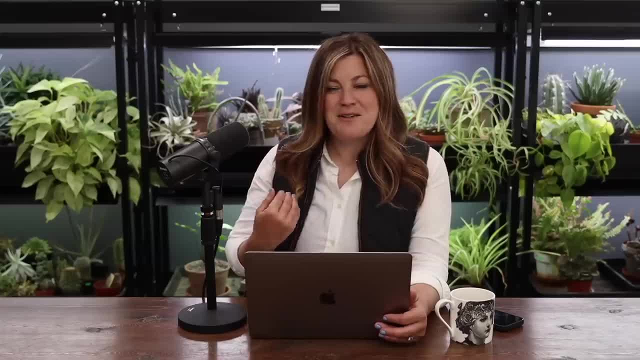 Um, but you want to know if it's applicable to yourself. I'll do some. I'll do like a little about me section or something in the description. Okay, That sounds good, Probably the best spot for it. We are in Eastern Oregon and we're high desert zone six. Amy deed said you are so smart. 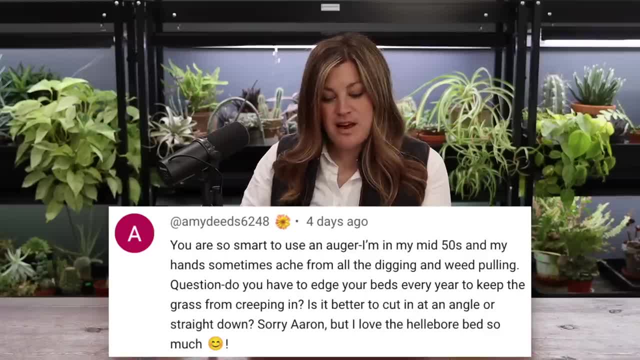 to use an auger. I'm in my mid fifties and my hands sometimes ache from all the digging and weed pulling. question: Do you have an edge? Do you have to edge your beds every year to keep the grass from creeping in? Is it better to cut in at an angle or straight down? Can I mean it might help to do it once a year with, like the step edger, but it's really just a matter of trimming every week. You're probably- if you have grass, you're probably- trimming with a weed whacker anyway. So just put it on its side and trim vertically. You could go at an angle if. 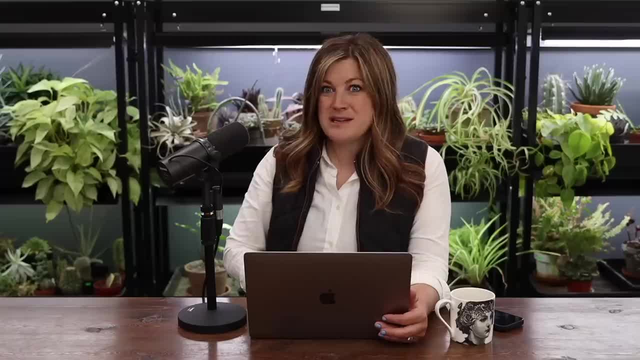 you wanted to. if you like that, look, but we do it vertically. Keeps it in check. Yeah, Like I don't really feel the need to Might have to pull a little bit of grass. that kind of creeps in Occasionally. 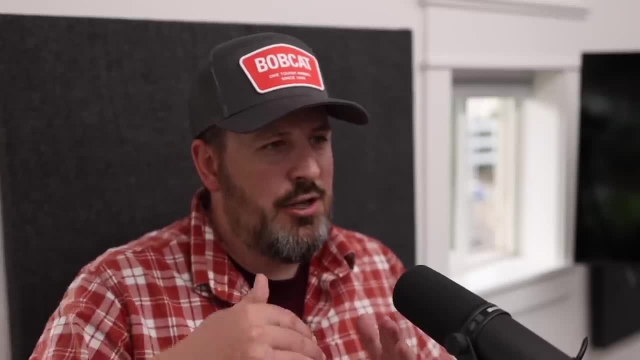 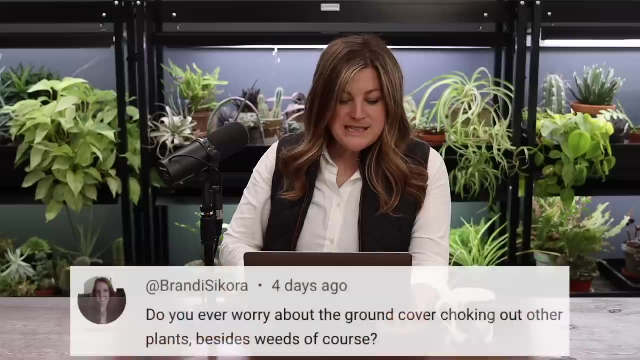 but not a ton Like. sometimes. there'll be a little grass that's like you've got your edge, and then there's a little grass that'll grow like a couple inches away from the edge. Yeah, Into the flower bed You might have to pull that. Yeah, Brandy said, do you ever worry about the ground cover? 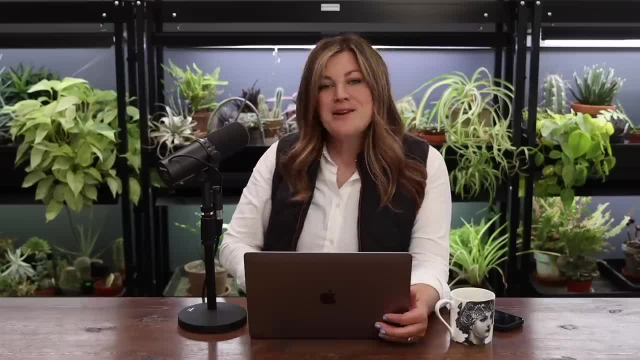 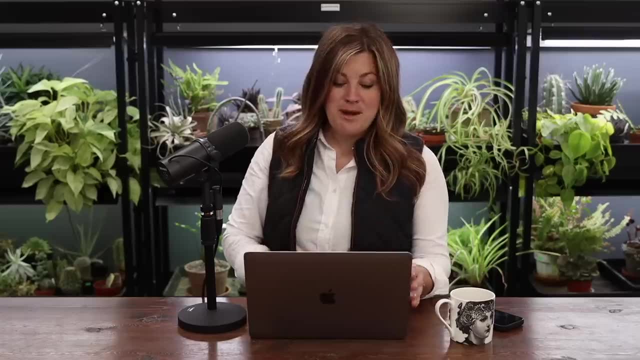 choking out other plants besides weeds, Of course. Uh, you know, I don't really worry about it. I've had my fair share of mishaps when it comes to ground covers. Like you know, in our very first garden spot right after we got married, we were renting a townhouse that had this little tiny. 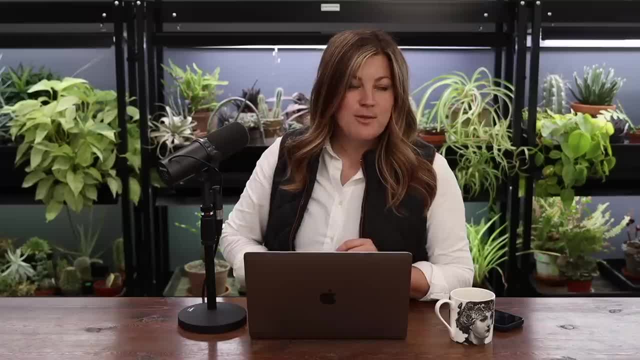 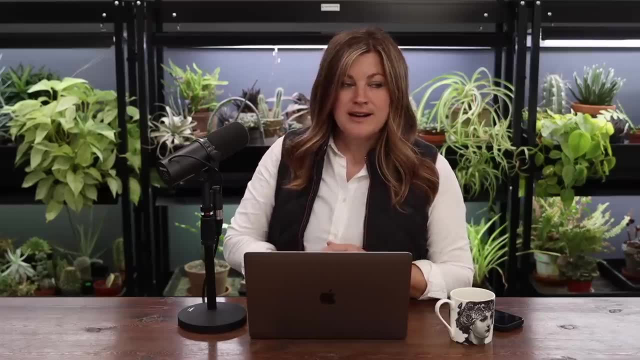 garden space and I planted one mint plant in there And that, while some of them are, I guess, considered ground covers because they stay really low, uh, all mint plants will stay really low, Spread like wildfire, And that was a hard one. Um, I planted sweet woodruff once, So in my 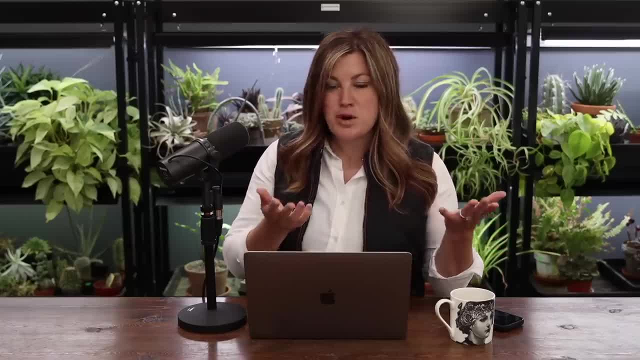 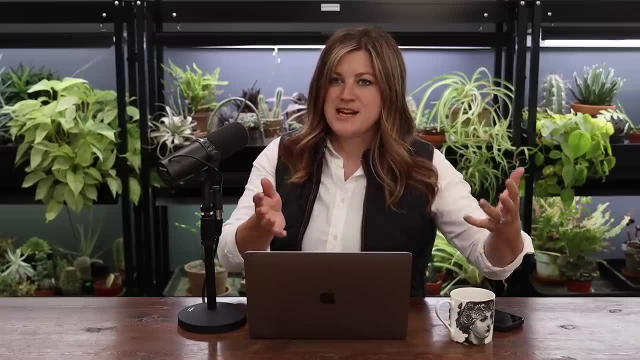 parents' garden. it was gorgeous And I thought I need that in my garden because it's perfect, Stays nice and compact. It just very- um, not unruly Like. it was very tidy, I guess, but theirs was planted in fairly deep shade And I just thought that when I planted. 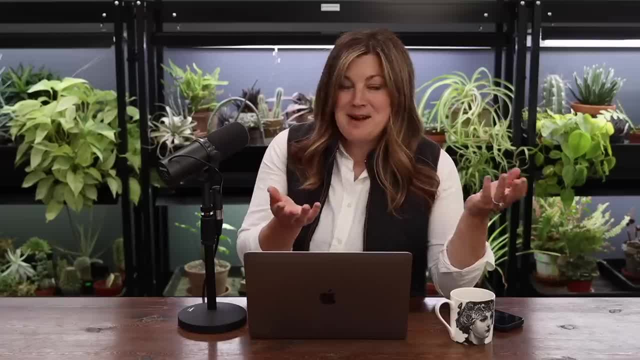 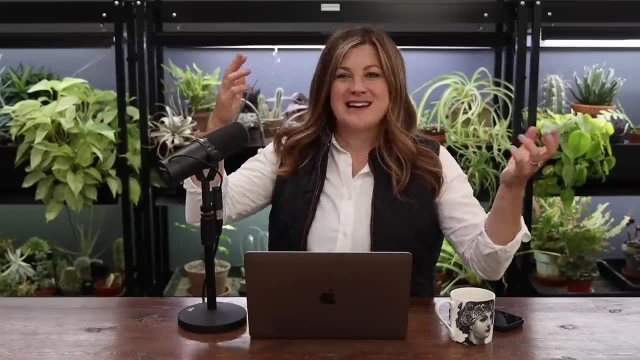 it in our garden, where it got sun for a good portion of the day, that it would be the same And that stuff grew so tall It didn't look anything like I wanted it to look. when it gets really tall, Then it kind of like gets a little like. it looked messy to me and it took over It. 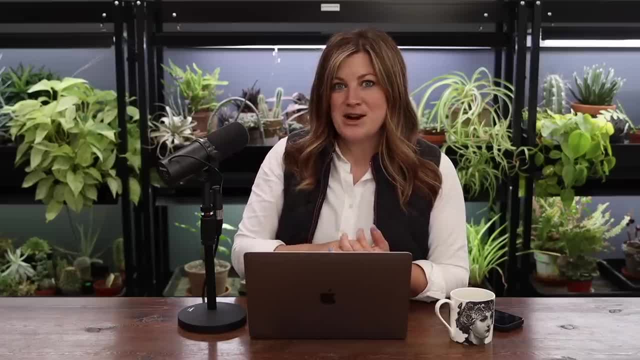 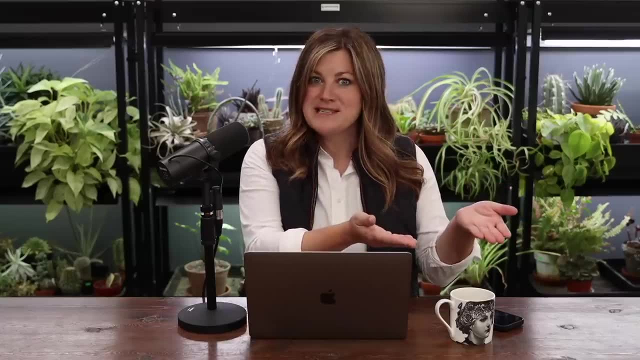 just spread everywhere. Um, so I've had a few things take over that I didn't really want to have take over, And sometimes it's trial and error, because you could look in somebody's garden and have it be this beautiful little dainty plant. Then you put it in yours and it just like takes. 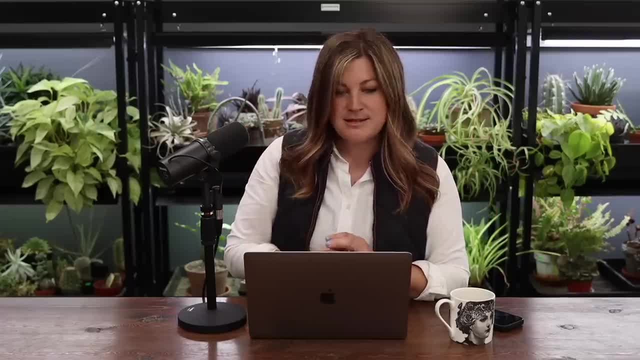 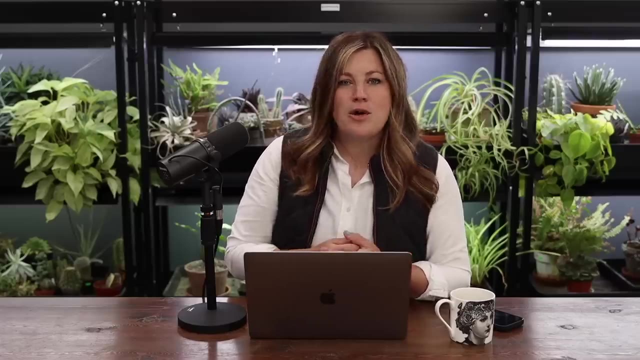 off and explodes. You know. there are some, though, that are just amazing, Like the Veronica, like lamium is an amazing ground cover. Lamiastrum is also really good. Chamomile or chamomile- chamomile, It's also really good. Um, so yeah, I don't know. I don't really worry about it too. 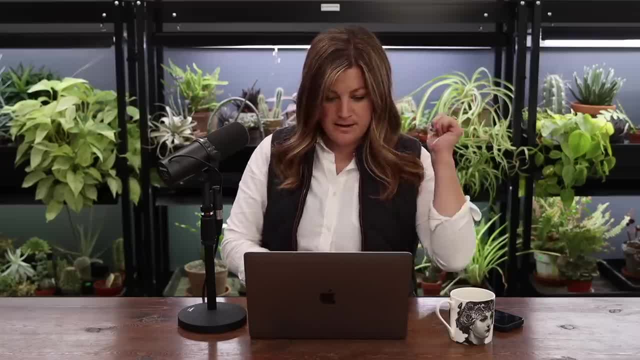 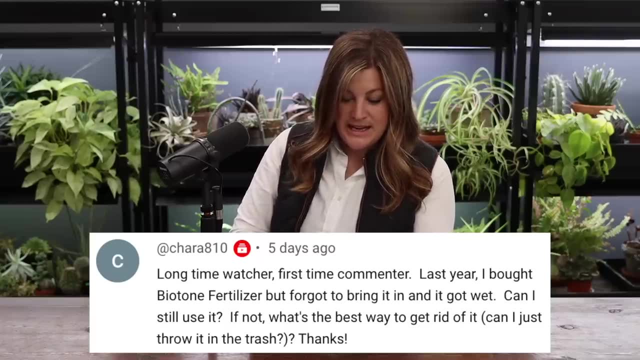 much If it's. if something starts to become unruly and it becomes a headache, then out it goes. Shara said: long time watcher, first time commenter. Last year I bought biotone fertilizer but forgot to bring it in and it got wet. Can I still use it? If not, what's the best way to get? 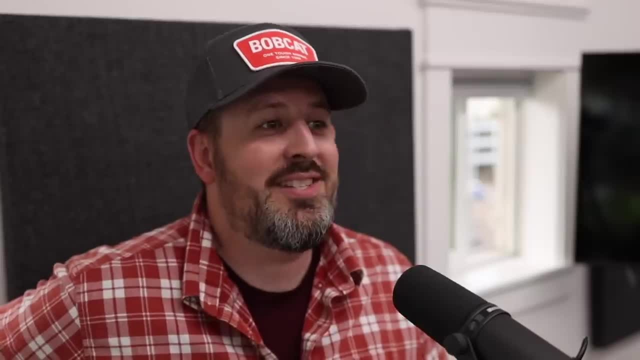 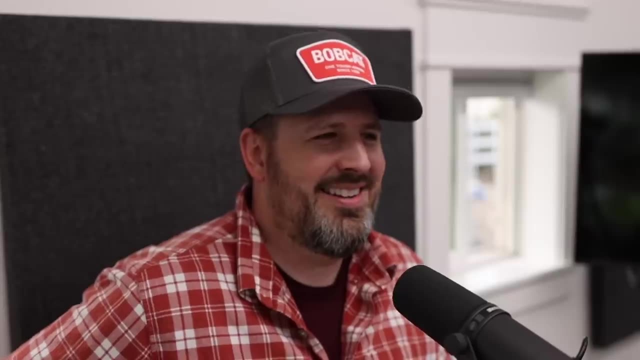 rid of it. I would just use it. I've done that several times. If you can stand the smell, Well, it depends A biotone that's been just lightly wet, like wet, wetted down, Sure, Uh, watered down, I don't know, Rained on. That's in our case. Um, it'll like clump together and it'll come out of the bag and clumps, which is kind of a pain and you kind of have to use something to break it up. But if it's been like deluged with water and then left to sit at the bottom of a pallet like some of our bags, it smells like something. 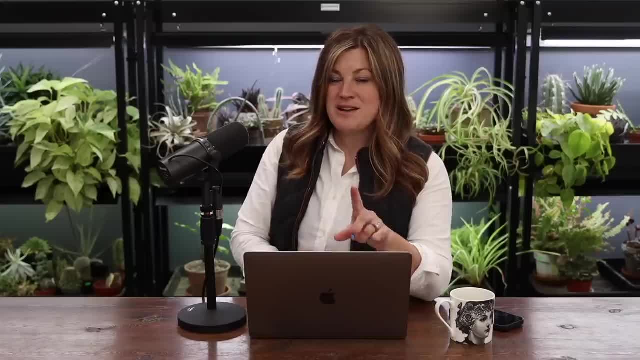 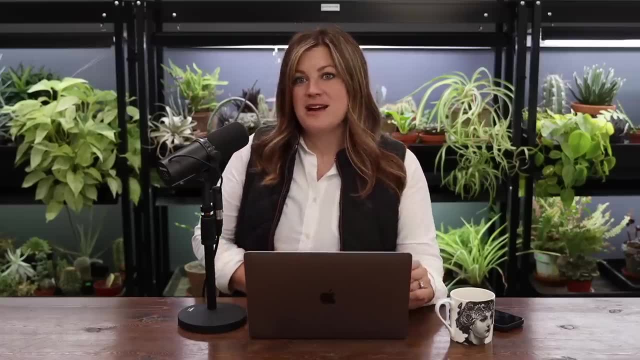 died. Yeah, That's not happened very often. The first time it did, I was looking around like legit. I just thought something is dead out here. What is that? And I searched all over the place to find out. it was my bag in the back of the gator And I did. toss that one, because there was no way I did not want that perfuming the air. Yeah, You know I, I fertilized the lawn last year, the year before, with a bag that smelled like death And in my mind I was kind of like, you know, I wonder if this is going to be like extra good. 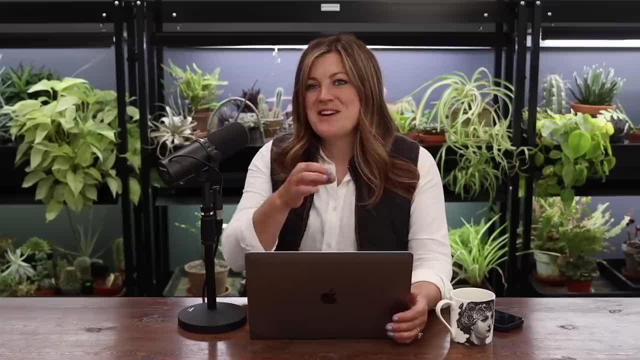 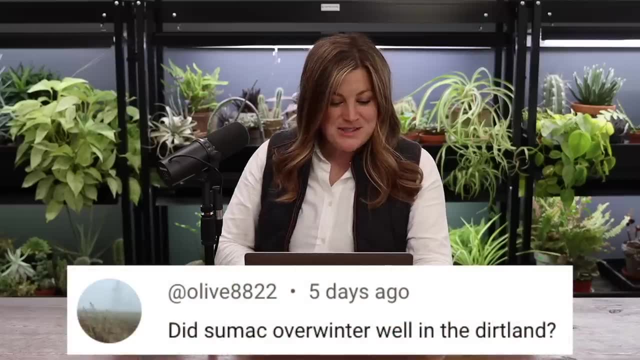 for the lawn. There's a part of me that just thinks like the worst. the worst it smells, the better it must be. I don't know. Olive said, did the sumacs overwinter well in the dirt lands? You know, time will tell They look. 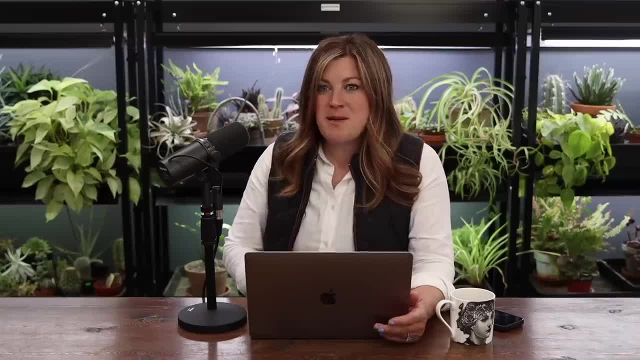 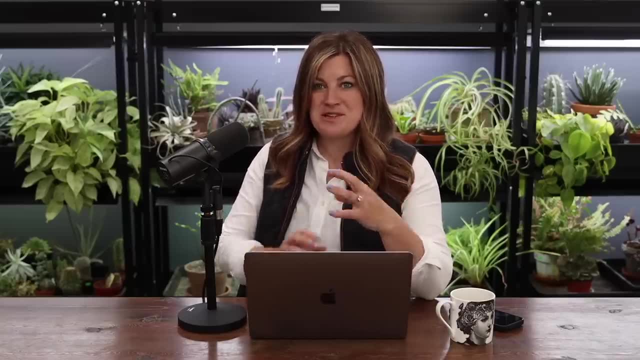 good, They look like my other sumacs do. So we'll see. They barely had any root system, I'll bet they'll take. I mean I was surprised they were standing upright because you guys saw the root systems on those. I mean they were just like these tiny little things, Sumacs. I feel like. 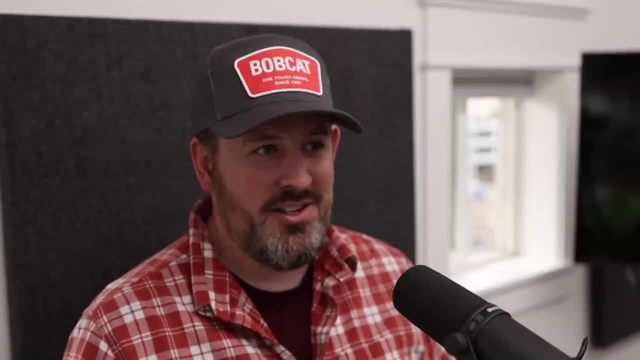 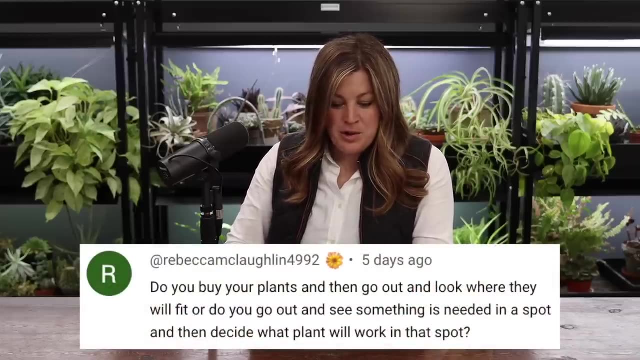 you could just cut them at any point and just stick it in the ground. As long as it had some moisture, it would just Perhaps. Yeah, that's probably true. Rebecca said: do you buy your plants and then go out and look where they will fit, Or do you go out and look at the? 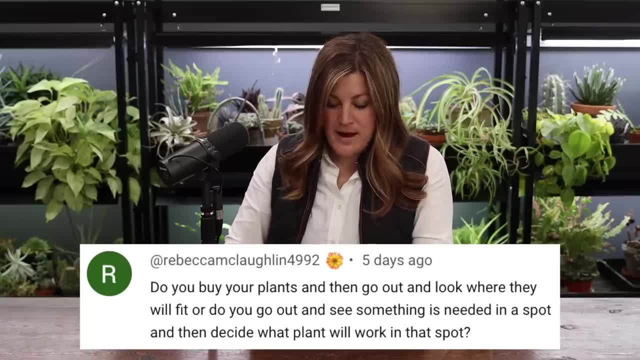 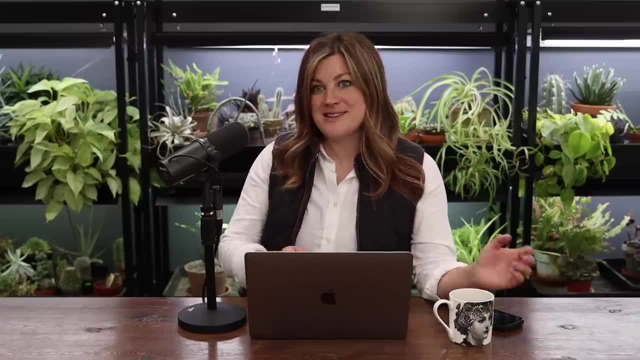 and see something is needed in a spot and then decide what plant will work in that spot- Both I need a good mixture of both. There are some spots like out in the South Garden we're starting to get full with big things that are going to get big, But there are a few little. 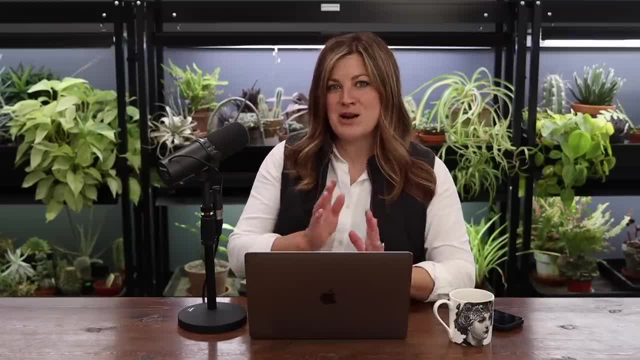 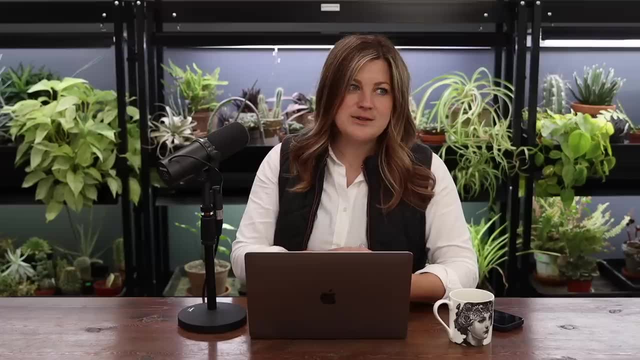 spots where I think that needs an evergreen And I just haven't decided which one yet. So I leave those spots open until I find the right plant. When I'm doing perennial drifts- depending on if I need to, I don't know. oftentimes I know what color I want to do next, You know there's. 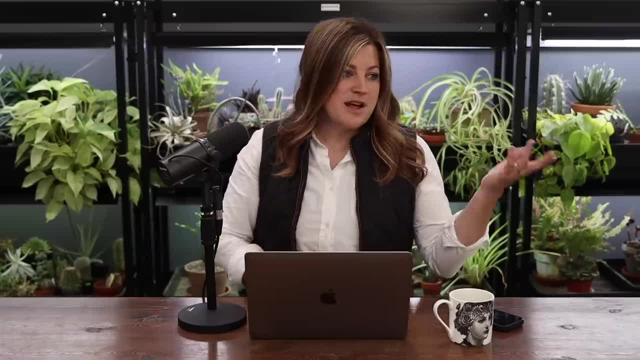 one corner I'm just doing the pinks, purples. And then there's other areas where I like to just kind of make sure it's a good mix And I'm not putting two purple things next to each other, that there's like a pink and a white and a purple. 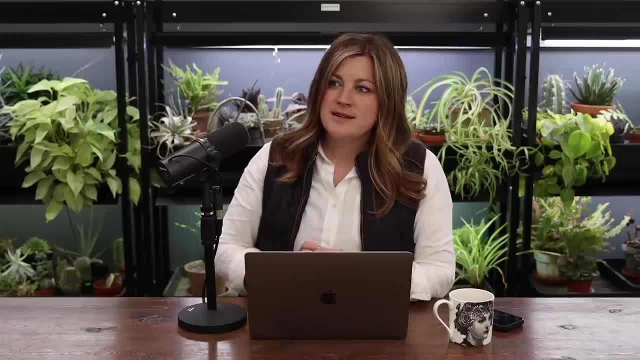 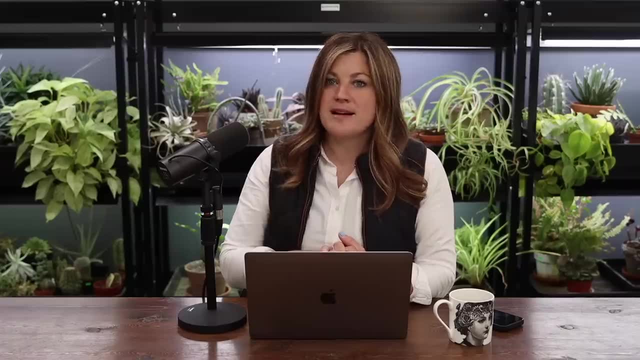 maybe a pale yellow and an apricot, and then kind of repeat. I don't know. But there's times where I fill up the gator, like this time, and I had no idea where anything was going to go. I just go out there and find a spot, And that's the beauty of the South Garden is that we don't have a plan. 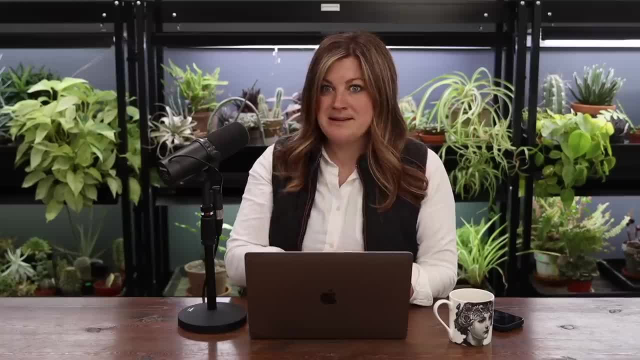 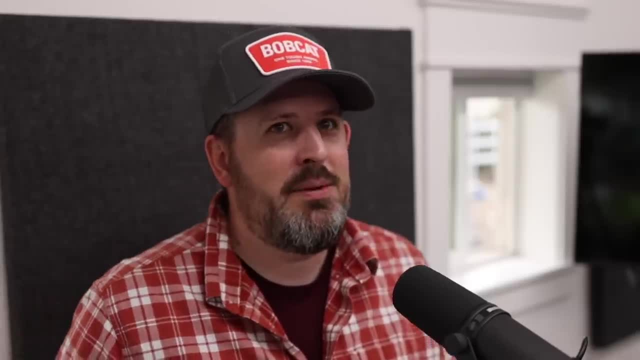 There's zero plan out there. It's just like toss it out there and see how it comes together And hopefully it looks good in the end And it's coming along. I feel like you have enough. I don't know Some people. they make it just seem effortless And 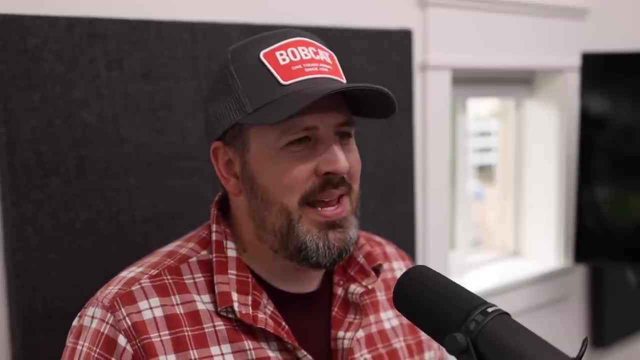 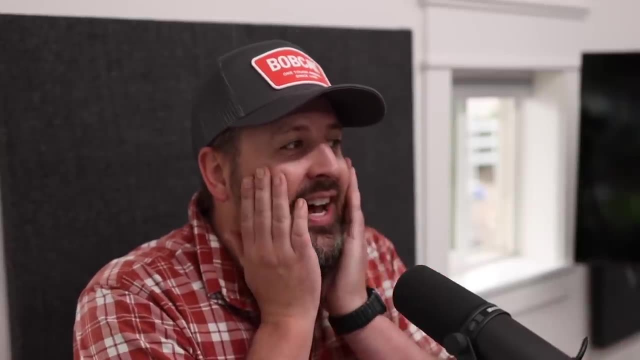 you're kind of one of those people Like if you watch Bob Ross paint, the way he explains painting is like oh yeah, you just do it, man, You know. and but it's like no, if I, if I tried to attempt. 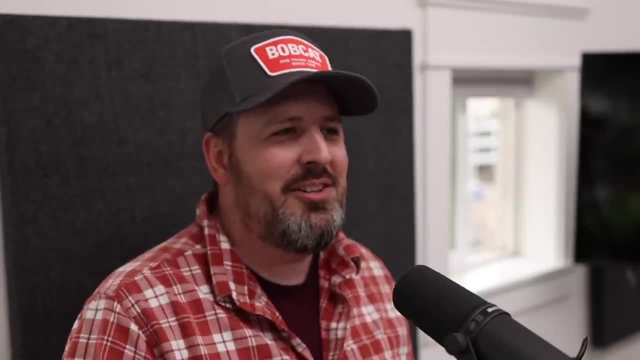 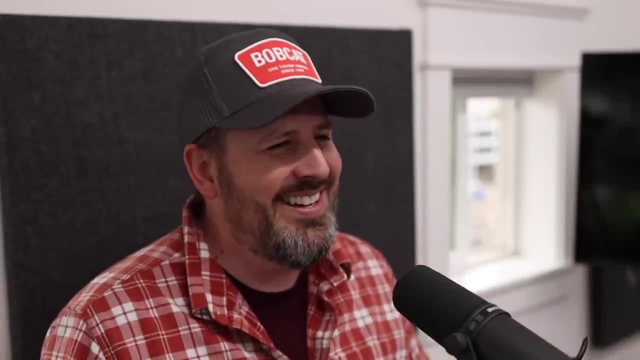 what you're doing. it would just look like total trash. And I feel like you're a little bit the same with with gardening. It's like, oh yeah, there's no plan, We're just going out there willy nilly. But it's like, OK, well, but hold on. Maybe there's more of one in my brain. 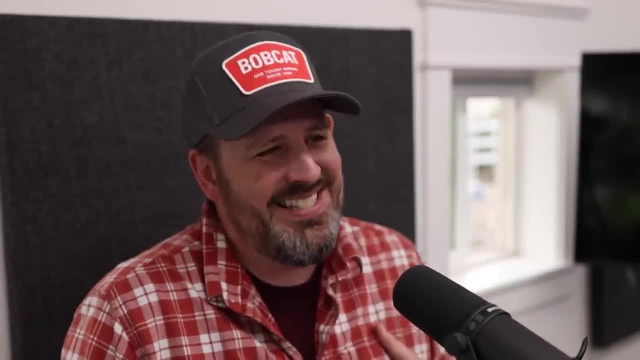 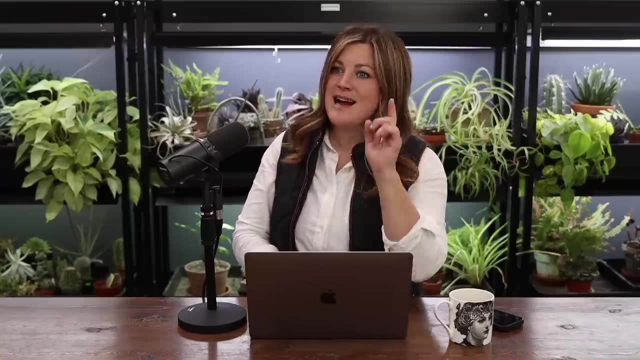 I don't know that the rest of us don't possess. I think that I think that you or I could stand back and be like OK, I'm scanning this bed, What does it need? And you would be able to say: I think we need an evergreen here, Yeah, Or I think we need something that's lower, right here. 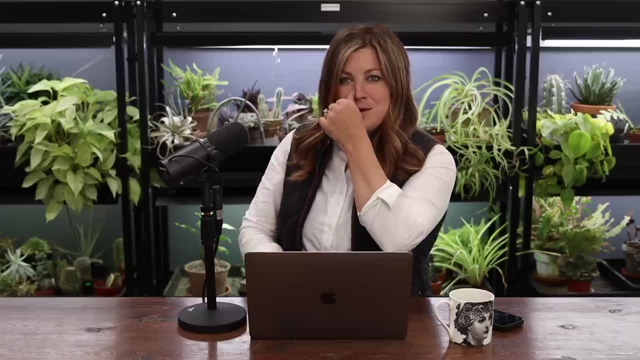 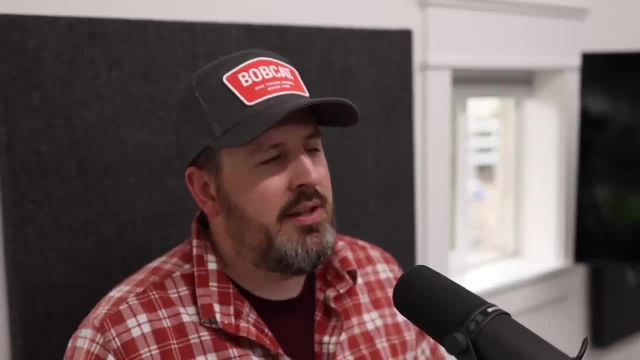 And then you just start looking for plants that meet those requirements. You know what I mean? I think most, I think most people could probably stand there and be like it's missing something. Yeah, If most people really think about it and they try not to put similar textures right next, 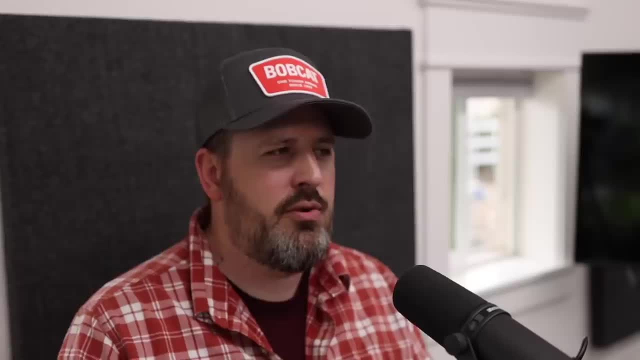 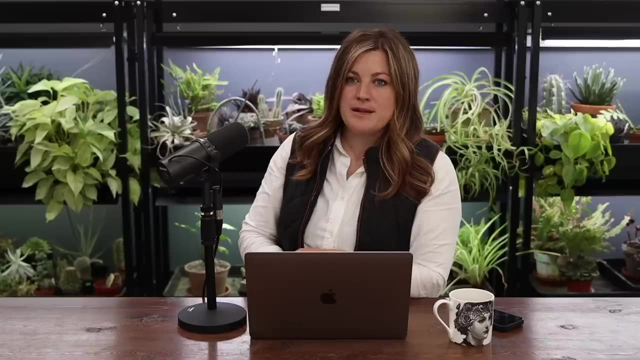 to each other, similar colors right next to each other, But also, I guess, understanding a little bit of color to where you're not putting like contrasting or like colors that will fight with each other. Yeah, Like pink and pink and red, or pink, soft pink and a hot orange. 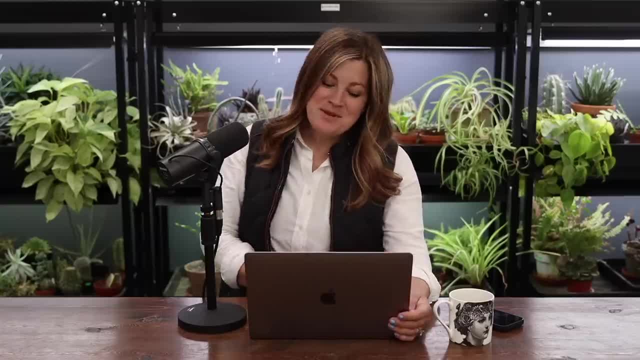 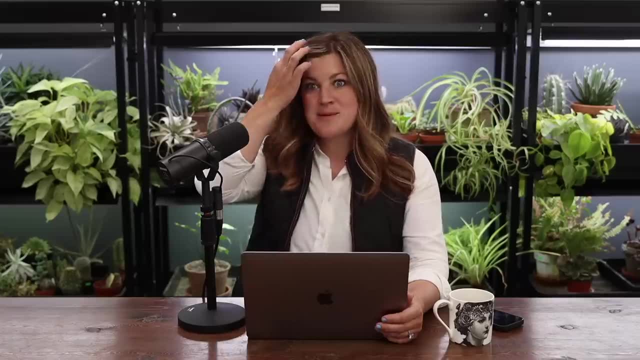 Yeah, I can't do that. Oh yeah, Landscape plans just don't do it for me. In fact, my mom and I were just talking about that today because we need to sit down and get serious about their landscape plan. My mom wants to kind of do that together And I told her: look, 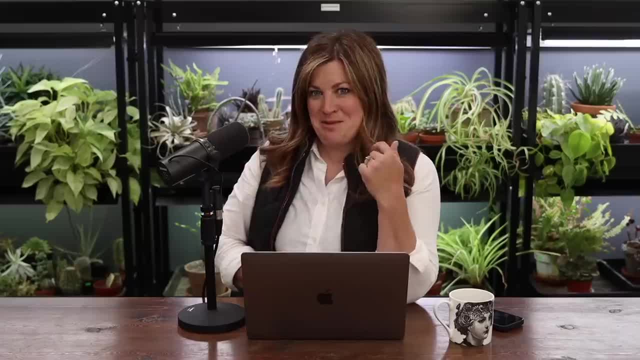 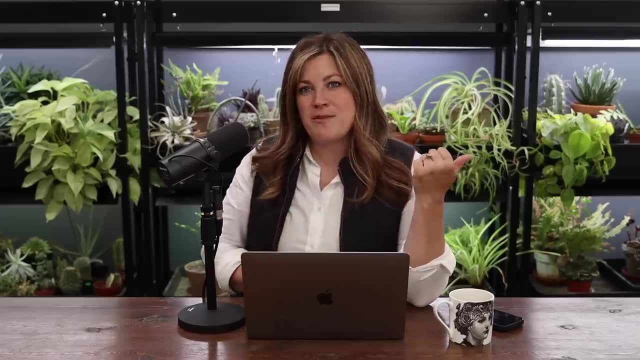 here's the deal: I'll help you with your landscape plan. You come over and help me with my front flower beds, And that way we can both bounce ideas off of each other, like set a day to do it, And I don't know. I feel like that front flower bed, though I think I know what I need to do. 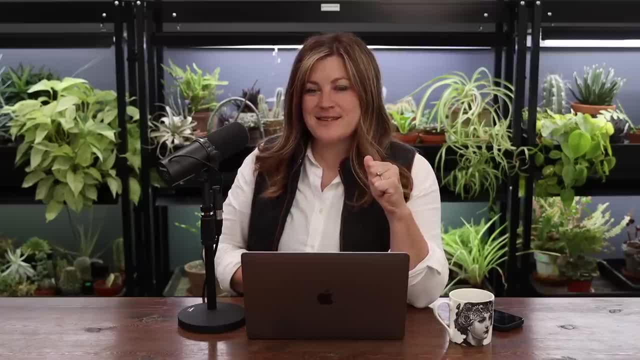 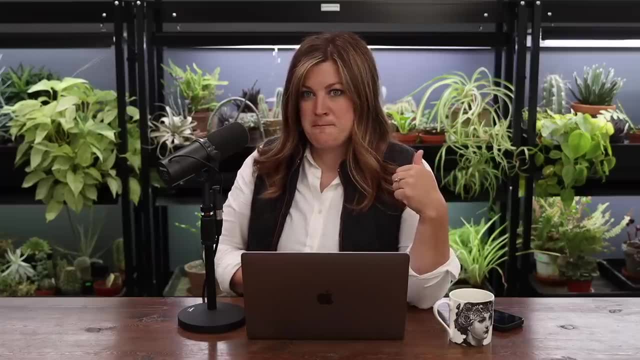 It's just a matter of like being brave enough to do it. Yeah, Because it's going to require pulling up a bunch of the lawn past the crab apple, possibly removing the crab apple because it's full of blight. Every year it's full of blight and we fight it. I don't even spray it. 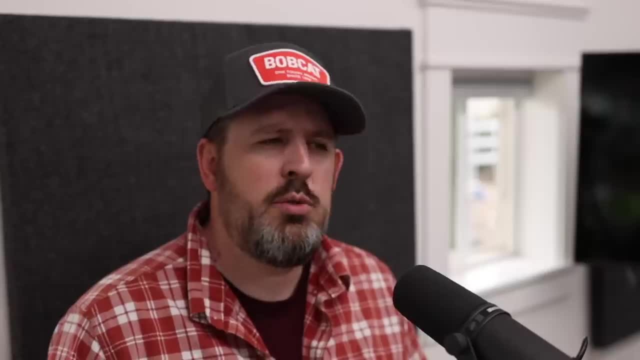 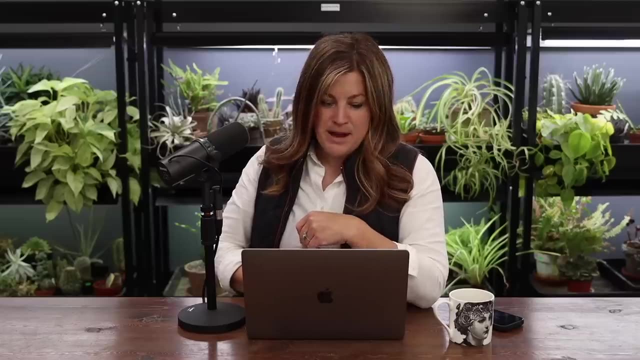 anymore because it never really works. Could we move it? Do you want to move it? I don't want to move a tree that deals with that. Yeah, that's true. I don't know. I feel like we could do something better up there. 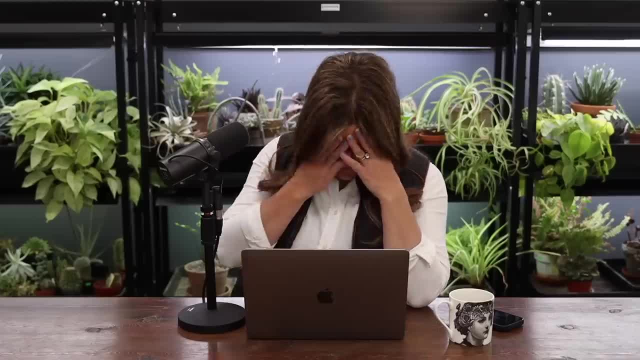 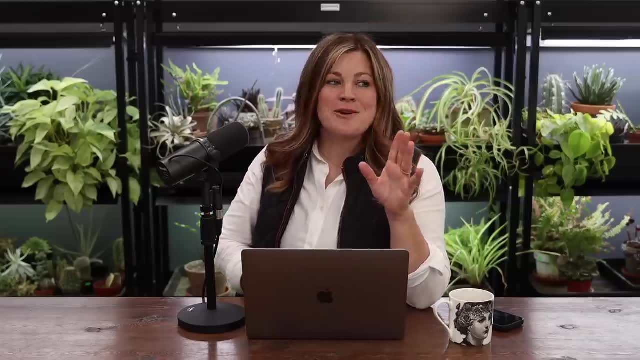 Well, we talked about putting a pond over there, but it'll get algae. You notice I haven't shown the pond for a little while. We're on Chris Schreiner's schedule. Oh, you called me today. I totally forgot to call him back. 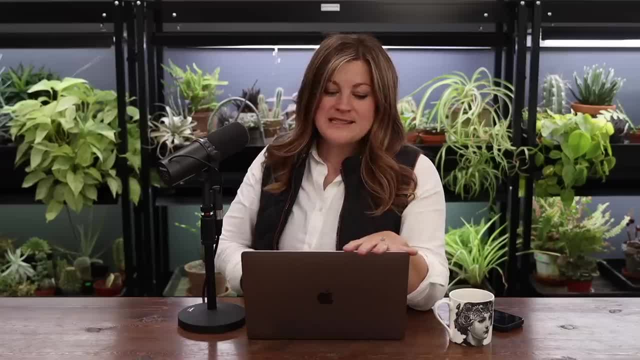 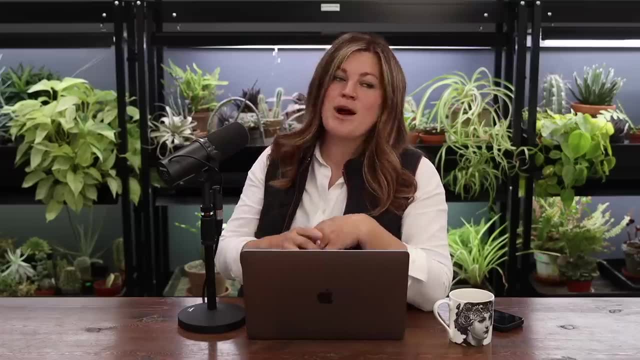 Oh, we're on a schedule for a big clean out. They said there would be a period of time where we were balancing the ecosystem and we would get algae. So they prepped us. We knew it was going to happen. I went and tried to get some algae out today. I actually got a lot of algae and it 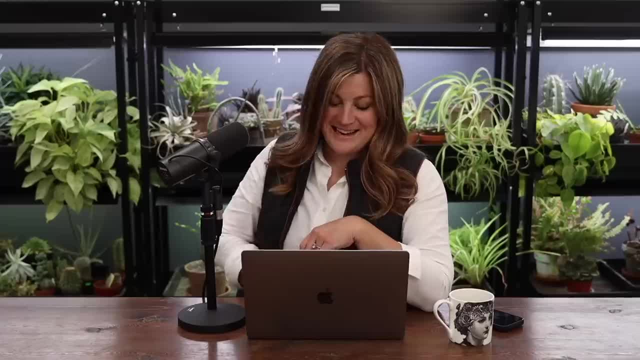 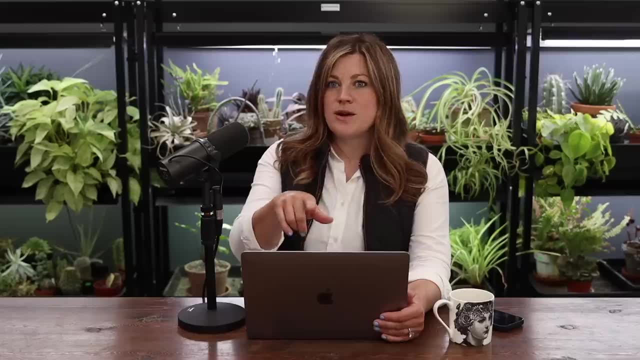 didn't seem to make an impact To dent. Yeah, You have to spend a lot of time getting it out right now. Growing Dreams, Homestead, said: love seeing you splitting plants to make them really stretch. Oh yeah, In that video with the ground covers there was a couple of them that were so rooted. 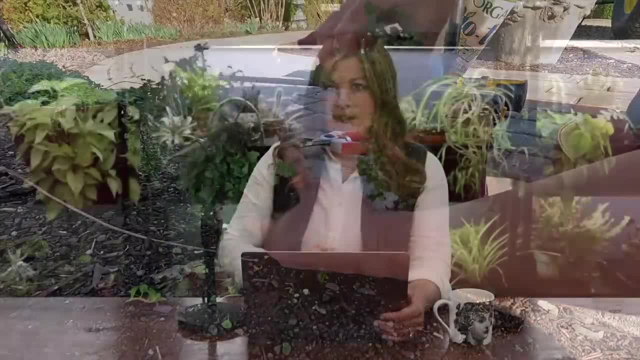 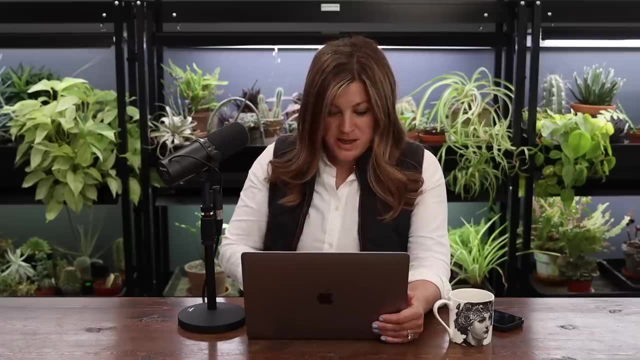 in all the way around the can that I felt like they were good to cut in half. Well, the one I cut in half, the star creeper, And then the Veronica I cut in quarters, which that made it stretch huge. What other plants can? 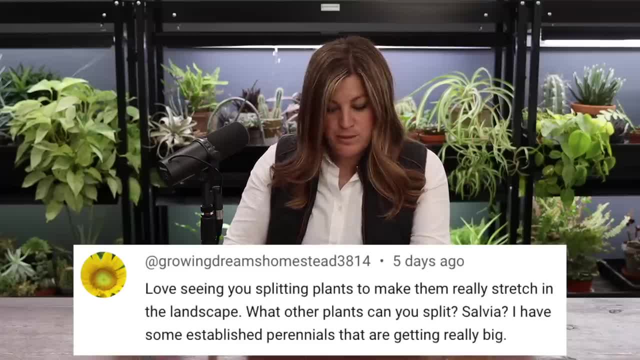 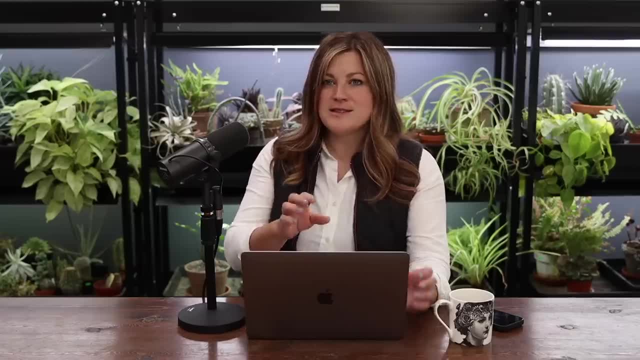 you split Salvia. Yes, I have some established perennials that are getting really big. Yeah, A lot of perennials benefit from being divided. A lot of times, like especially ornamental grasses, they'll start to just have like a ring around the outer part- that's nice, And then the center dies. 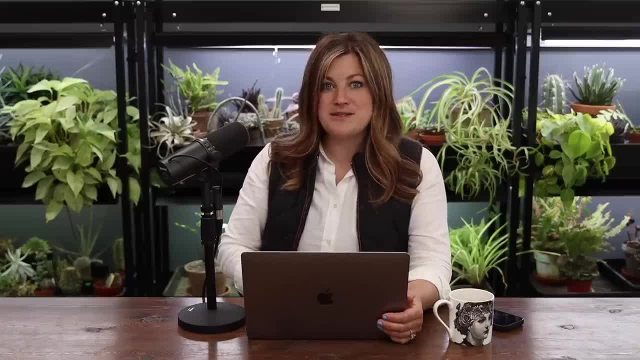 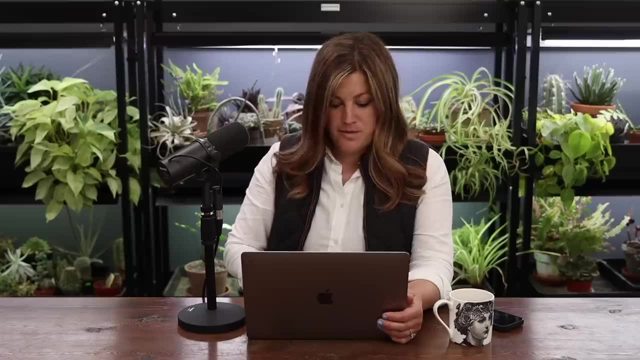 out or they'll flop over a lot easier because they just simply need to be divided. So a lot of those much more mature things- Yeah, definitely split them up and stretch them around your garden. Give them to friends. That's kind of fun. Rose Torn said how spaced. 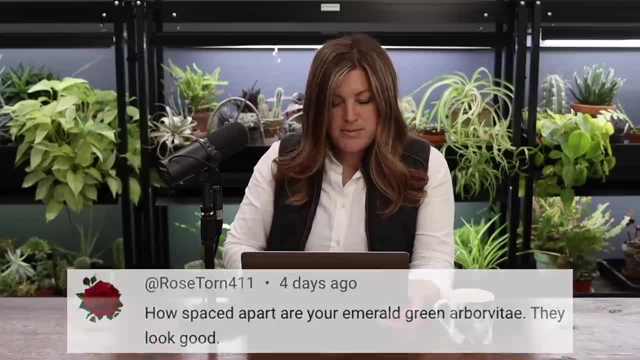 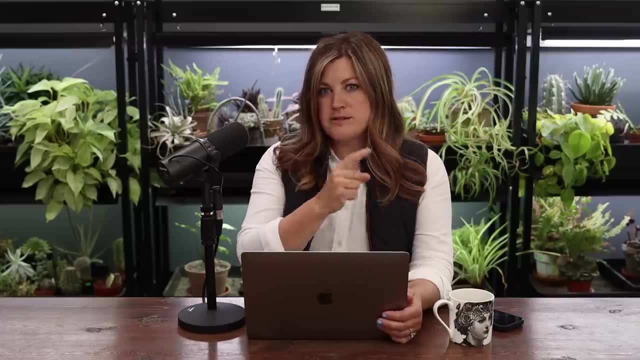 apart are your emerald green arborvitae. They look good. I think you are probably meaning the North Pole arborvitae- Very similar plant, but I don't know that we have any emerald greens. They're all North Poles along our fence lines. Yeah, I think we have all North Poles, Yeah, And 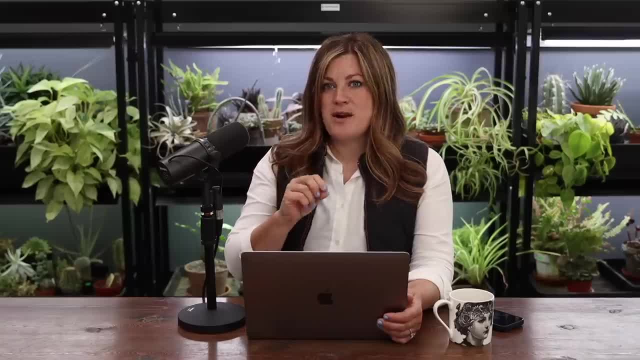 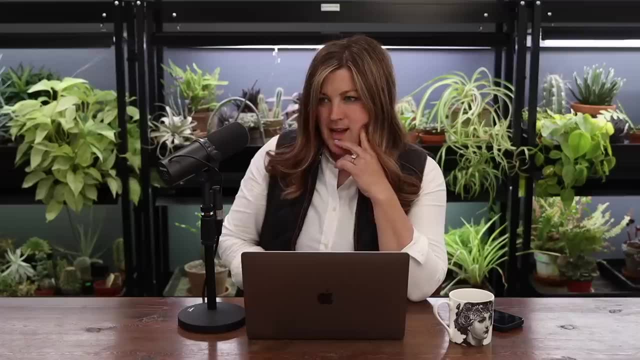 I think they were spaced about four feet from center. Whatever it was that we chose, I wish we would have gone a little bit closer together. Yeah, I think we were trying to take the average, because they say they grow three to five feet. Yeah, I think we were trying to take. 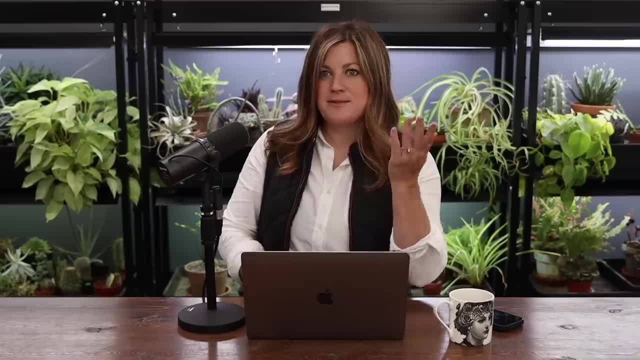 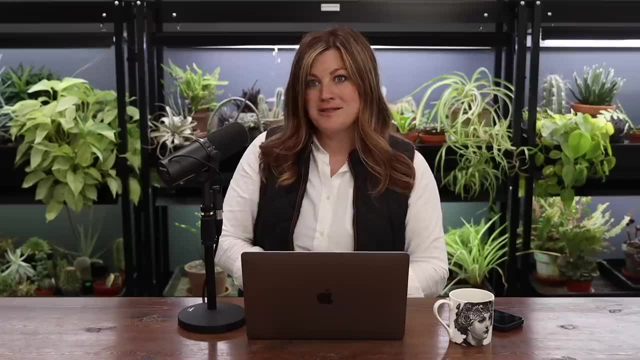 five feet wide, rather. So we thought, well, four feet, We'll go right in between. So they're not too close, but they're not too far, And you know they're creating a beautiful wall. I mean, if you. 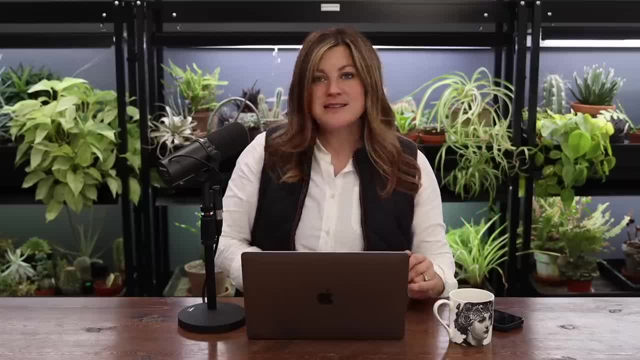 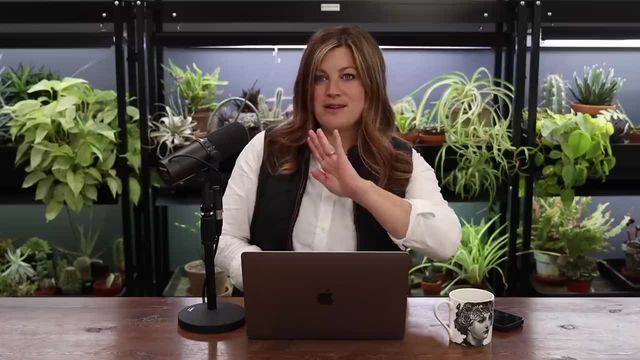 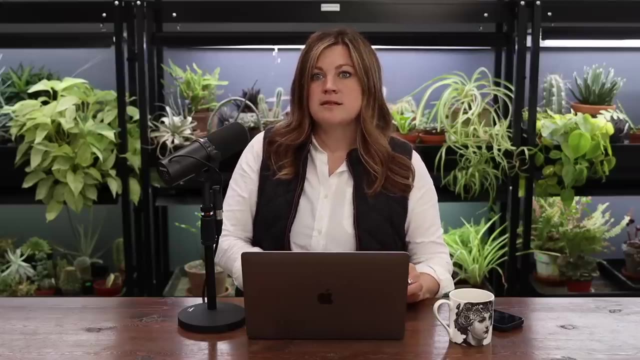 look at this row of arbs and that's kind of been your baby, I mean. you kept them looking really nice. I looked down that and I just this is exactly what we wanted. We wanted this beautiful green wall, and that's what they do, Maybe just a little bit taller. Well, yeah, Yeah, But they'll. 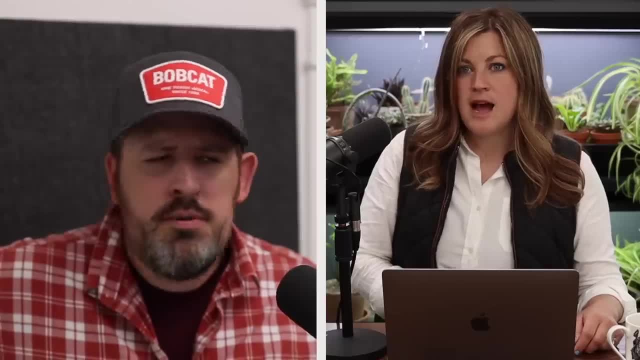 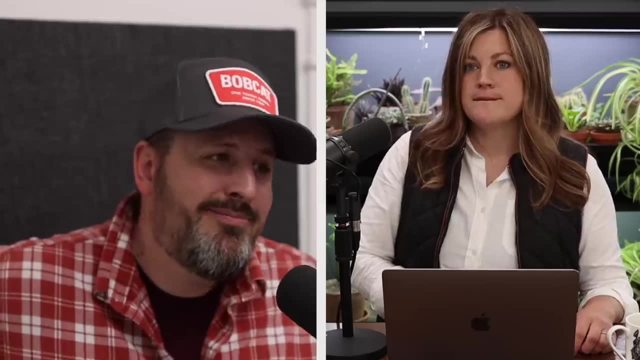 get there. Yeah, I mean, what are they right now? Eight, No, they're probably closer to 10.. Are you think so? Yeah, So we'll probably just get a few more feet, Another few feet. It's like 12 to 15, right? Yeah, So 10 to 15, I think I always think, I always assume it's just. 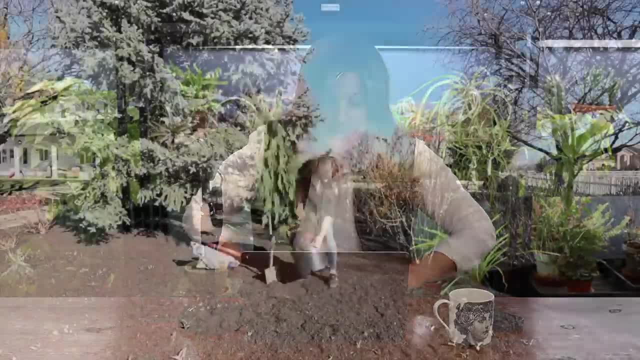 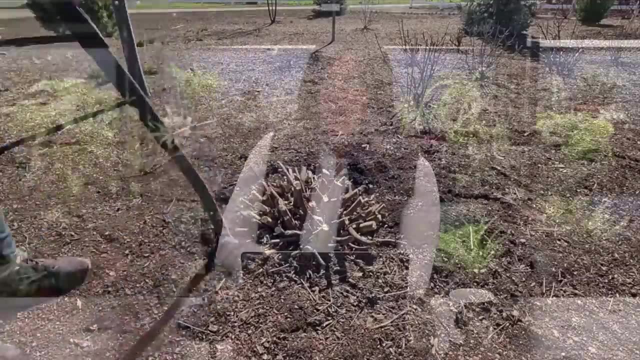 a little bit more. Yeah, Maybe we'll see. Our next video was planting a weeping Alaskan cedar, sedum and hydrangeas, plus transplanting a massive mature hibiscus. That root ball was a beast I had. 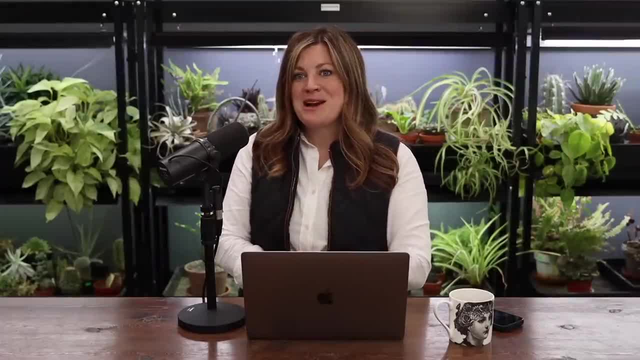 I got it out of the hole, but barely. You were like: do you want me to come get it Because you were standing there next to me when I was digging. I was like, no, I'm going to get this thing out of. 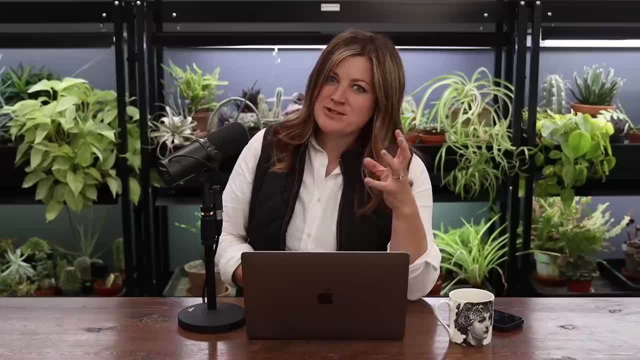 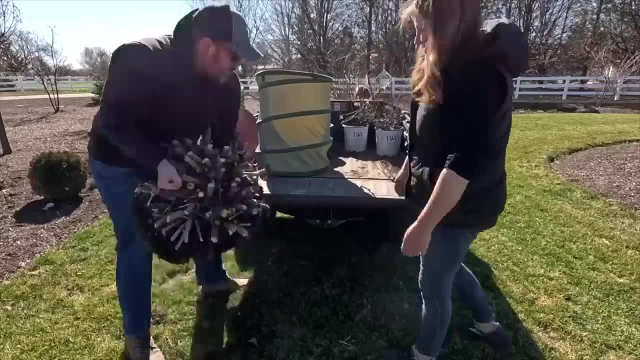 the hole, but I got it taken over to the gator. You know when you get into a project and you just like, do not want to admit defeat. That's where I was at, Cause I was kind of mad at the root ball being so heavy, but I couldn't get it up into the gator, So Aaron had to lift it up. into the gator and back down in the dirt lands when we got that, all that, it's whoops, it's spot, all prepped. Uh, but the weeping Alaskan cedar, the variety is Jubilee. It stays a little bit more. 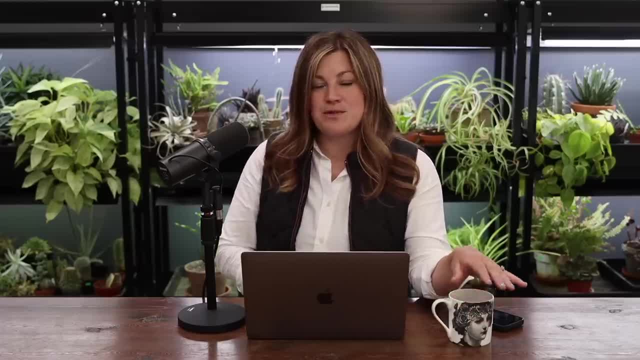 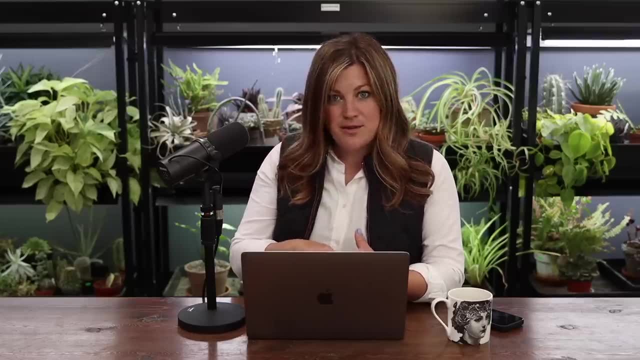 narrow than the traditional weeping Alaskan, And I just think they're all so beautiful, So architectural and graceful looking. We planted the lemon jade sedum near some reminiscent pink roses out in the South garden, And then the hydrangeas were the little, not little lime, They were the lime light. 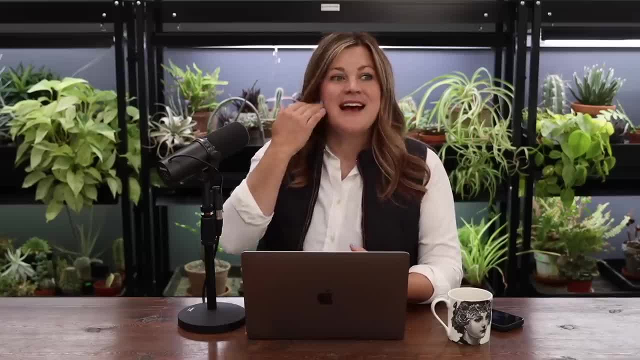 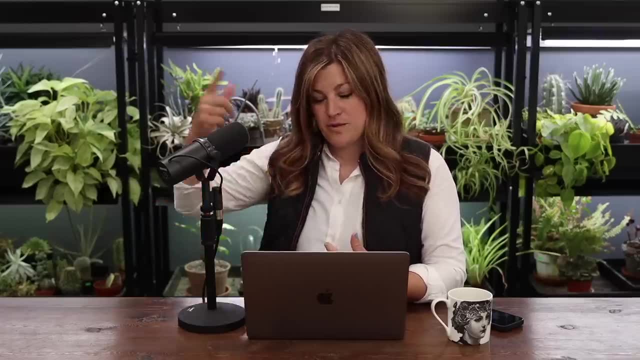 primes- I hate those names kind of jumbled up. Anyway, when we took the hibiscus out it opened up room for two more hydrangeas on the far end And then one to fill in a gap toward the other side. So Anna said, if I remember correctly, you have a weeping cedar planted close to your house. 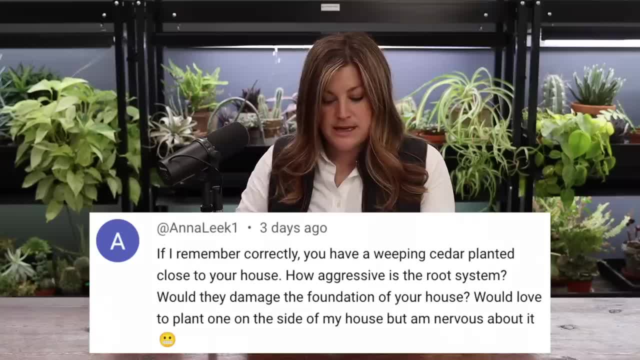 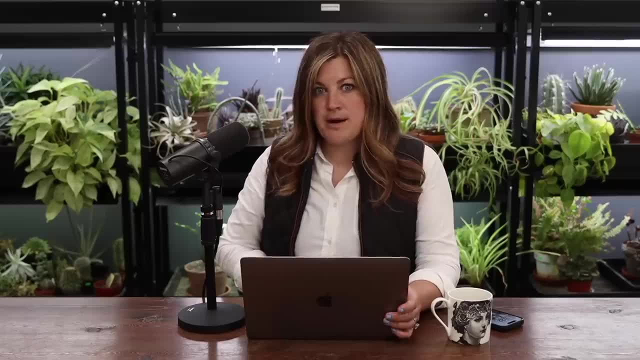 How aggressive is the root system? Would they damage the foundation of your house? You know, we have a weeping white spruce, which is a little bit different, The weeping Alaskan. I probably would not put right up next to my house because they'll typically get um, like what, 25 by 12, was this one? the traditional ones get 25 by 15.. That's a pretty sizable. I mean, if it was like 10,, 15 feet away from the house, which is not that far, I would say I wouldn't be worried about it. but I would not. 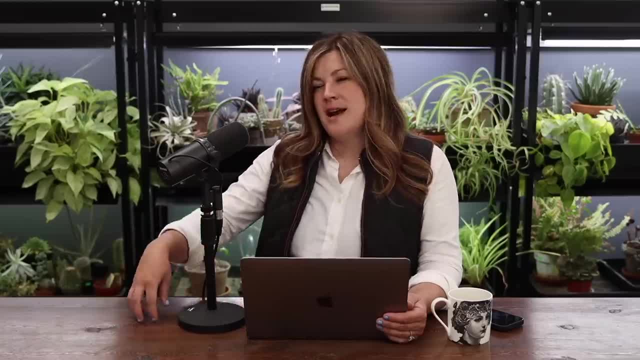 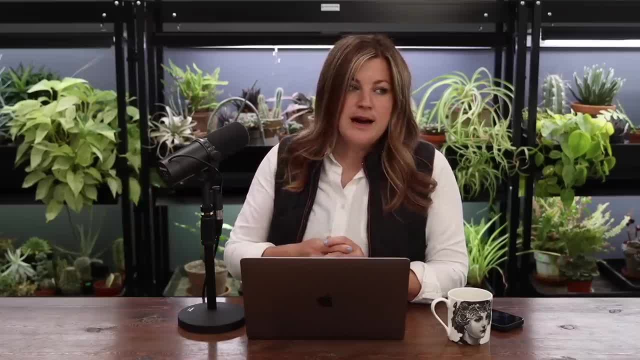 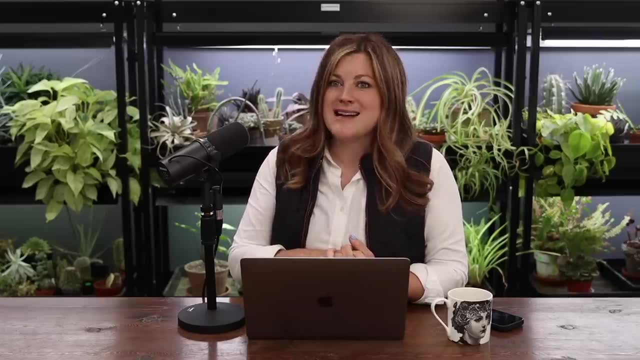 four feet wide, So it stays a lot smaller. Um, so it's just naturally not going to have as big of a root system And it depends, like on the culture of the plant, Like it depends on where it's at. Um, some will get upwards of 15.. Some will stay closer to the 10 foot. The leader of. 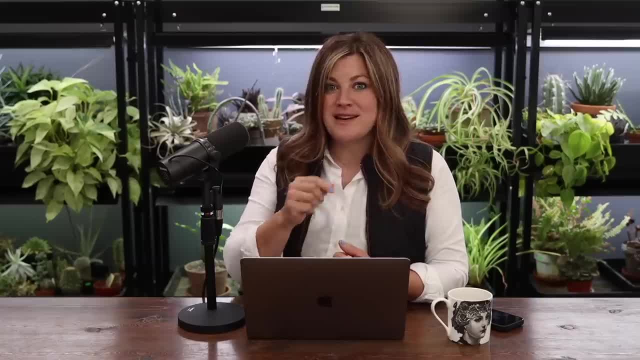 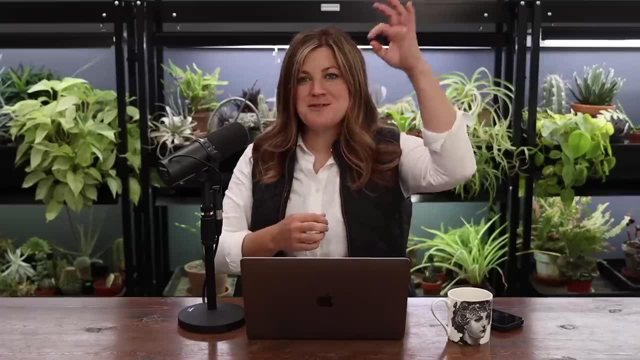 ours broke out not this winter but last winter, because we don't have any gutters on that side of the house. I don't know why There's not that much watershed on that side of the house. It was just enough. I think it was just enough to drip on the top, right on the top of that plant. 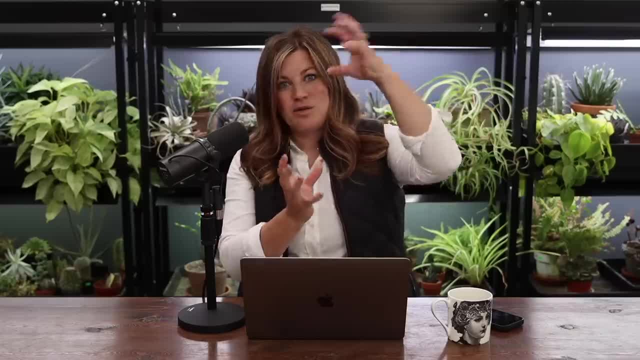 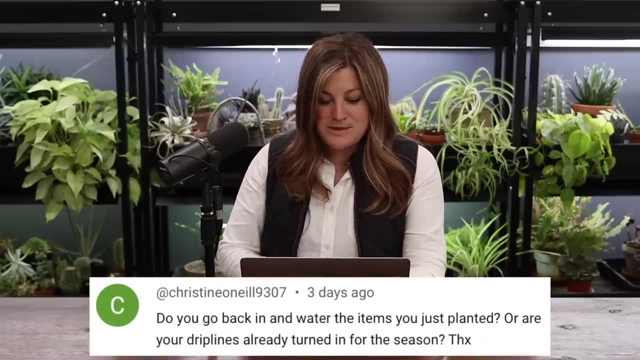 And it formed a big chunk of ice and the whole thing just like tipped and cracked. That's the leader. I know the rest of the plant looks okay, though Christine said: do you go back in and water the items you just planted or your drip lines already turned in for the season? Our drip? 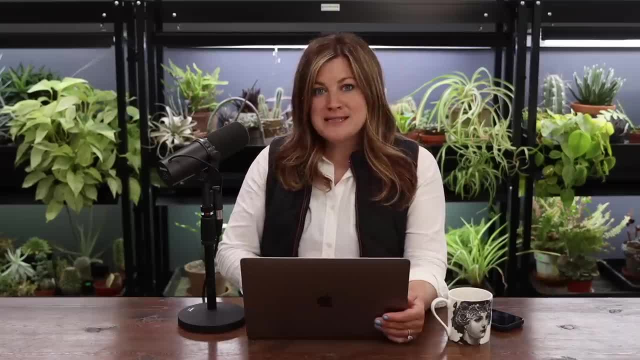 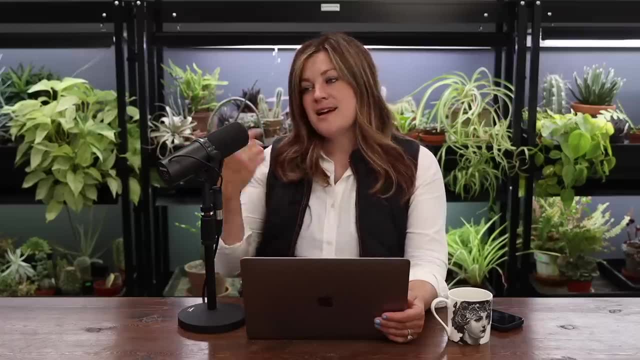 lines are not on yet. Um, and I do go around and water them, but at this point when we don't have our water on, I have to go find a frost free faucet, which is oftentimes not nearby the plants, And I have to lug watering cans and buckets around. It's just kind of a more labor intensive. 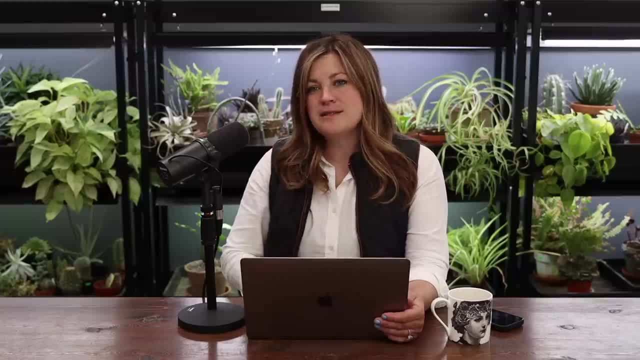 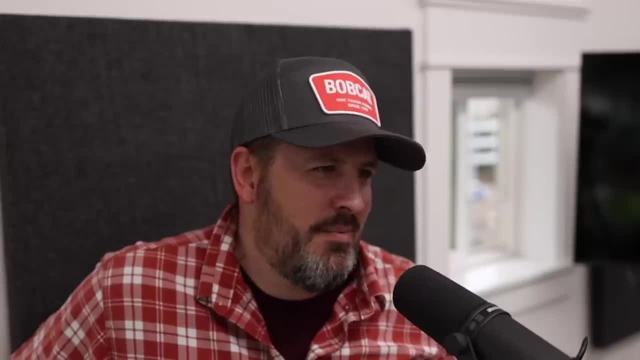 tedious job, So I usually leave that out. Maybe I should leave it in sometime because I do, And maybe I'll just mention that we'll go back through and water everything That time. I think we went around in the evening. I think that was yesterday. Yeah, Yesterday we went around and watered stuff. 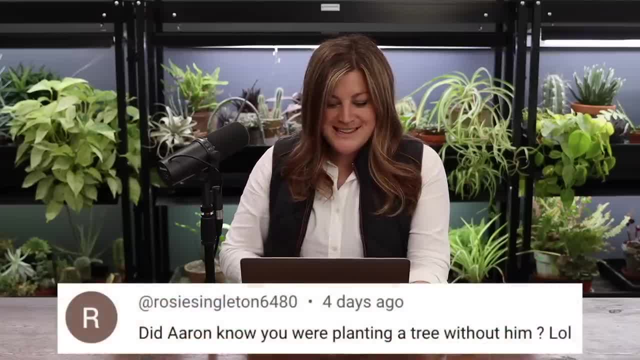 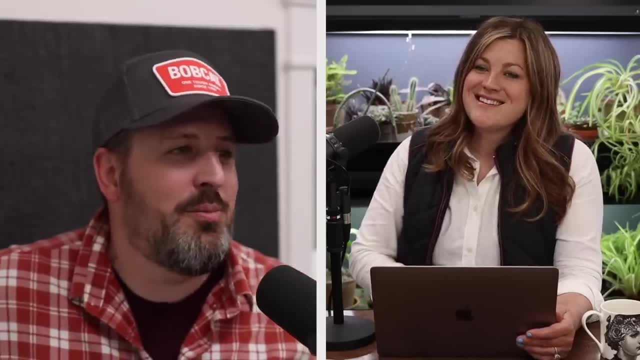 that I planted earlier. Uh, Rosie said: did Aaron know you were planting a tree without him planting the tree? Oh, the waving Alaskan cedar. You didn't. You told me, you showed me afterward. You were all proud of yourself. I know I love that tree. 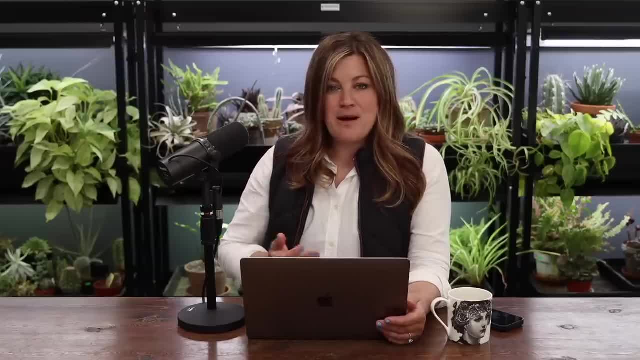 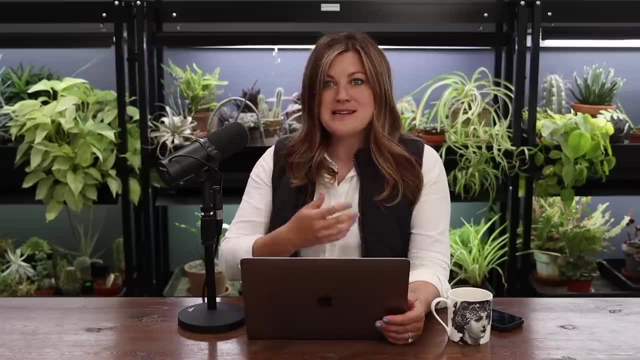 No, Most of the time when I'm planting like that, I'm filming myself. So I'm out out there all by myself and just moving the camera around and and such So oftentimes you don't even know where things are, what I'm going to be planting or anything I'm doing that day, And so in the 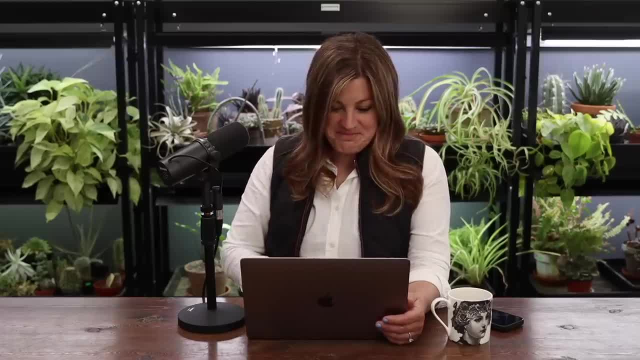 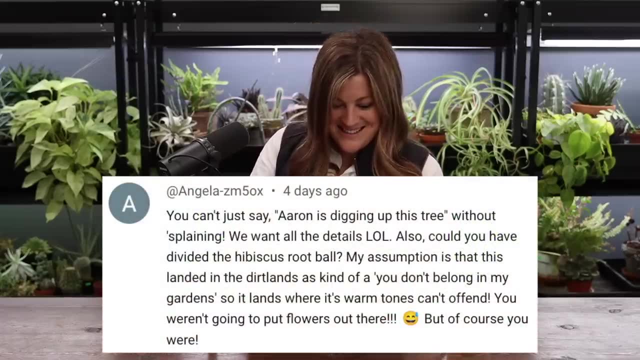 evening we go around and I'll show them the things that I just planted. Angela said you can't just say Aaron is digging up this tree without explaining. We all want, we want all the details. Also, could you have divided that hibiscus root ball? I'm sure we could have. 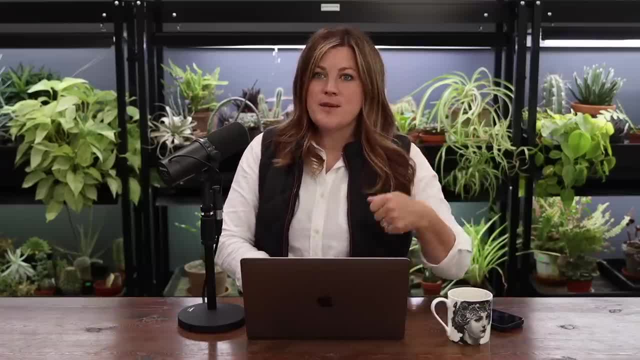 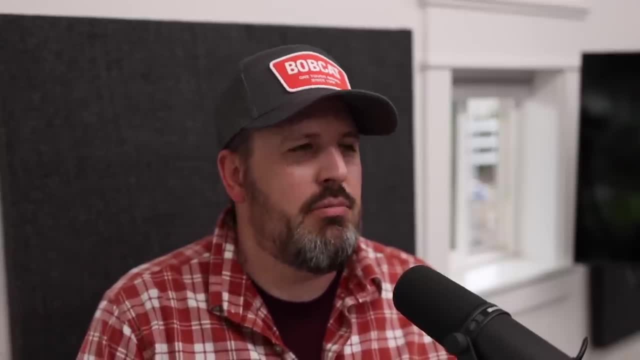 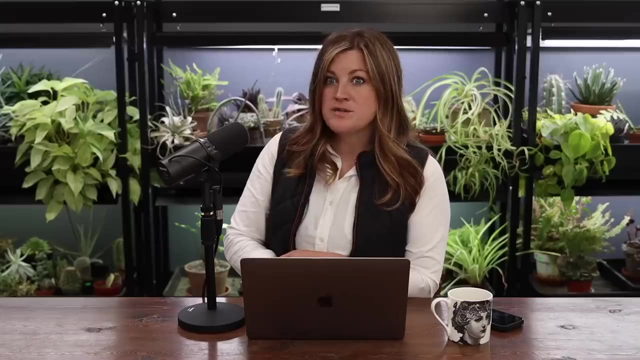 The tree. Oh, you were clawing away at the soil around the base of that Linden tree. Yeah, I think we got a little bit too much. We either planted it too deep or we, like some mulch, got over the top of, like close to the trunk, Yeah. So I was trying to move it away And you did a bunch of them. 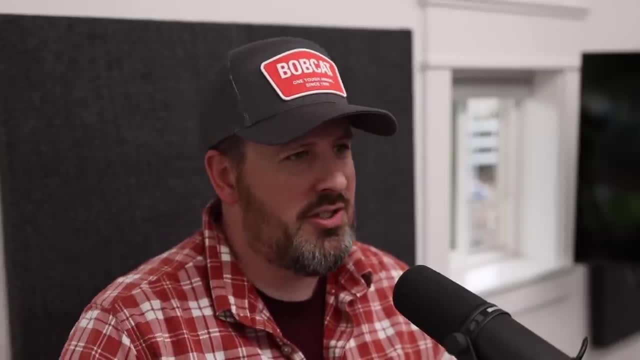 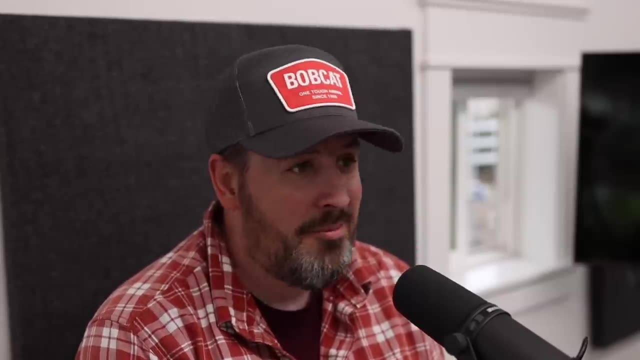 Yeah, All the trees out there in the South garden. I was just. I used a little cultivator, I was just trying to get the kind of soil away. So anyway, we probably see that's why you got to plant Plant them high. Well, it's kind of true If you plant it right at soil level, pre-mulch. 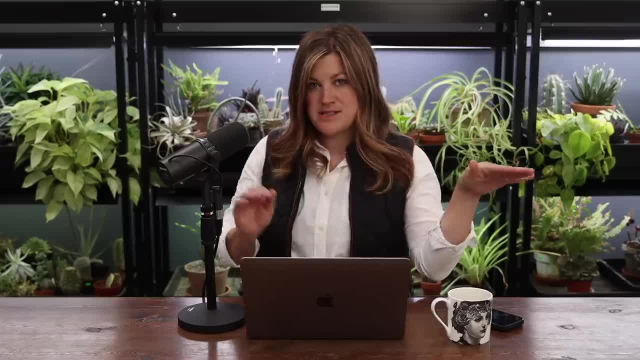 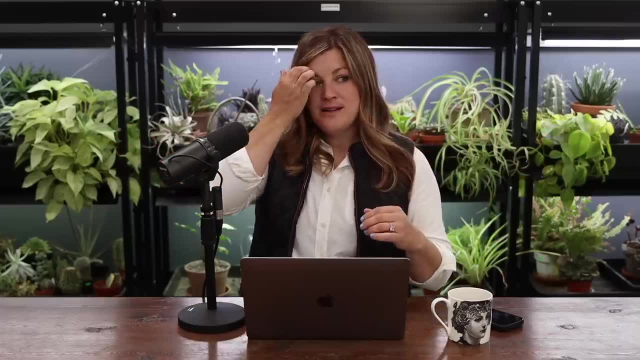 then you have to be very careful about like you can put a skiff over the top just to blend it in, but then it gets washed away a lot easier when you're planting your root ball up high and then mulching up. you know to that level, then you know you're not. I was telling you that I was. 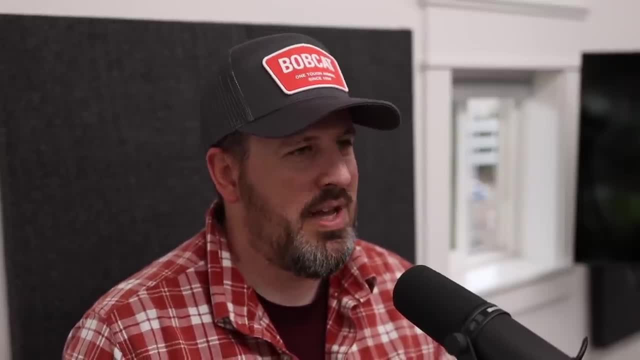 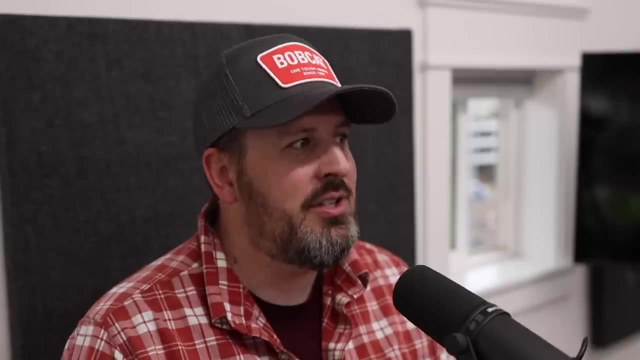 like I feel like a lot of people really misunderstand when I say: planted high, because I am planting high, but I'm also counting on that layer. I'm counting on bringing in a couple inches of mulch, And when you bring the mulch in all of a sudden it's not. 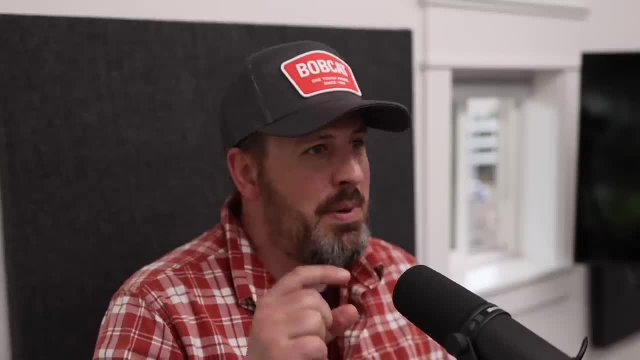 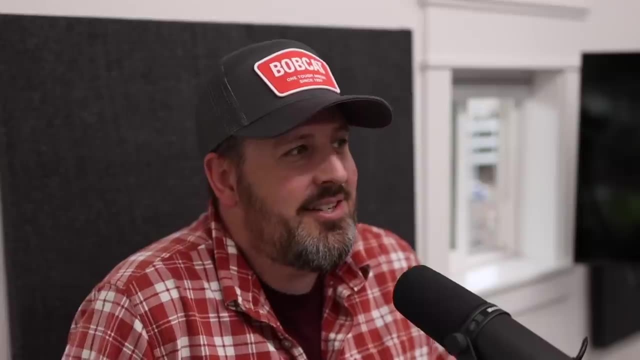 it's not high anymore, Right? I mean, it's like it might be barely above, you know, like a half an inch above soil level after the mulch is brought in. So yeah, it's like cause, if you plant at soil level and then bring mulch in, well then you just plant it in a 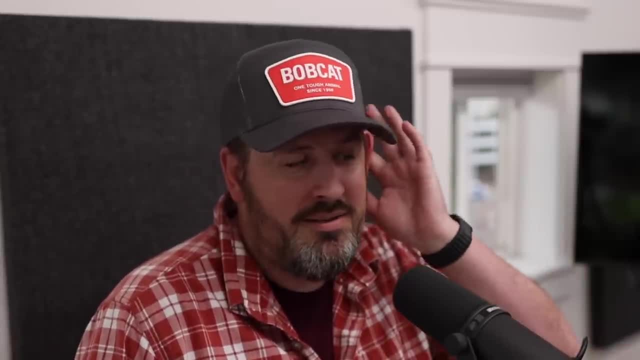 concave. And if that's what you want, great. It's not what I want, Yeah, And not usually that great for the trees. Yorkie said: love the weeping cedar, but the boxwood hedge looks so out of place stopping in the middle of the bed. 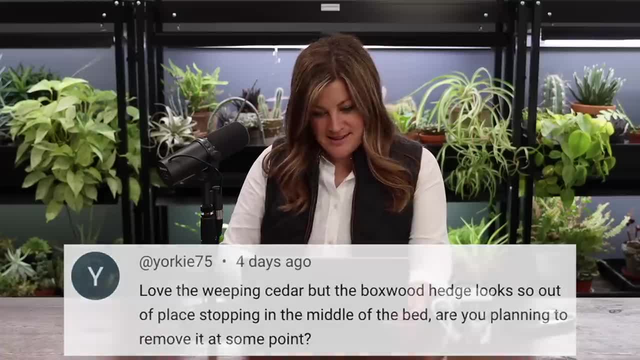 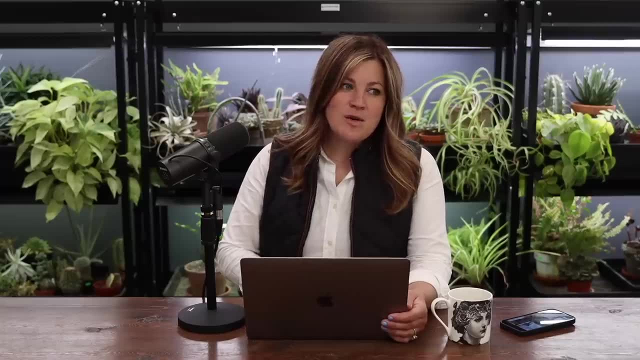 I do agree with that. Are you planning to remove it at some point? Yes, Yes, we are, And I don't know what's stopping me at this point doing that. I could probably do that because the overall shape of that bed isn't going to change when we- you know, when we do. 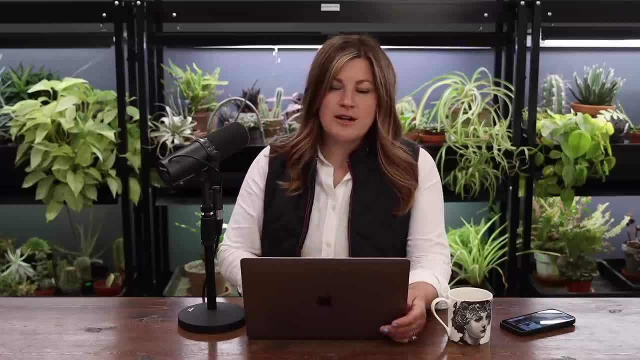 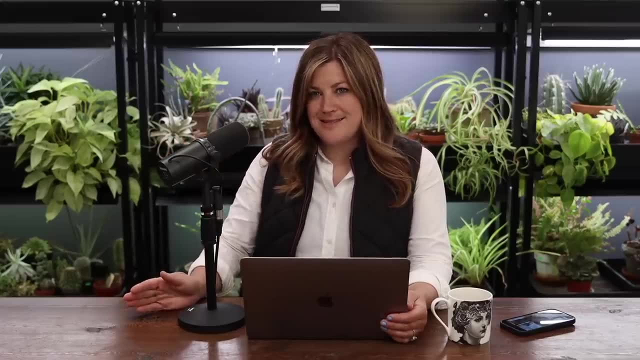 overhaul sort of the Persephone garden area, Um, but at some point we do plan on removing that little picket fence in front of that garden. Maybe I don't know. I like it there, The picket, Really, Oh wow. 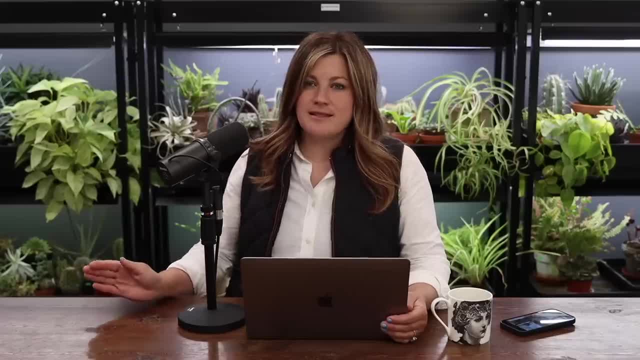 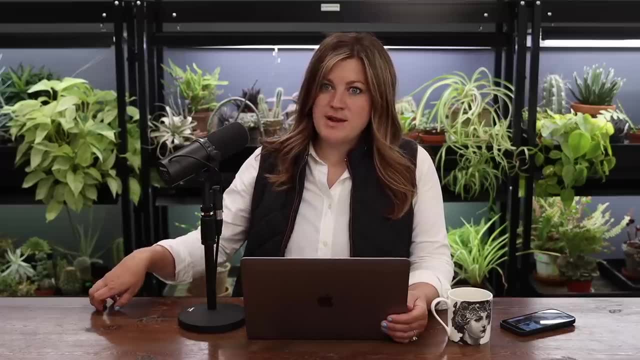 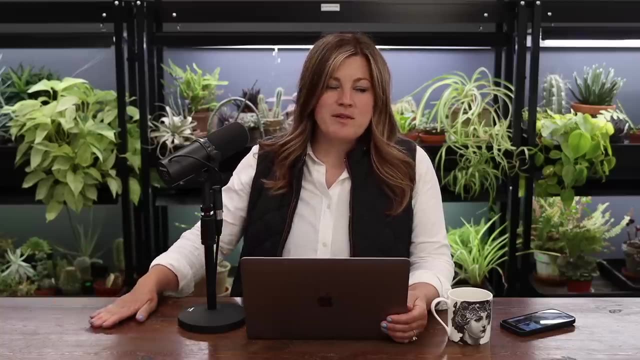 I like that it differentiates it between like garden and driveway. But Paul and Aaron did get out into the new lawn area you know just beyond there And they mapped out where the paddocks are going to be and where the barn is going to be sometime down the road. But I feel like when we 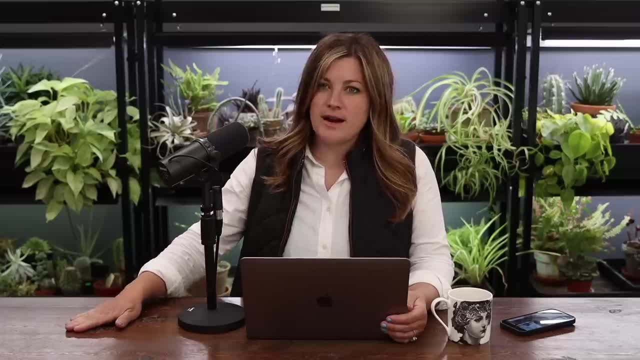 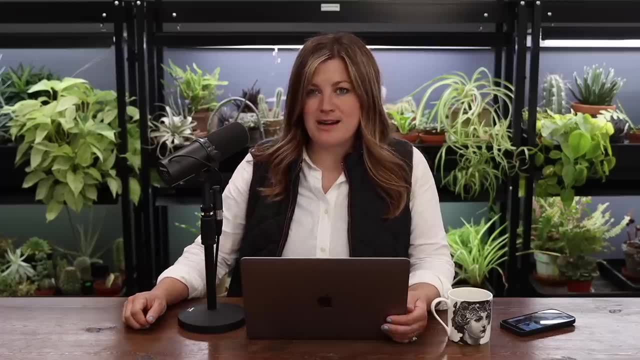 start planting that area up and tearing things out over there. um, I feel like that's when that area will change. I don't know. I don't know. It's making me hold on, I think. I think I just grasp onto certain things that, like the boxwoods, are largely healthy, And so I don't know most of. 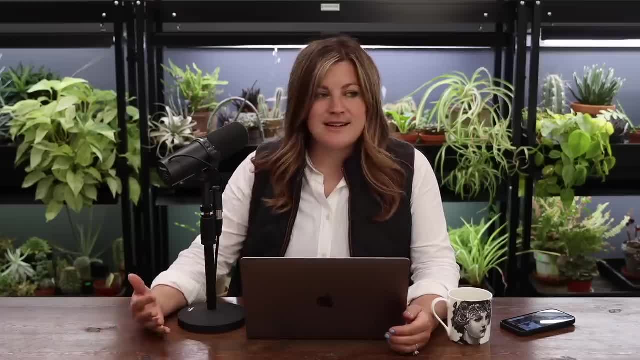 the time when we get rid of something, I'm like, okay, that's good, I'm glad we did that And you know voice of reason back back over there. I mean, I think you know Paul and I could rip. 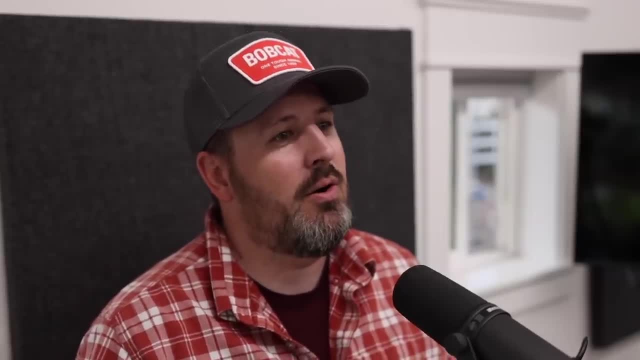 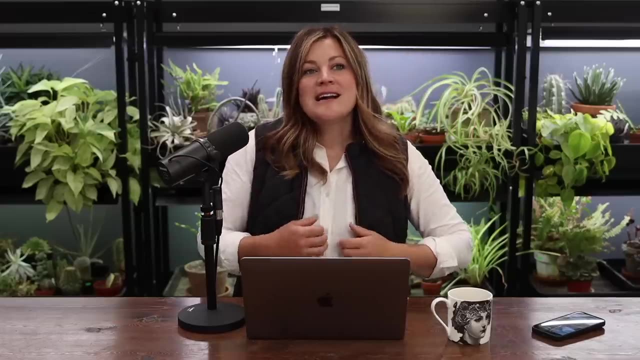 those boxwoods out and just mulch it And you'd be like, oh, that's what that space needed, And you're probably right. You're probably right, I don't know. I just I get to a point where I do start getting overwhelmed when, um, there are too many irons. 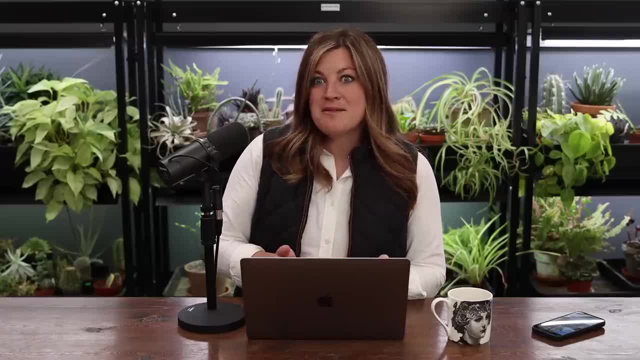 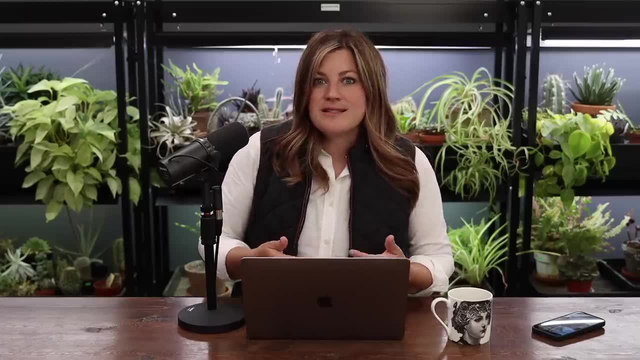 in the fire. I feel like I just need a year where things aren't ripped out. I just need a year to go in and plant things and fill in the holes that we currently have, And I actually have the, the brain space and the energy to do that. But when we've got things just like going 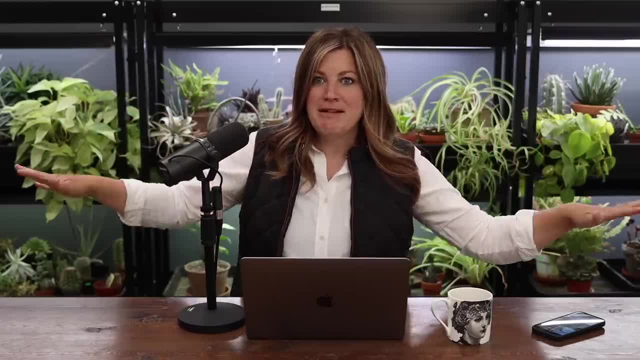 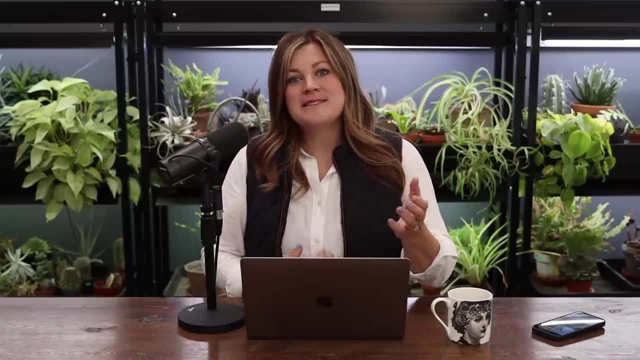 you know, tearing out here and there and everywhere. I just feel like everything's just and then I feel like I can't, I can't grasp any idea in my in my head, I don't know. So hence the random boxwood hedge will probably stay for a little while. Cassandra said. 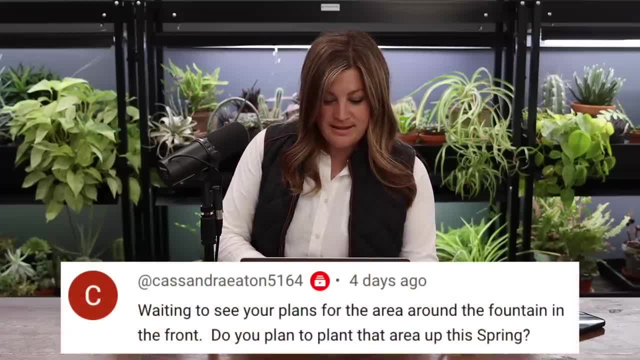 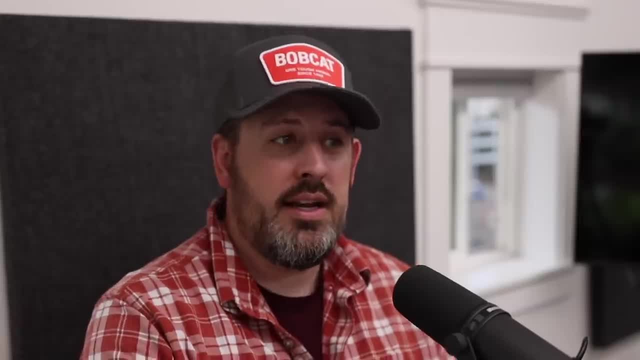 waiting to see your plans for the area around the fountain in the front. Do you plan to plant that area up this spring? We are going to tackle that area this year. See, that's one of the things. like we are going to get a concrete under there. I, the guy uh, got the bid. I said yes, let's do this thing. 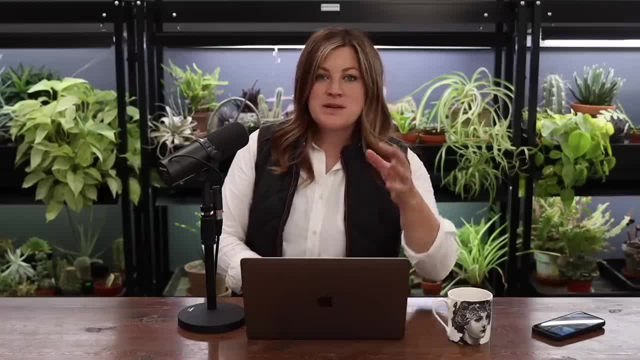 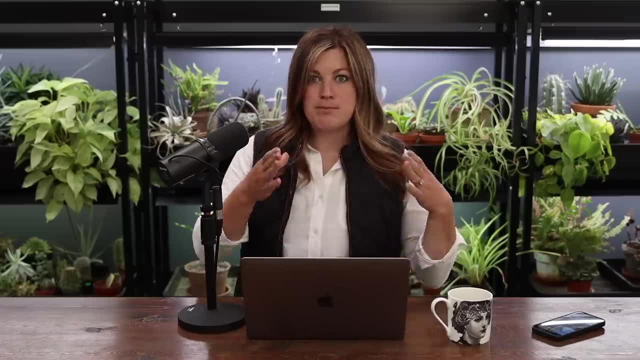 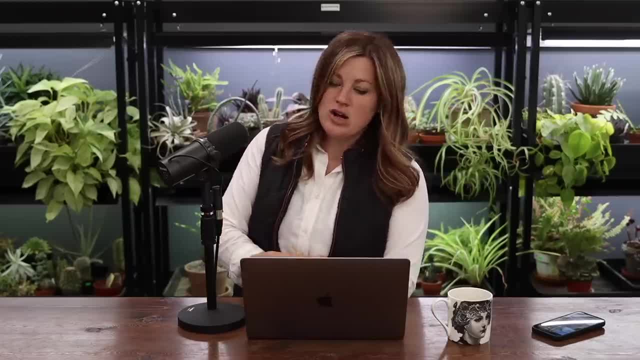 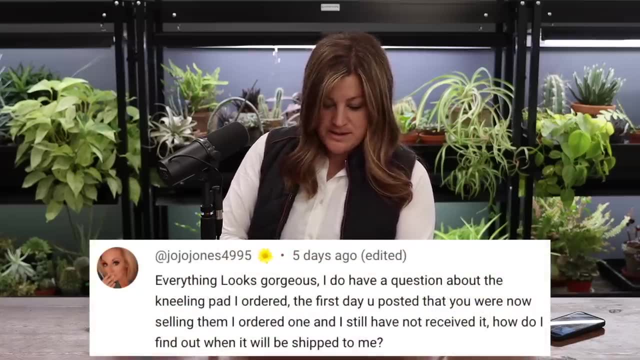 And like: tidy and set up nicely. Yeah, It can't sink at all That sort of thing. Jojo Jones said: everything looks gorgeous. Thank you. I do have a question about the kneeling pad. I ordered the first day you posted that you were now selling them. I ordered one. I still have not received. 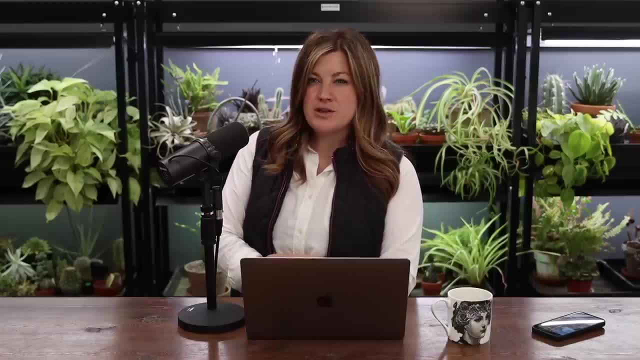 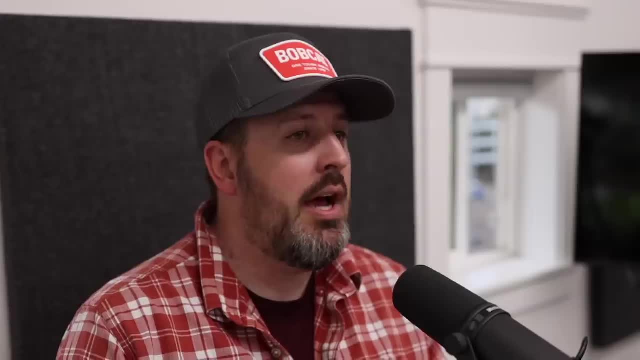 it because they were on pre-order. We actually do not have them yet. They should be here like soon, soon, Uh, but they are. they were just pre-orders. Um, so sorry. I mean I know a couple people like did misunderstand the emailed and we just gave them a full refund, If you know. 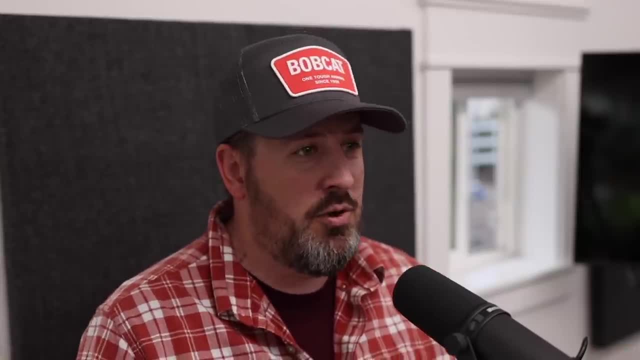 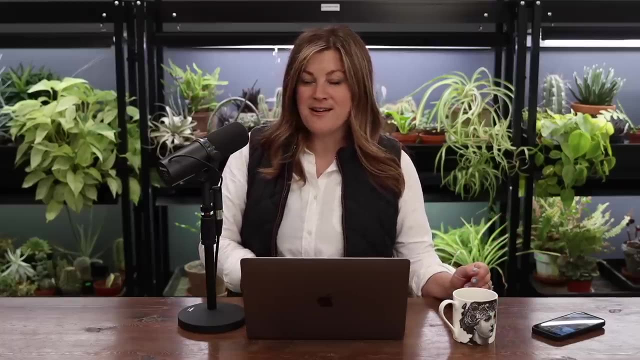 there was some misunderstanding. So, if that's the case, just shoot us an email If you do want to refund or if you want to wait, you know. but they are awesome though, You guys. I've been using them now for this whole growing season so far And I just I think you guys are going to love. 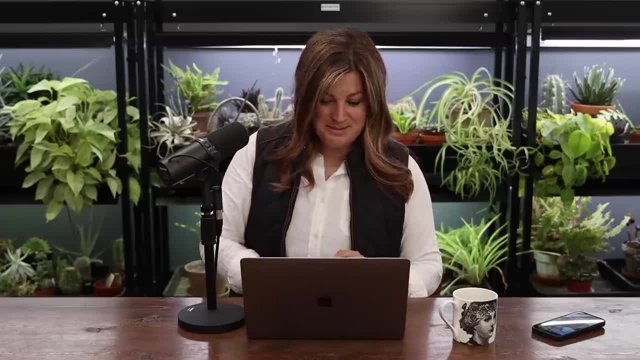 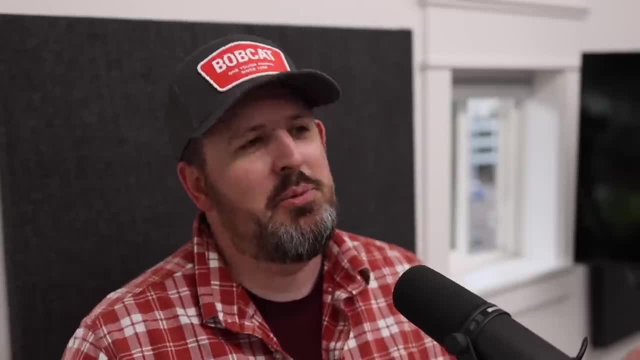 them. So thank you to everybody who has ordered one. And yeah, we have more coming, A lot more coming. I don't think we're going to do the pre-order thing again. Uh, it was. it was a little bit of a nightmare, to be honest, Cause I think, um, I think a lot of people just order. 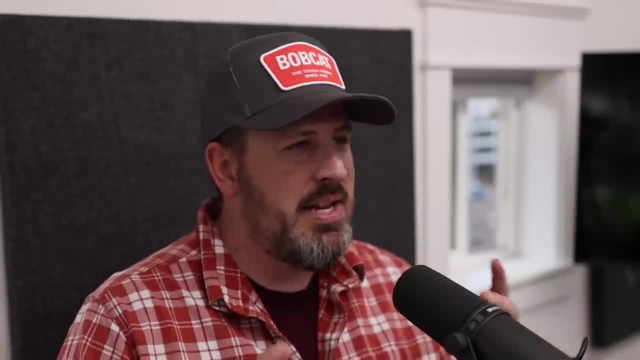 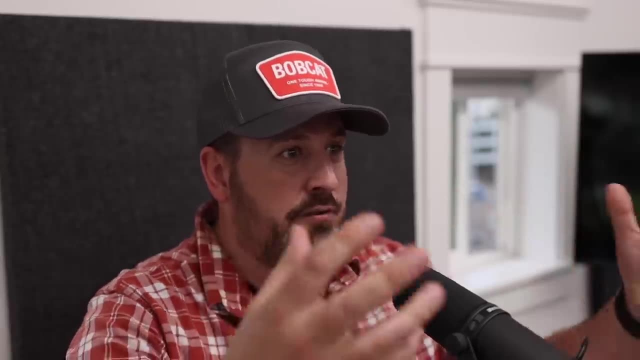 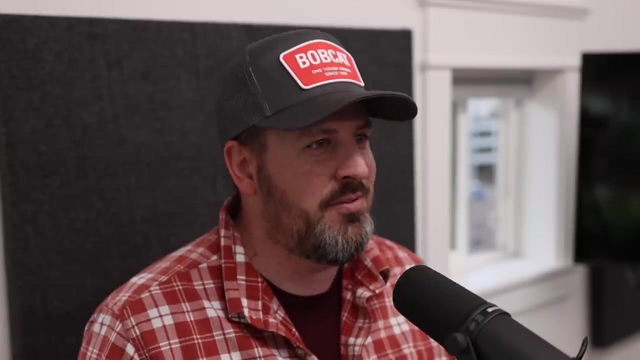 quickly and you can say it's a pre-order. You can write it in as many places as you think. Yeah, Um, aside from like we, we didn't have like a flashing screen that was like: before you order this, it is a pre-order, you know, And so it. it created like tons of customer service emails and 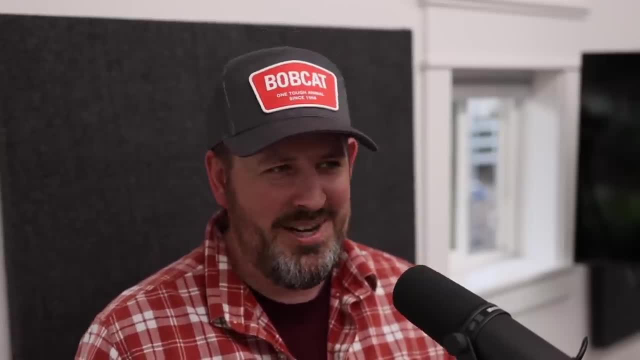 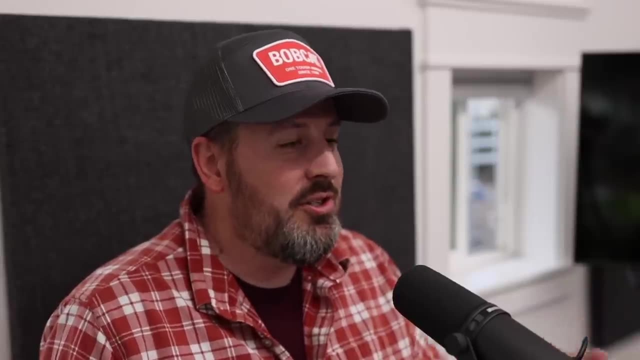 calls and stuff. I think, because of that, we'll just wait till we. because of that, we have a new customer service representative starting next Monday. Yeah Well, actually. um, so the store, and then, by like the end of like, in two weeks, there'll be four full-time people. 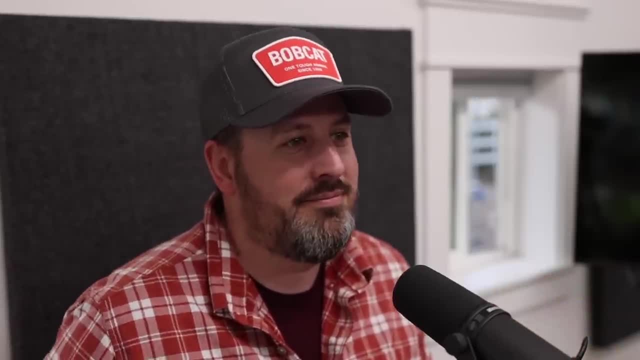 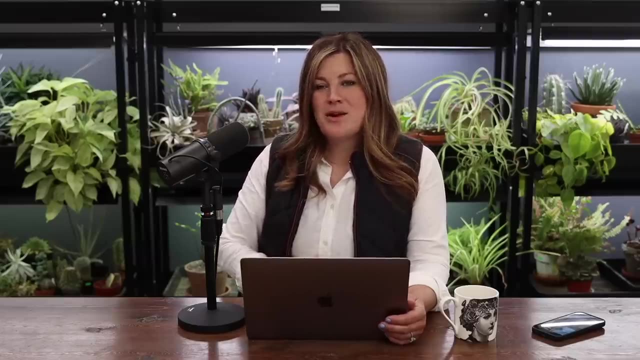 working on the store stuff. It's like it's growing, Which is amazing. You guys are so awesome. Thank you for the support, for sure. I'm really sorry, though, about that. you know, I feel bad because I feel I feel like I've done that before. You know, sometimes you just get. 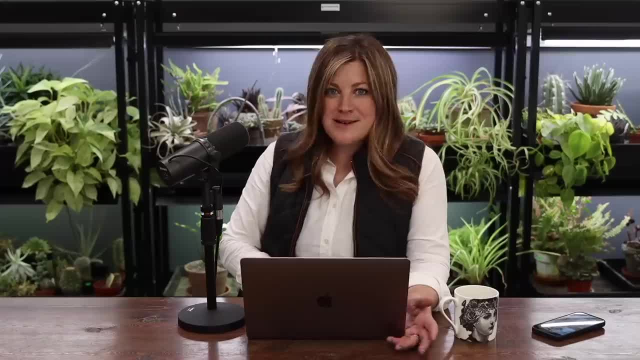 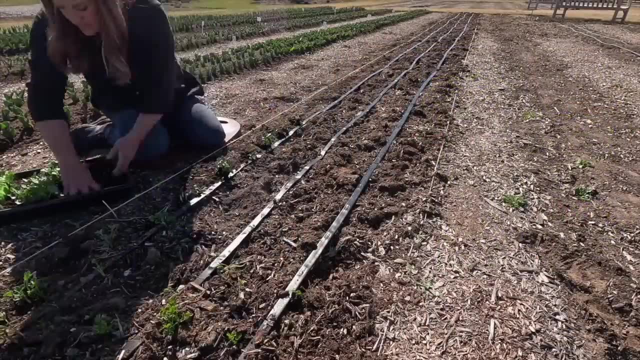 excited and you want to, you know, be supportive, which was so awesome of you, Um, and it's. it's easy to miss details like that. Next video is planting Ranunculus and setting up the best low, like low- caterpillar tunnel that I've ever set up before- Not that I've set up a. 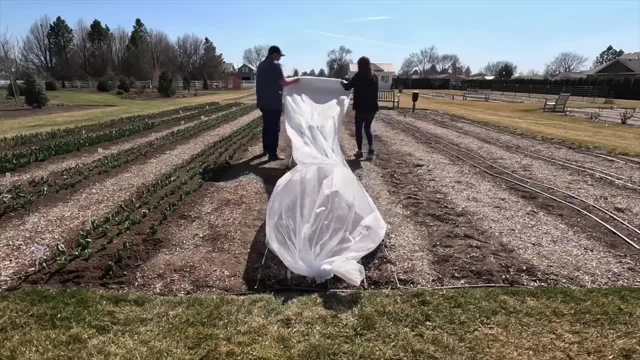 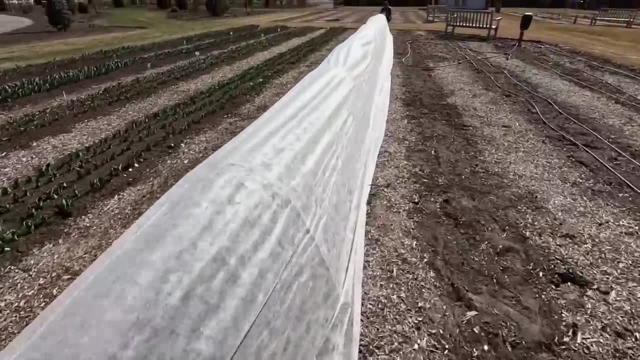 tremendous amount, but this one was so easy and I bought it from Never Sink Farm Tools Tools, Never Sink Farm tools. I don't know, Maybe you're right, Never Sink Tools. You might be right, I don't remember. We linked it down below, but they had a reel on either Facebook or I don't know. 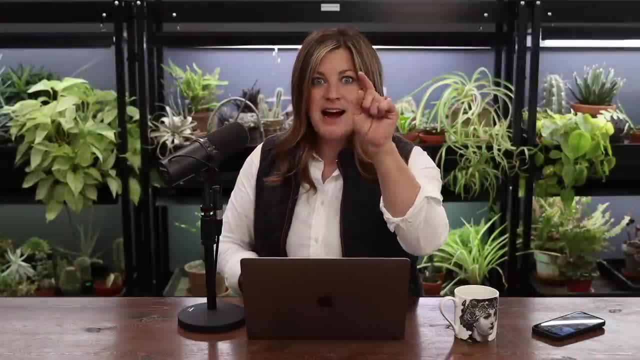 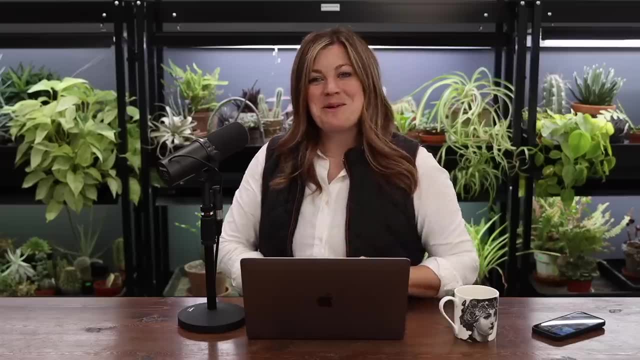 where I was at. but I saw this reel and I was like that, I need that in my life. So I got on their website and ordered one: Never Sink Farm, Never Sink Toolscom. See, we were both right, So you probably type in either one Sure And you would get there. Anyway, it's just like it's. 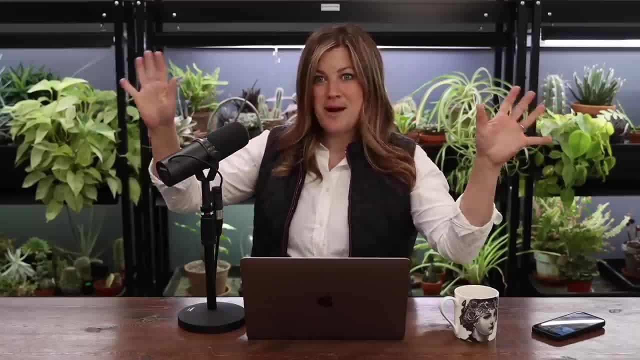 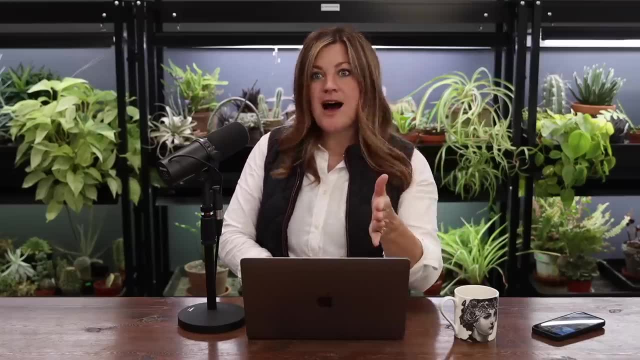 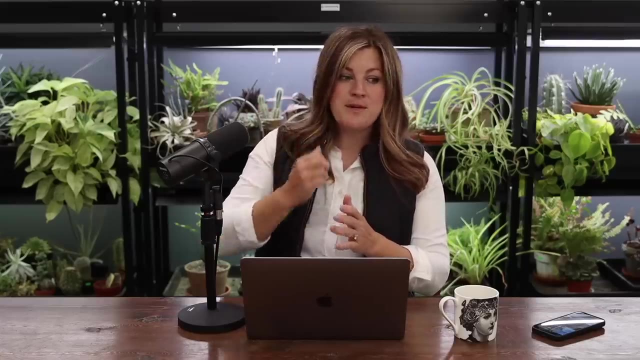 like kind of plug and play, Like you just put your fabric on. It was so easy And then the ranunculus looked really good. We got them all fit in the area. but I took my time, Like we. I measured everything out. Everything's very tidy. I had to rerun the drip tape, It's just all very. 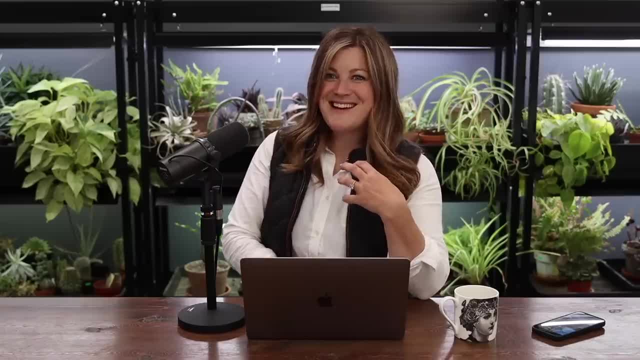 yeah, I don't know. I don't normally measure stuff, So that to me is like I feel so accomplished. I did have to have Aaron come out and look at it. He was like you're off by like six inches, So I did have to move it. 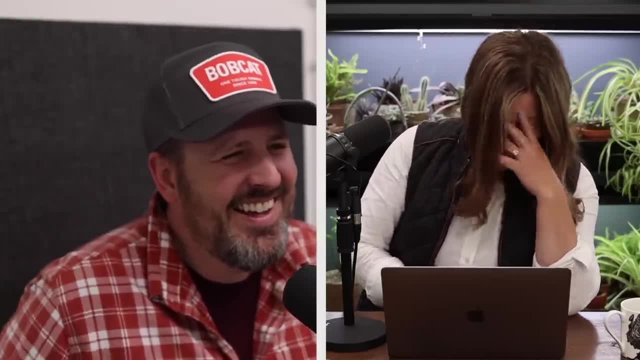 You were too. We cut that out of the video. Well, you know what I think I did? I edit that video. I don't remember. Yes, you did, I think I edited it and I so I cut it out because it wasn't. 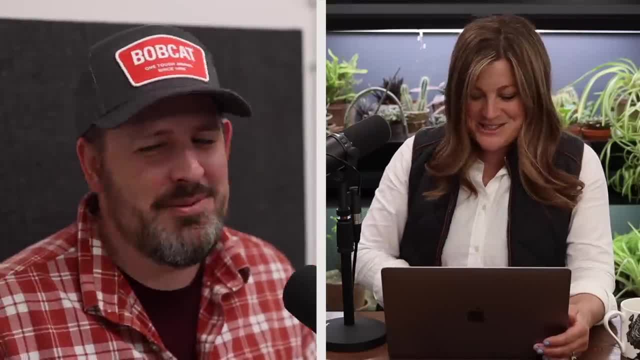 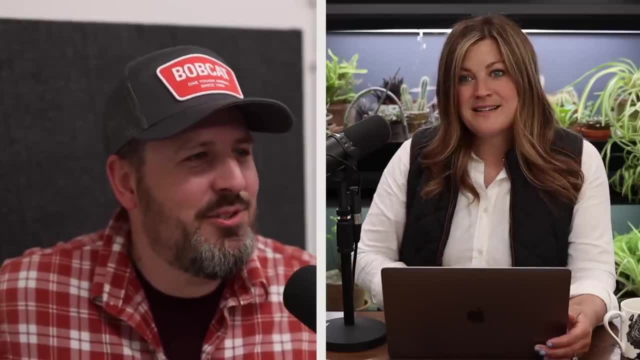 Thank you for that. You made me look so good in that video, Like I just had it together with my measurements. but I know my weakness, That's why I had you come out. I noticed that you cut out a section because you were like. you were basically like an infomercial to me. You were telling me 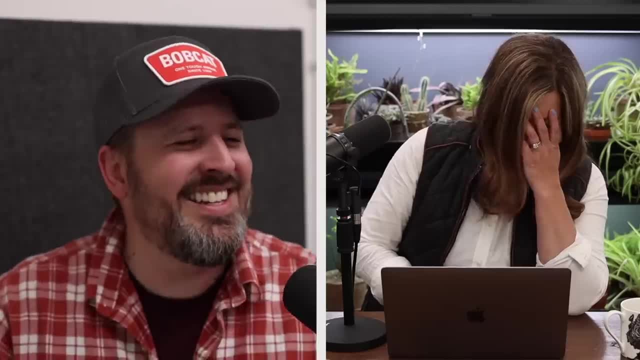 like: this is amazing, And you were kind of like it does this and this and this, But I wasn't looking at that. I well, I was just holding the camera kind of like, as you were, I didn't know you. 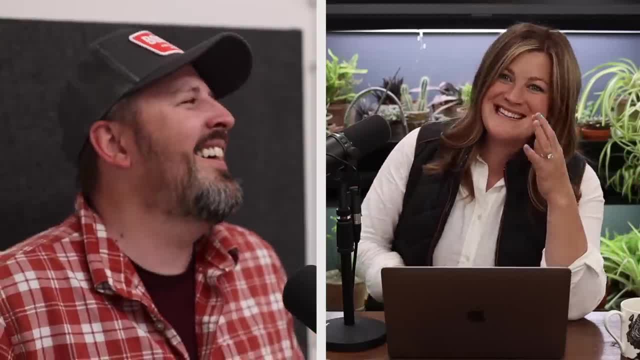 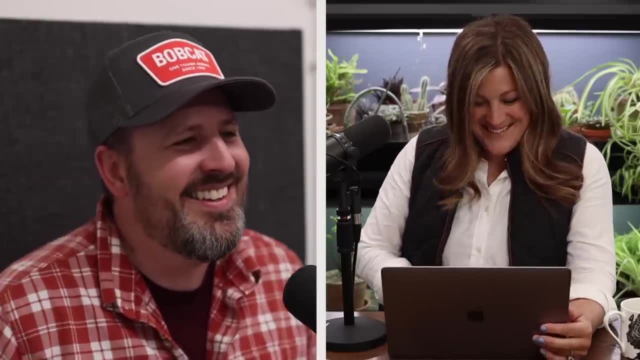 I didn't know you were filming that though. I was like just this is amazing. But I saw you cut that part out too, Cause you were like you were going hard on, like everyone needs to have one of these things. It was a little much when I watched it back. Uh, RSK prod said I tried to pre-sprout. my vernacular About three weeks ago. I soaked for three and a half hours and put some soil in them And then I put them in my garage where it's cool, but they should be protected from freezing temps. So far, no growth at all. What did I do wrong? Any chance they could still root Boy, if you're not seeing, 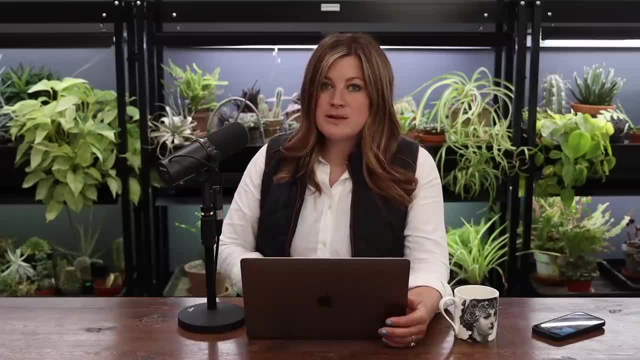 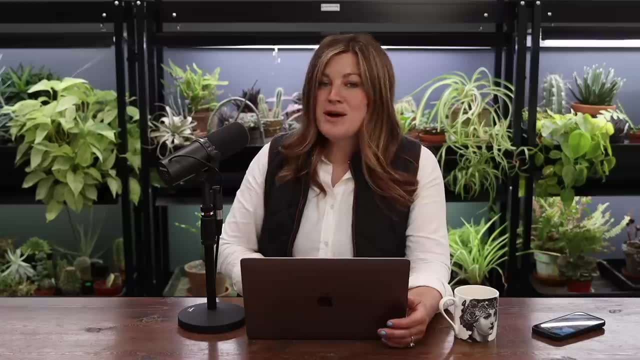 any roots yet put them somewhere warmer. I mean, that's the only thing that I would say to do: make sure that they're staying moist but not soggy, So they're not rotting. If you don't get any action after that, you can toss them in the ground if you want to, but they might just be bad. 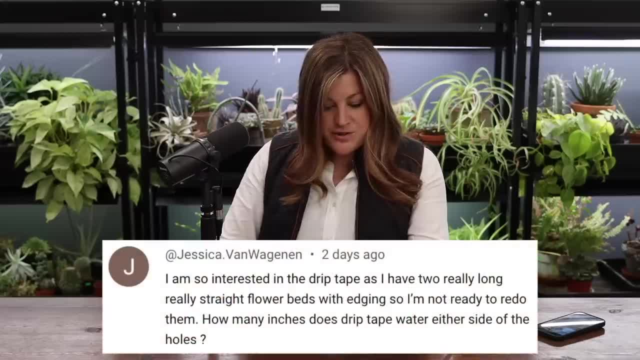 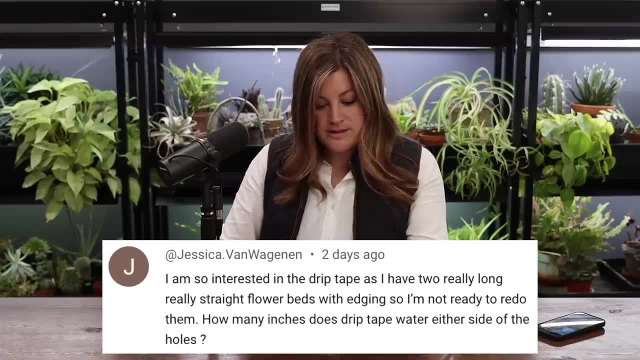 if you're not seeing any roots come out. Jessica said I'm so interested in the drip tape as I have two really long, really straight flower beds with edging So I'm not ready to redo them. How many inches does drip tape water either side of the? 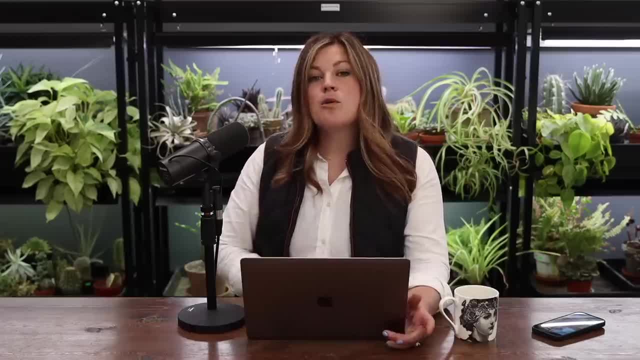 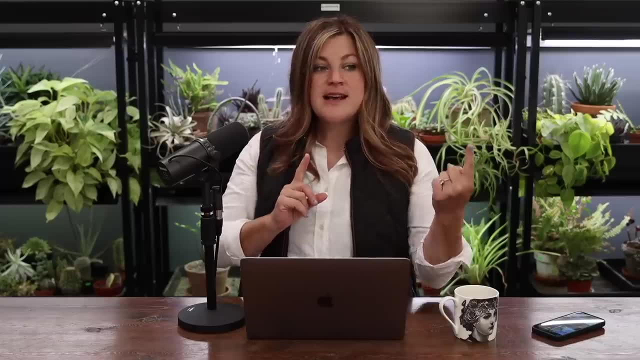 holes Depends on how long you run them, Like that's. I will say that we have tried the drip tape with emitters every six inches and the emitters every 12 inches And even though, like in the dahlia rows, I'm planting my dahlias every 12 inches, We pulled all of the 12 inch spacing. 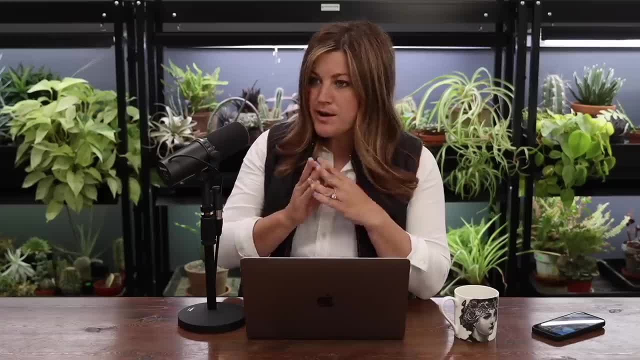 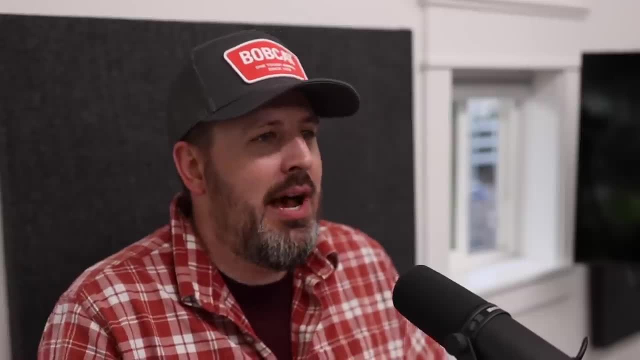 and put in six inch spacing because I felt like the coverage was so much better and my plants were happier and we didn't have to run it quite as long. So 100% has to do with how long you want to do it. It'll sub out farther and farther. And also keep in mind too that like um it's, it goes like a. 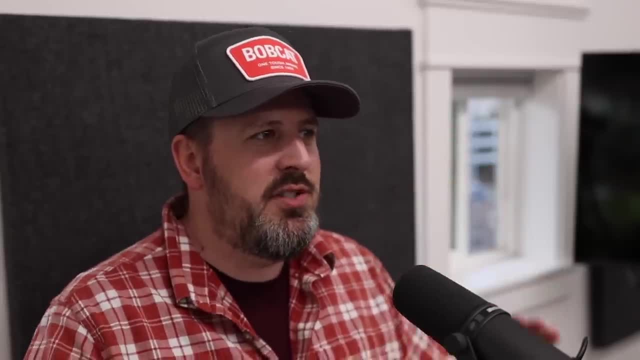 kind of a triangle or like a cone, shaped a little bit. So if you see how far it's subbing on top, it's probably going out farther down below. Yes, Brian said I purchased for Nucleus. I'm in zone. 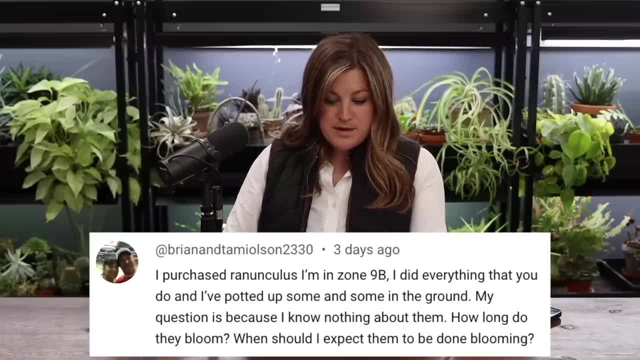 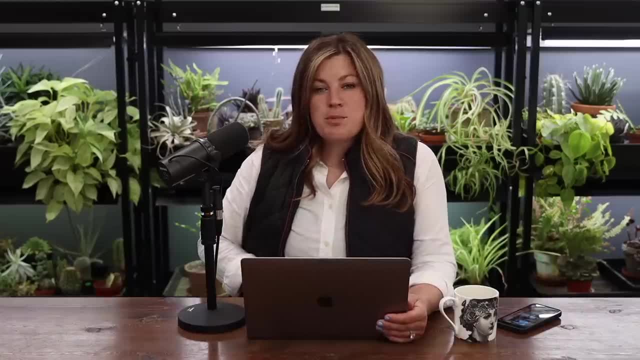 nine B, I did everything that you do And I potted up some and some in the ground. My question is because I know nothing about them: How long do they bloom? When should I expect them to be done blooming? They usually start blooming about 90 days after you get them planted. 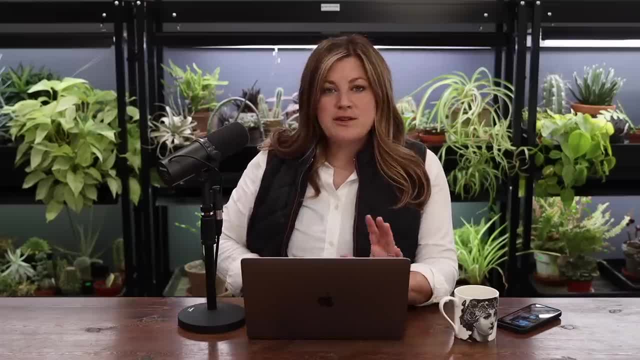 Um, that's just. it'll vary a little bit depending on if you did the pre-sprout process or, you know, if you had them in a warm spot before you planted them out, but it's typically right around 90 days. And I want to say that they're in bloom for some weeks outside, because you know the plant will continue to push blooms, Um, but they last, for they last forever. The flowers last forever in a vase, like upwards of two weeks or more in a vase if they're harvested, like at peak, which is not. 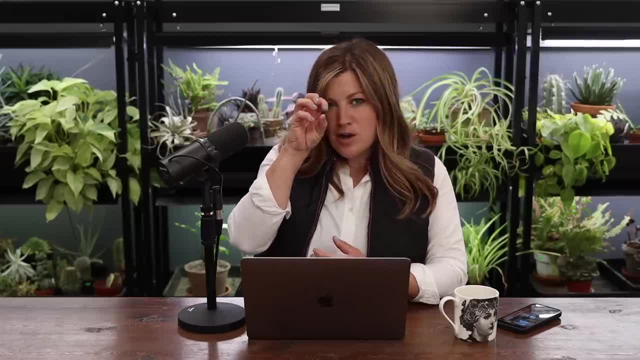 when they're fully open, It's when they're kind of marshmallowy, like they're all. they're kind of closed like this, And if you're in a vase they're kind of closed like this, And if you're in a vase. 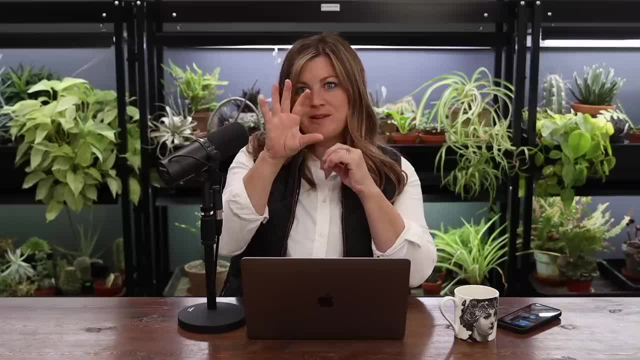 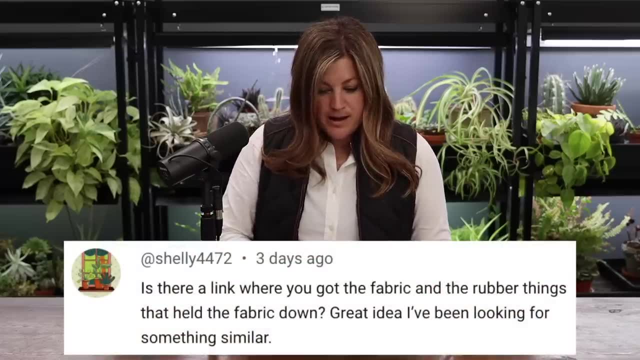 you can kind of do this thing and they've got like a marshmallowy bloom and then they will open in the vase and they last a really really long time if you swap water and all of that business. Shelly said: is there a link where you got the fabric and the rubber things that held the fabric? 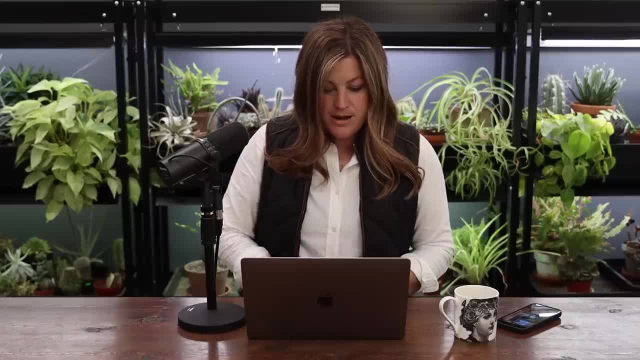 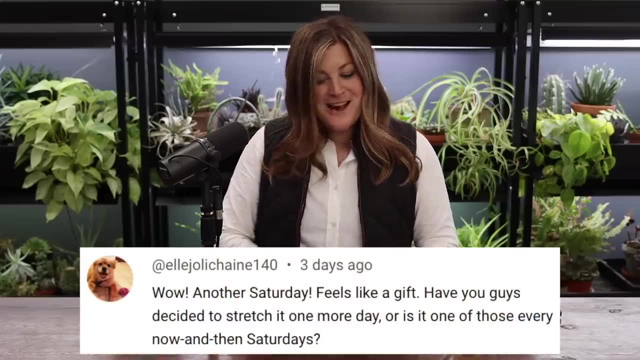 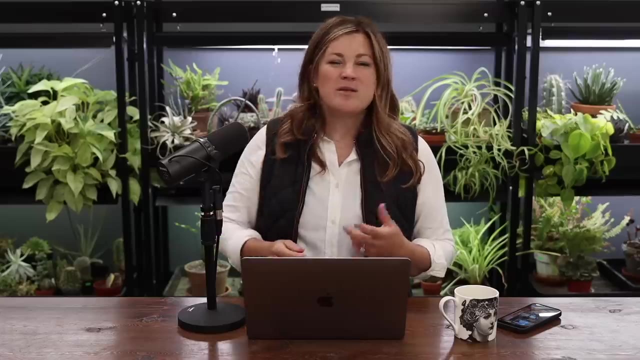 down. Great idea. I've been looking for something similar. Um yeah, we had a link below that video: never sink toolscom. Uh, Elle said: wow, another Saturday feels like a gift. this time of year We just have so many projects going on that it's easy to post a lot more, And we've talked been 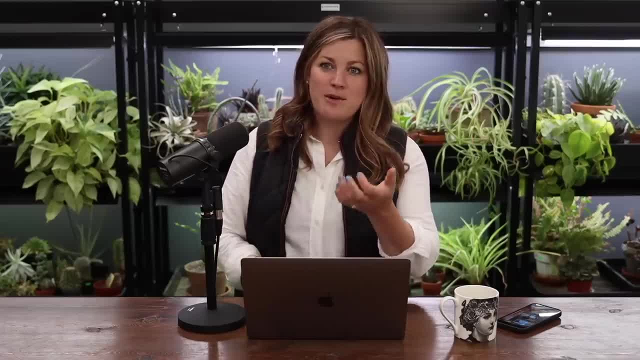 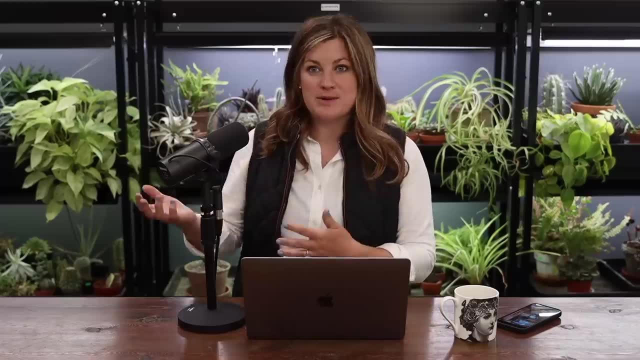 talking recently about how next, like late fall into winter, I think we might like scale about back the amount of videos just during the winter months, And so cause we've been doing five videos a week, plus the recap, even through the winter, And while you know we make it happen cause 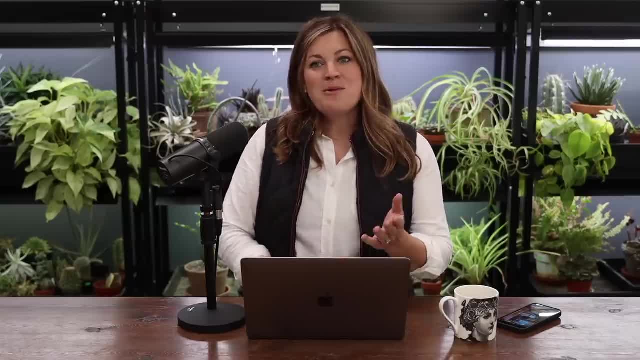 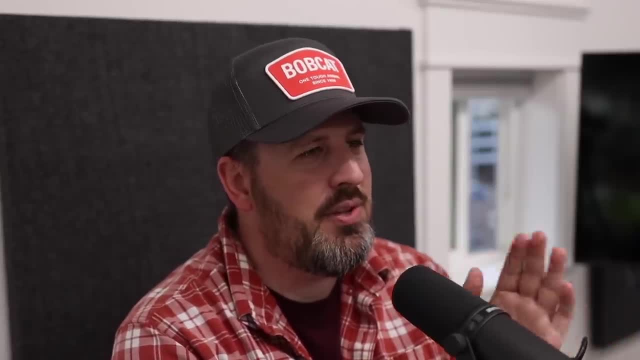 there's still things going on. It would be nice just to like: maybe we'll go somewhere warm next January. You know what I mean? Yeah, There's also. there's also some like projects that I think both you and I want to do that require a little more production. Yes, And they they'll take multiple. 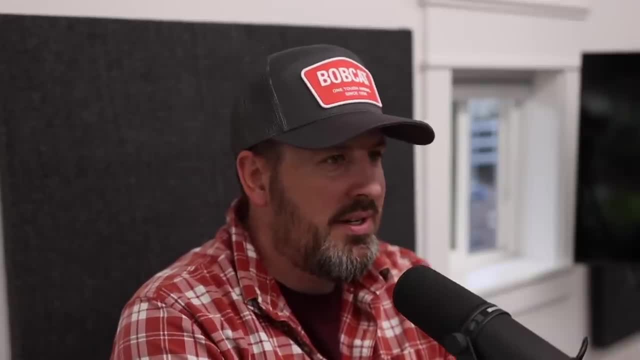 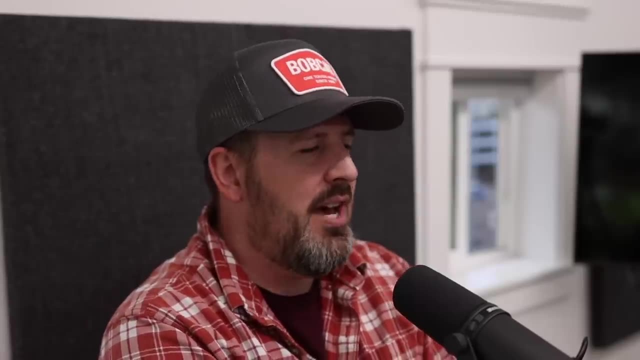 days to do, And so I think if we did like three videos a week- um, maybe three videos plus the recap- Yeah, Not permanently, but just just during the winter time- Yeah, I think we could do some that we've kind of been wanting to do. but yeah, Are are just harder because they just 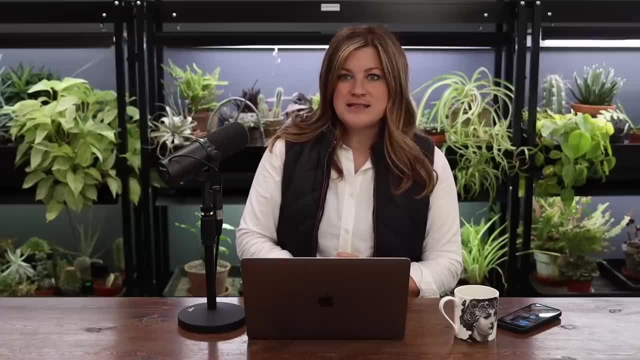 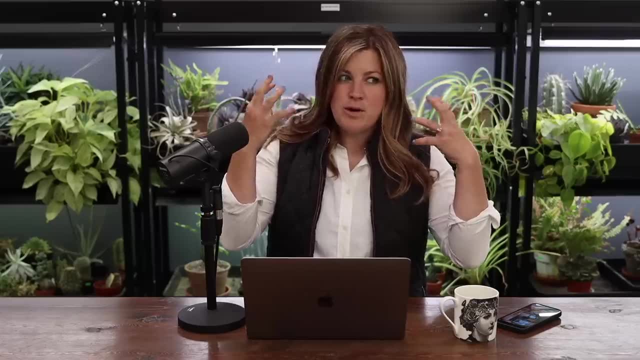 take a lot more work, Right. And you know, there's days where, like I just need days to think like think and putter and kind of come up with. you know, I've got like a little vision in my mind of what I want to do with like a creative project or like how we used to do fairy gardens with water. 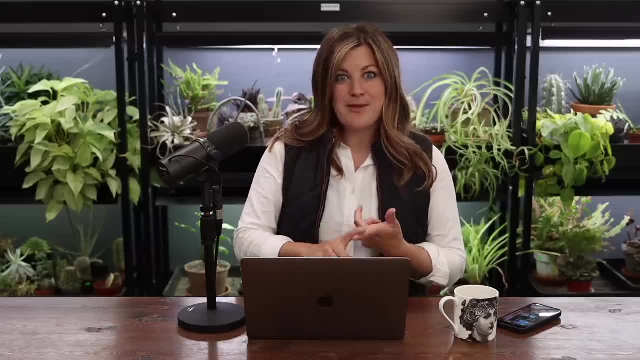 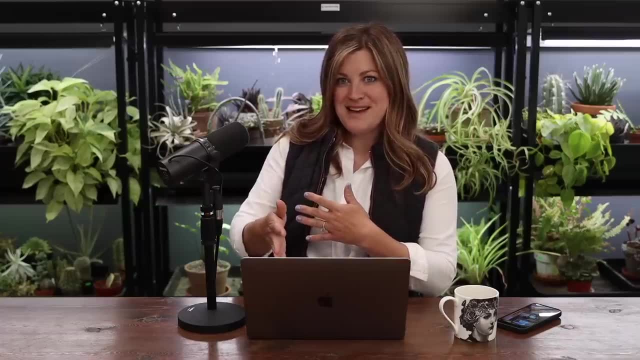 features and things, And sometimes it would take a day to gather supplies, kind of think through the design, see if it's going to actually work, And then the next day you try to execute. And sometimes even then you don't execute very well and it takes the third day to get it all the way done. 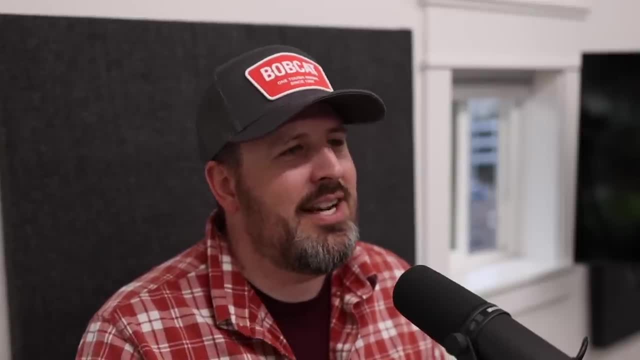 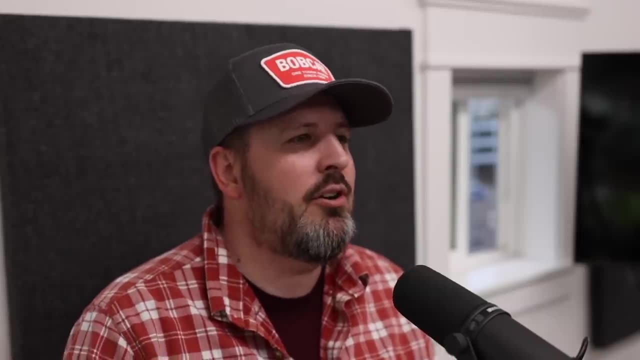 And I think that you used to really like doing, especially like decorating projects, decorating the house or things like that. It's so time consuming, It's really time consuming, but you enjoy doing it. I think, like I want to encourage you to do the things that you like. 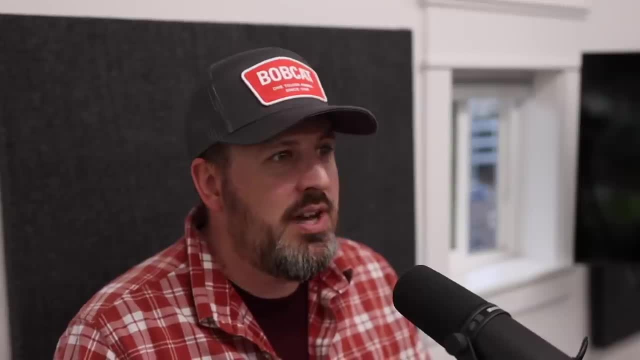 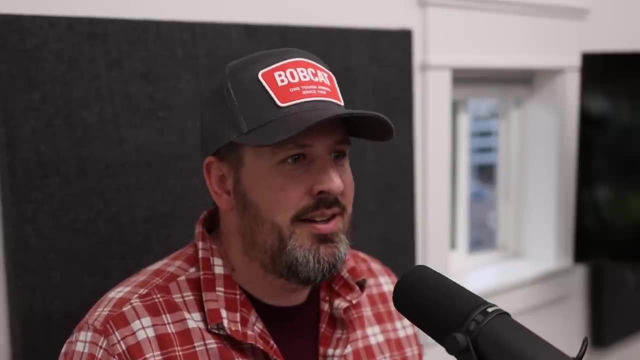 doing and don't feel like you've got this time constraint, like, Oh well, we've got to stay on this schedule. Like, if we skip days, that's totally fine. Like, do what you like, do what you enjoy, keep it fun. And you know, yeah, Not that it hasn't been fun, We're just like thinking forward. 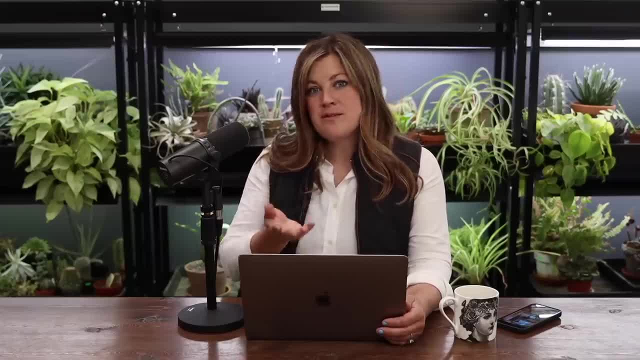 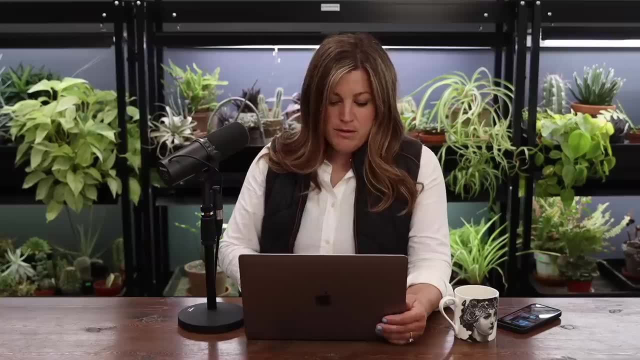 you know, and I used to love all the decorating projects, but I don't love them as much when I feel like the pressure to like I've got to get it done. when it's light outside, you know, that gets to be a little bit, Oh, but this time of year it's like. 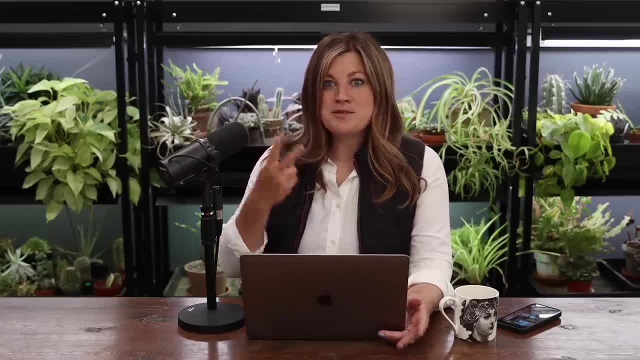 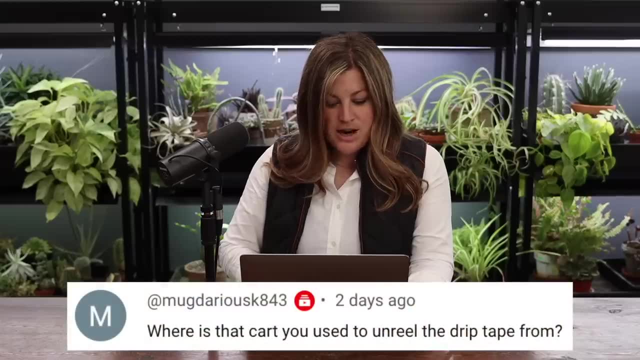 I could do multiple projects in a day. Yesterday I filmed two videos. Well, you have, like the sun is out, like literally twice as much, right, You know? Yeah, Mug Daria said what? where is the cart you use to unreal the drip tape from? 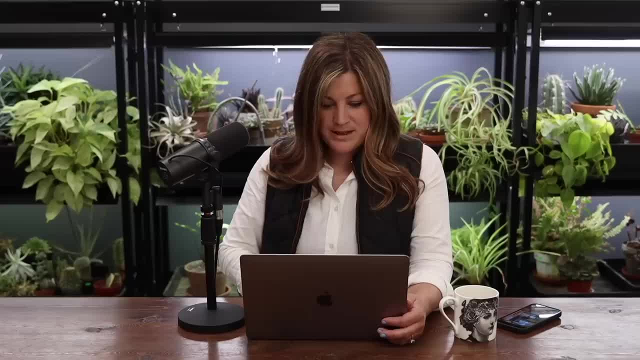 I don't know Where's that from. I think I ordered that from home Depot. Really, Yeah, It's handy, Handy, It's just a well, you can make it wider, or I ended up and I don't know if I. 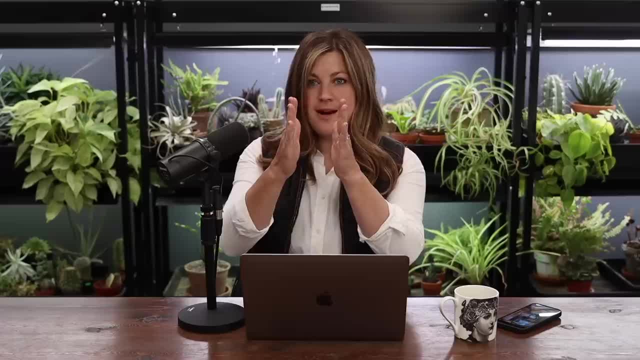 it showed it all the way, Um, but I ended up making it real narrow, So it kind of pinched that really skinny roll. They sell those for all sorts of things, Drip tape, I mean. like electricians use them. 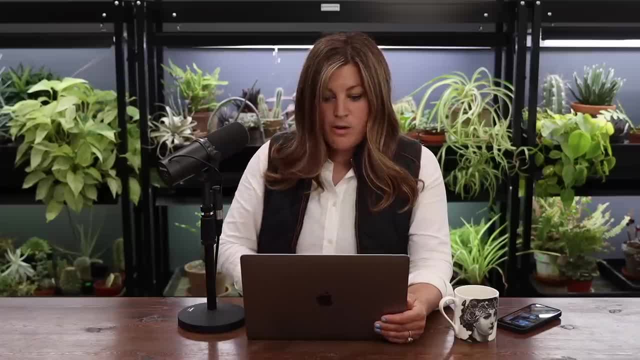 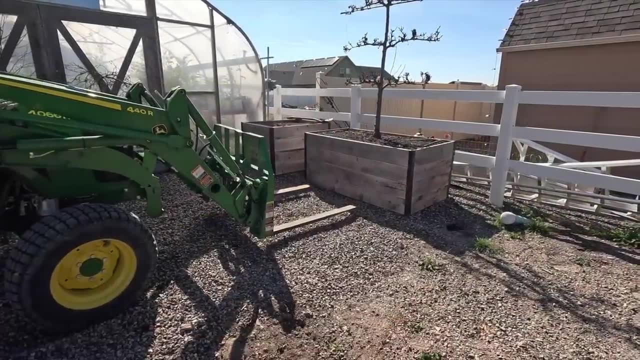 I'm spooling any kind of wire I would imagine. Yeah, Okay, Okay. Next video was Elm tree removal, new stump by the pond and moving a honey locust tree. We started that video out, trying to move that raised bed with the. 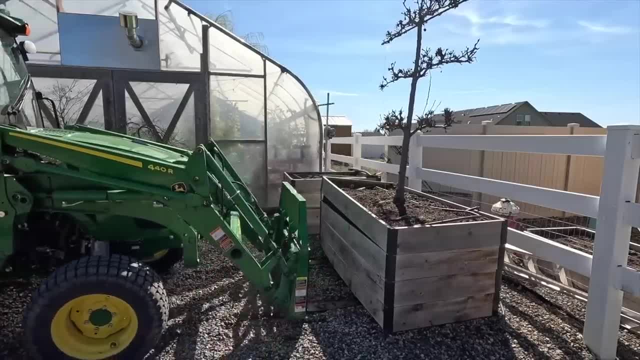 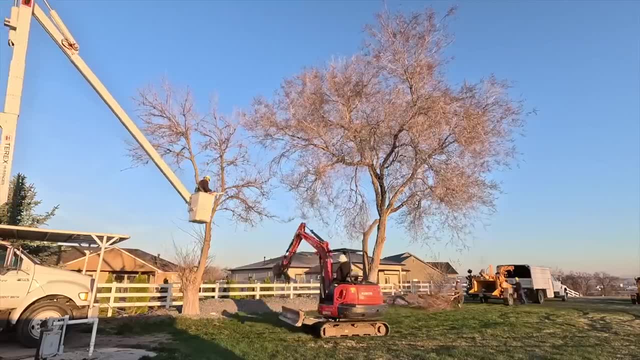 espalier in it with the tractor, so disappointed in that tractor did not happen. Um, so we abandoned that project. but right after that the tree crew showed up from natural tree and they got those two. actually, one of them was a mulberry, The other one was an Elm, Both were, I mean. 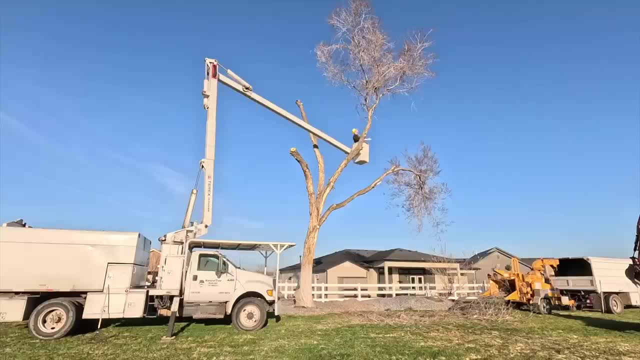 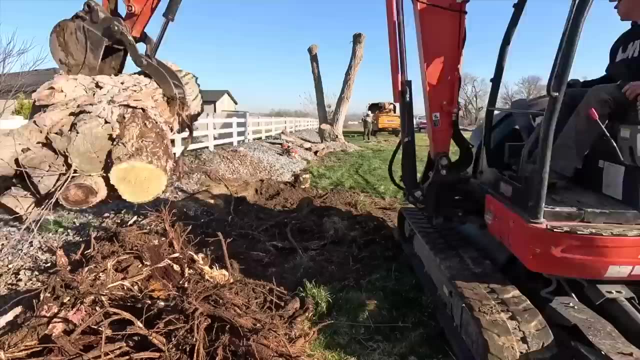 you saw them like falling apart trees with multiple branches, like trunks cut off at the base. Um, so we got that handled. Our neighbors are thrilled They're gone, which is great, Um, and that we both got thank you texts. 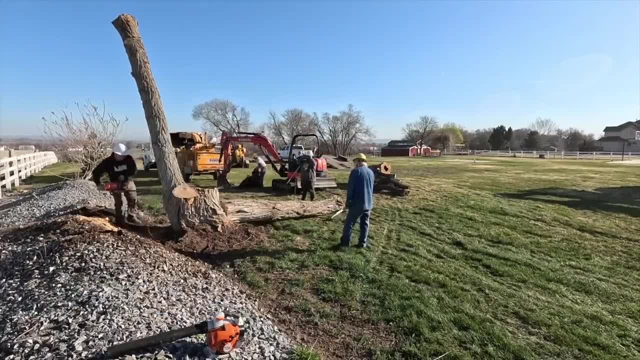 Like: thank you for doing that, which makes you feel good, Like you just did something to benefit not just yourself, but somebody else, And I hope they like the new trees when they go in. Well, I wanted to ask them like: 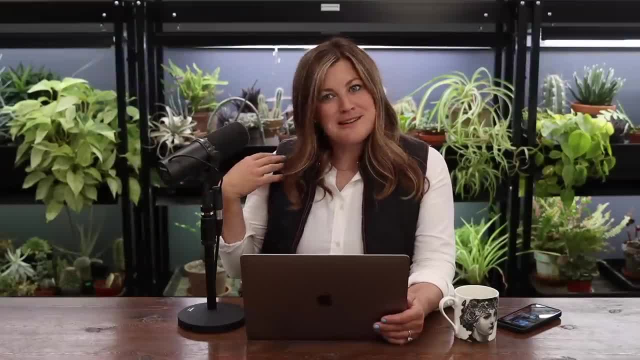 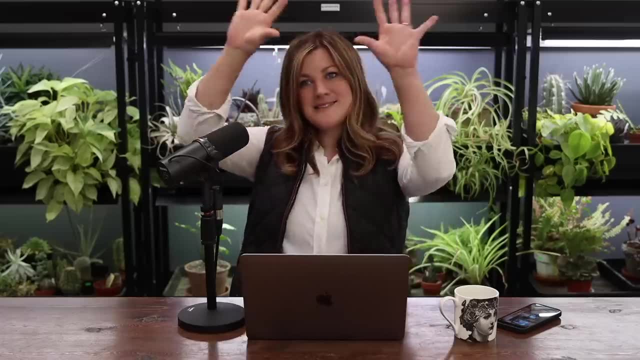 is there anything in particular that you haven't been able to fit into your garden but you'd really like to look at? Oh sure, Like, maybe they like a Magnolia tree or something like that, you know, and maybe we can back one so that they've got this nice. 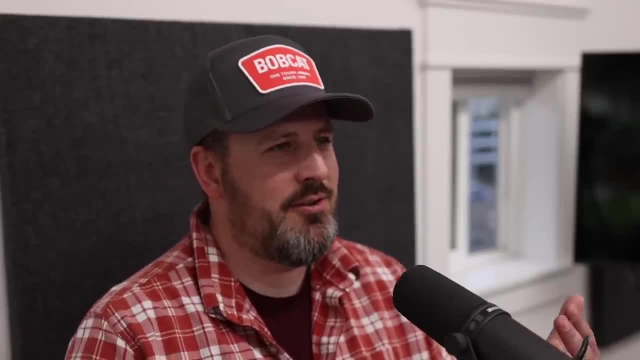 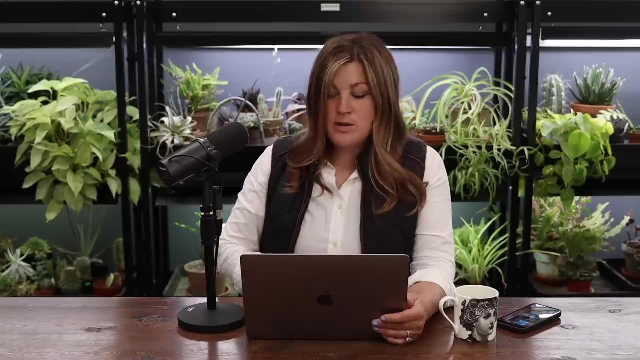 I don't know full hedge though, So like they're going to get evergreens either, either, Yeah, But they'll be able to see some deciduous, pretty stuff too, So, and they like all of it. They. they're really good gardeners and their garden is always like pristine, Yeah. 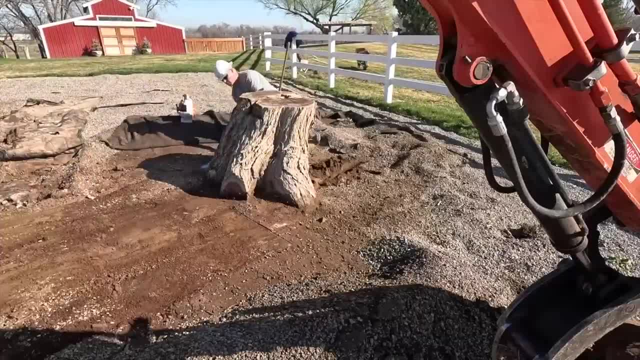 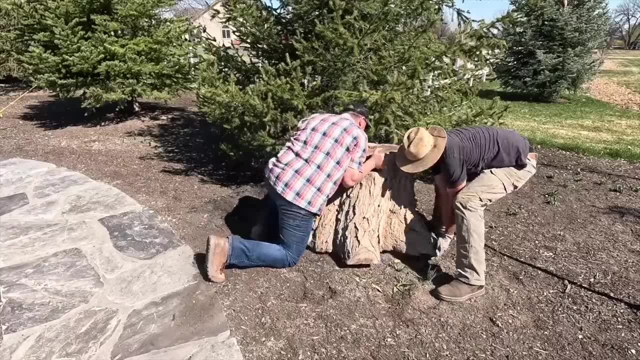 Yeah, And then we did um: cut the natural tree, cut the big stump from the chicken coop area in front of the new red barn, And we moved that over to the pond area and Paul and Aaron had ended up having to get it in place. I tried, I couldn't even. I couldn't even like nudge it. 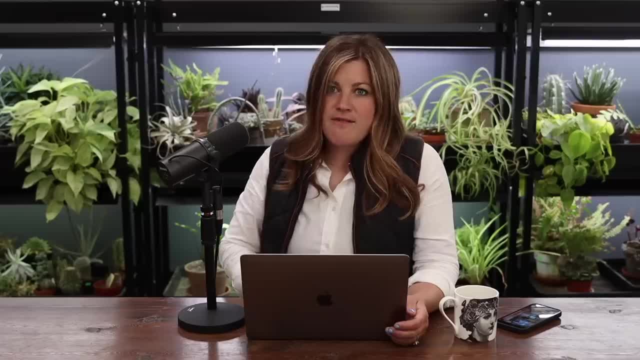 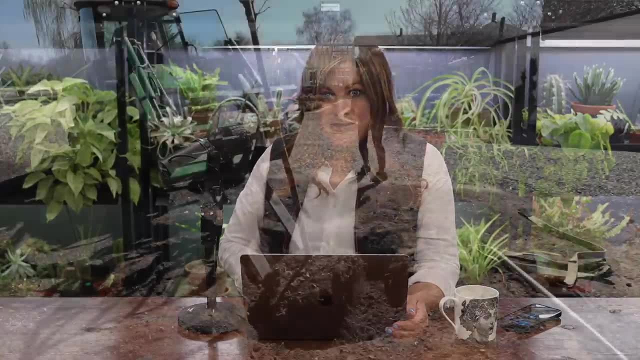 What did we guess that it was like 300 pounds, I don't know. It felt so heavy, I bet. Well, I mean so so heavy for. and then we moved a shade master honey locust tree, which we planted last year before we knew we were going to buy this property. 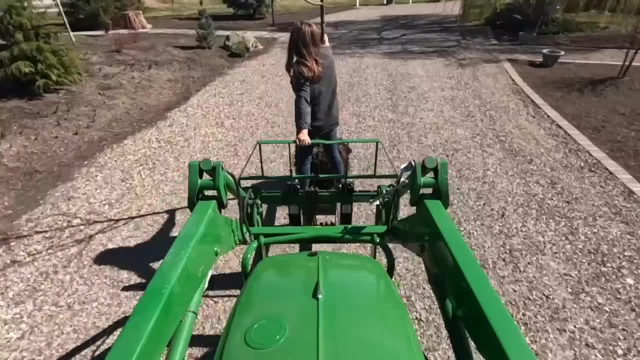 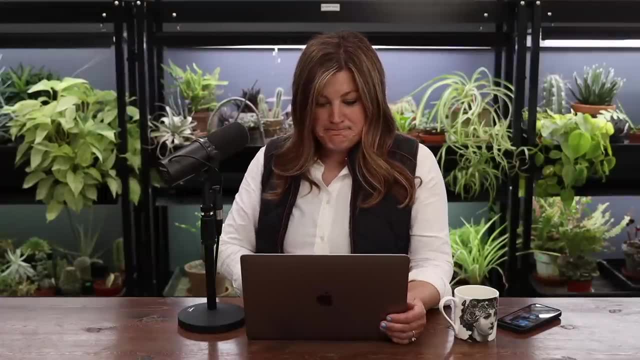 And, um, it was right in the, the area where the new lane needs to go, So we got that out. Chad never got here last week, So hopefully he gets here this week at some point. we're here in the middle of the week. I'm like hello, Um. 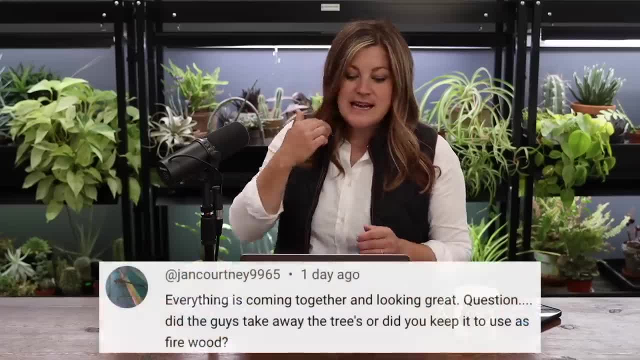 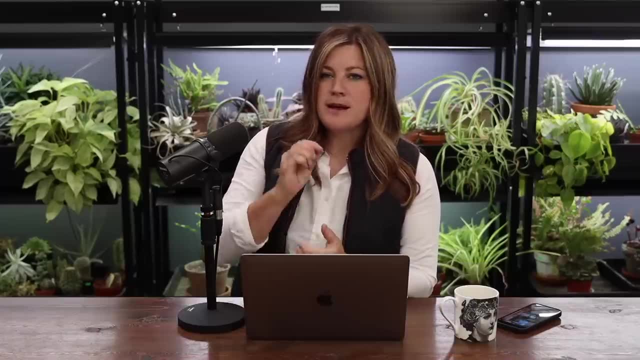 but it's all prepped and ready to go for him. Jan said everything is coming together and looking great question: Did the guys take away the trees or did you keep it to use as firewood? They chipped or they, uh, sent most of it through the chipper and we have it all. 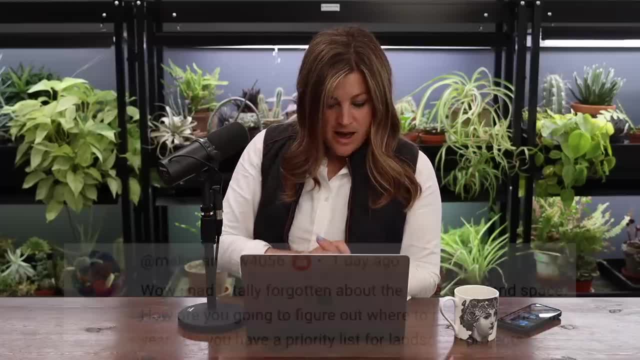 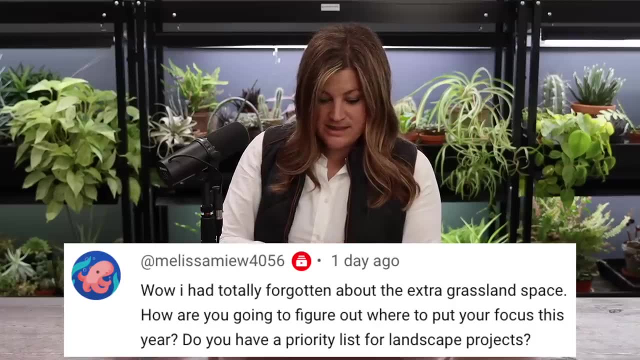 So they dumped it in some piles and we're going to use it tomorrow. Actually, Um, Melissa said I had totally forgotten about the extra grassland space. How are you going to figure out where to put your focus this year? Do you have a priority list for landscape projects? 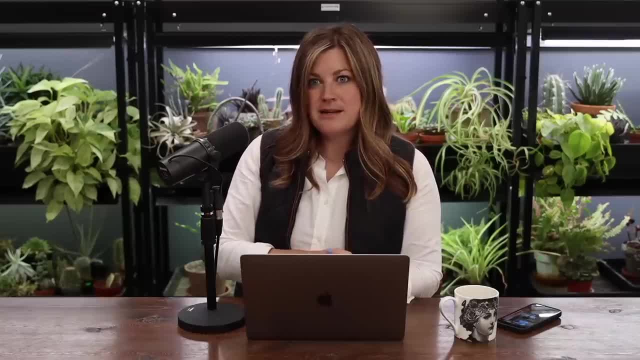 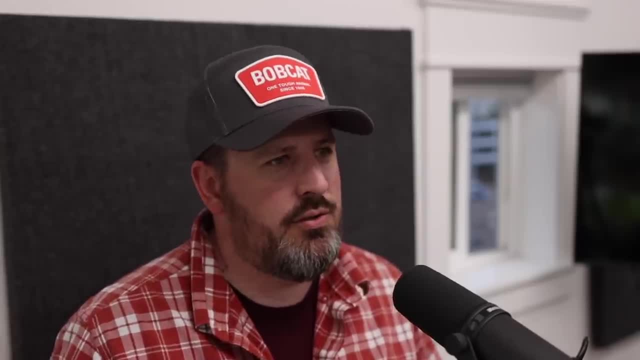 Our priority list kind of falls into place on its own, It seems like so. it's based on how, how many people we can get out to do certain things that we're not they're good at or can't do. Yeah, So it just kind of it. everything just falls into place how it should. 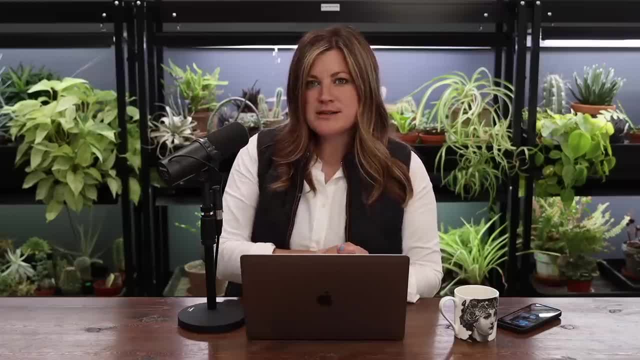 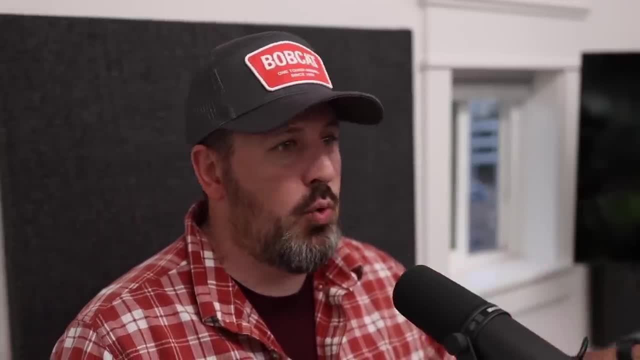 I guess I don't really have a lineup for projects. I feel bad, Like the grass space out there. I don't want more space to mow. The sprinkler system isn't going to work the way that it was designed. We would have to put a new sprinkler system. All the pipes are cut at this point. 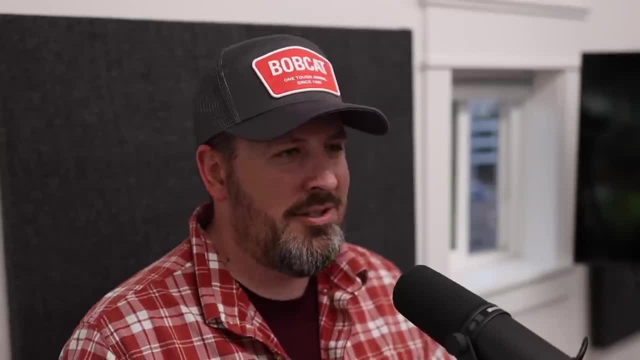 Yeah, And I don't want to. so I don't want to pay to put in new pipes just because we don't have like a full idea. So the grass is going to grow up tall. It's going to look like a pasture out there. 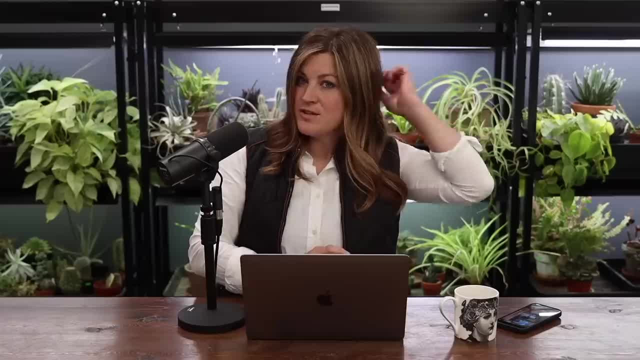 It's not going to be pretty this year. No, I'm fine with it. Neither the dirt lands, like the grass in front of the Persephone garden, will turn to look like the dirt lands until we can get all of everything figured out. Yeah. 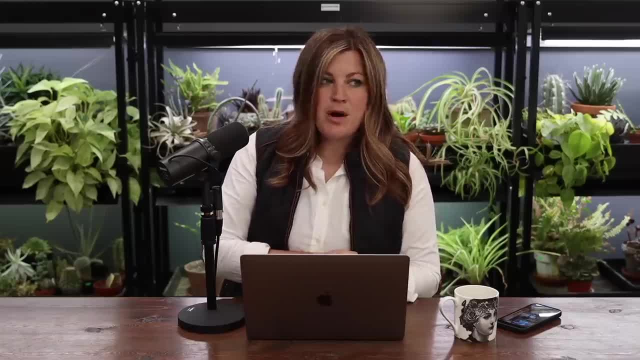 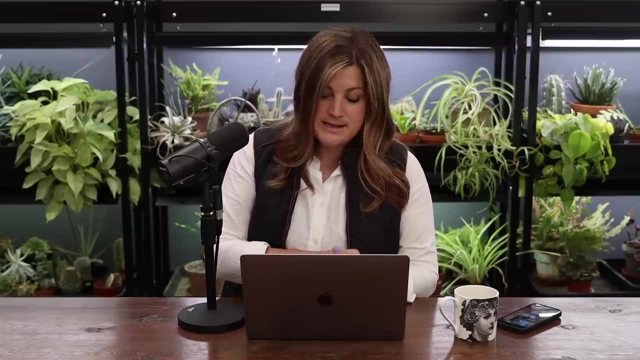 So you have to go through the proper avenues to get you know all the proper things in place so that you can use your property the way that you want to. or or maybe you need to adapt, to move it, to use it a different way. 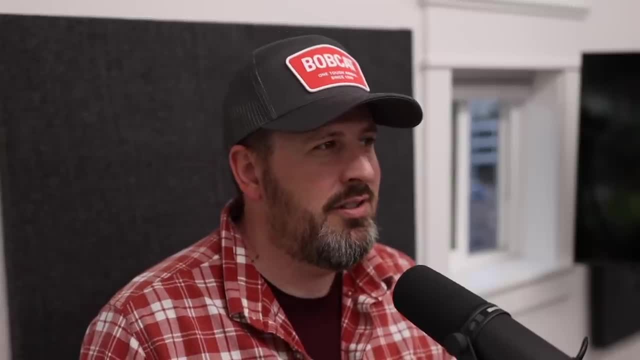 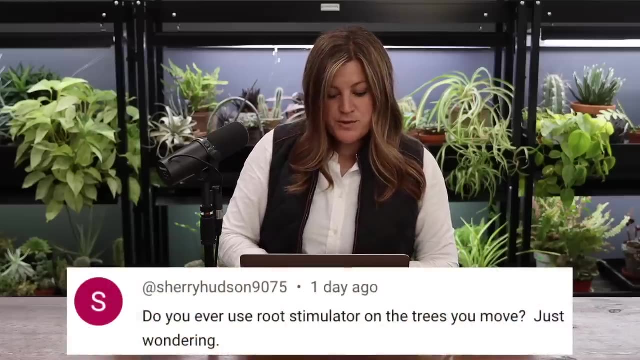 So anyway, we're just kind of waiting on all that. I just don't want to be rushed into coming up with a design, and I don't. I also don't want to do it twice. No for sure. Sherry said: do you ever use root stimulator on the trees? you move. 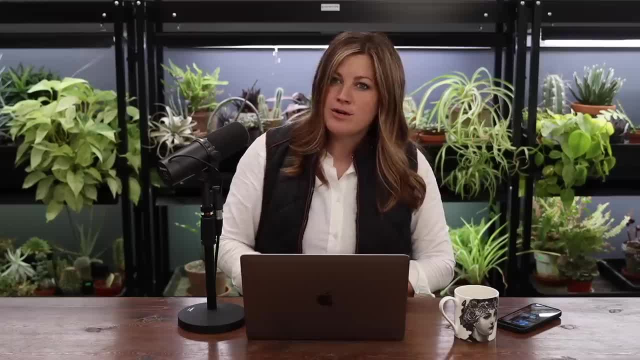 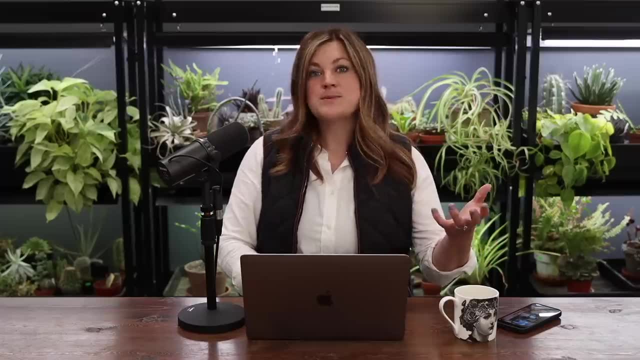 Just wondering. I used to all the time and I don't know why I stopped using it. I don't really think about it. I think just using the biotone because that's like mixed specifically for root development. That's been all we really needed. 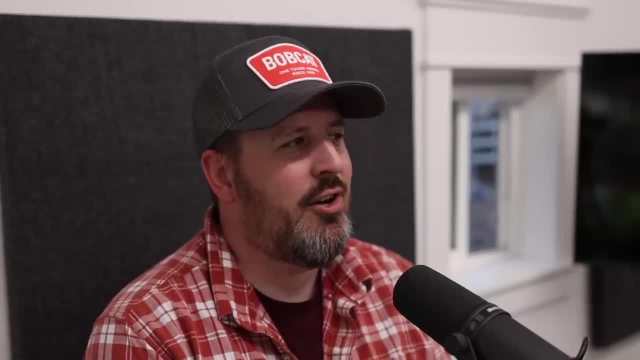 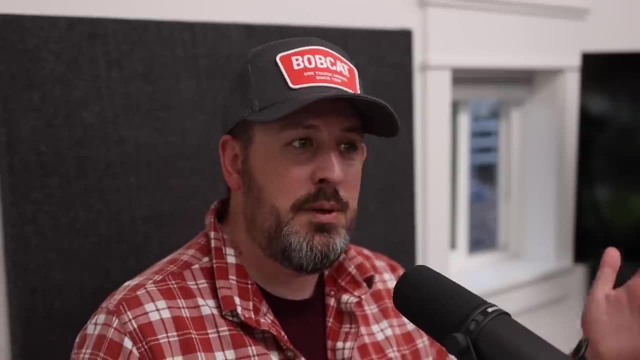 Everybody kind of has their own thing. that it's. it's hard to really, you know, when it comes to moving things like that, it's hard to say what really works. or doesn't You just kind of start using the things that other people talk highly of, because 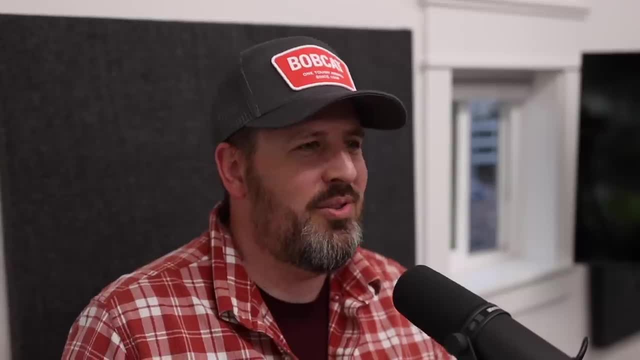 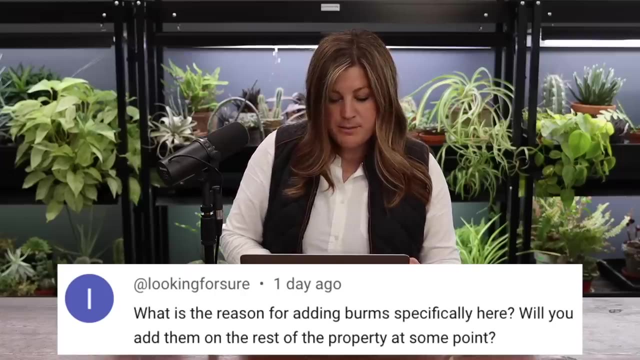 it's like, unless you have an AB test, it's hard to really know what. if the root stem is working better than whatever else you're using. Right Looking for sure said: what is the reason for adding berms specifically here? Will you add them on the rest of the property at some point? Well, back there. it's just seems natural because there already is one there and we can just build that one up. It'll also help us create a little bit of elevation for more of a hedge quicker, because I do think we want to move high tunnels not right up next to the fence. 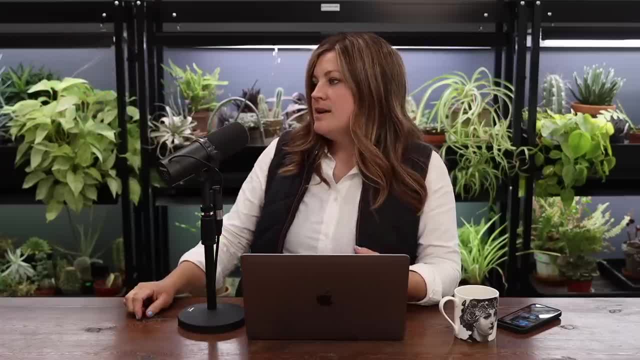 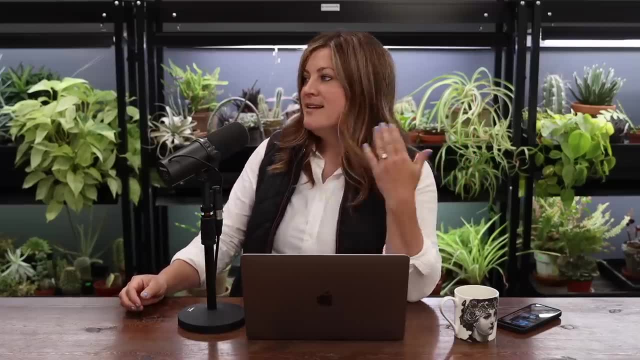 but some more back in this area they'll end up, And so I want to have some privacy for- not for us, but for the Nate, for the neighbors sake. I want there to be a nice thing for them to look at, because that's. 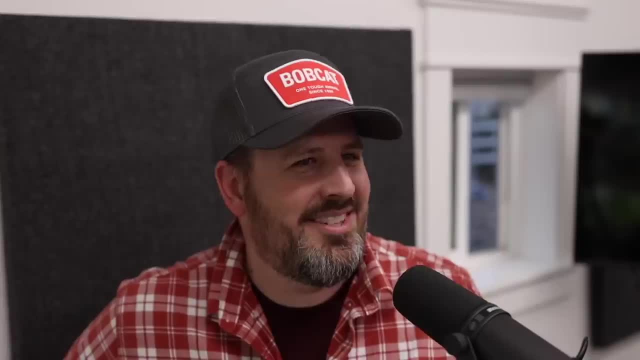 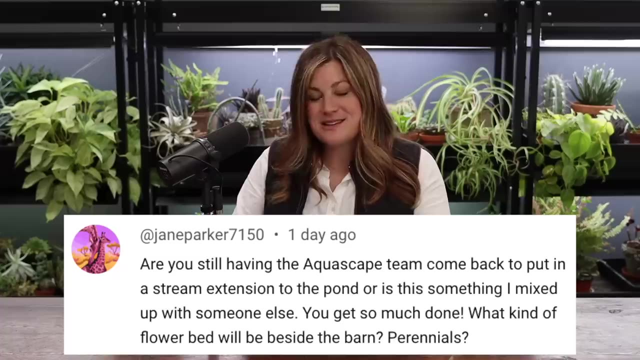 that's what I would want for myself from neighbors. Yeah, Yeah, I think we talked about that last time, I think so. Uh, Jane said: are you still having the Aqua scape team come back to put in a stream extension to the pond or is this something I mixed up with someone else? 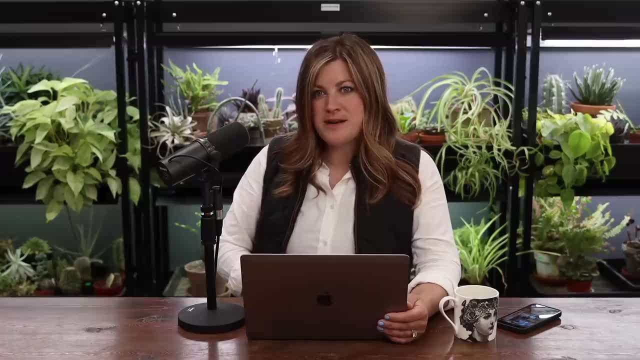 You did not mix it up with somebody else. In fact, part of the team is going to be here next two weeks from now. Yeah, Not to do a project, but we're going to be. well, they have to. we're going to be mapping it out. 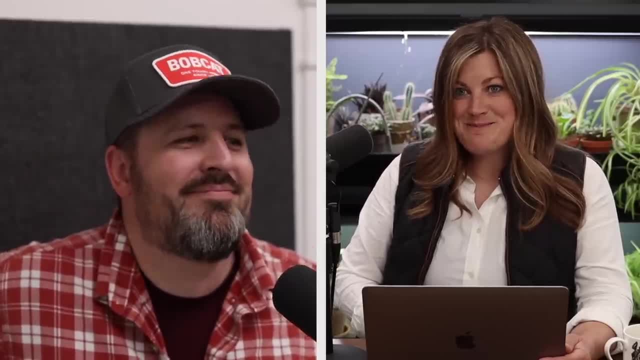 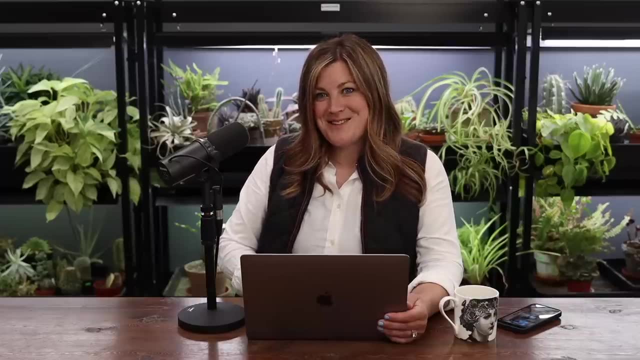 Yeah, Yeah, Come up with a plan. It's going to be awesome. Yeah, What kind of flower bed will be beside the barn perennials? There'll be a mix. I think we want to put a weeping Alaskan kind of in the corner. 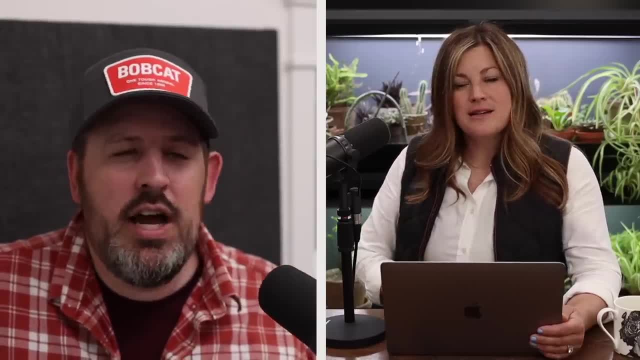 Don't say we, don't say we. you wanted it too, right? No, I have. I have definite: uh, Oh, he wants to block the barn, He doesn't want to see it. but I think there's some charm in that. 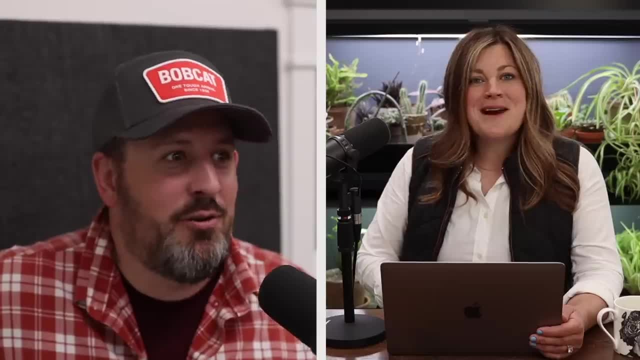 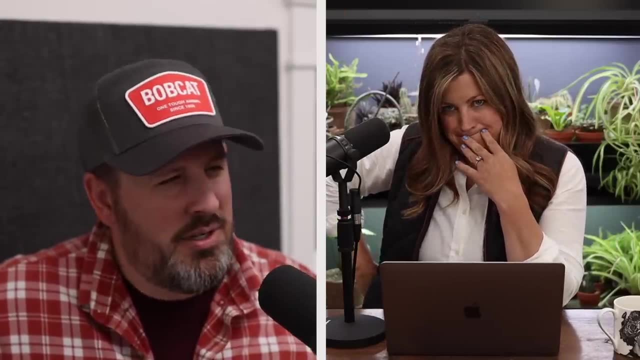 this old barn? I don't know. We'll see. Go for it, We'll see how it goes. What if I covered the sides with like climbing roses and masked it? Is that what you want to do? That's what I could do. 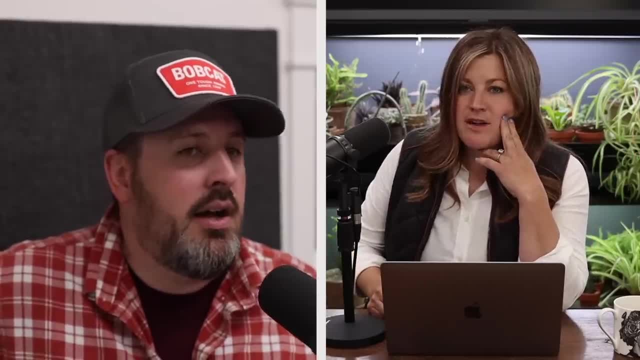 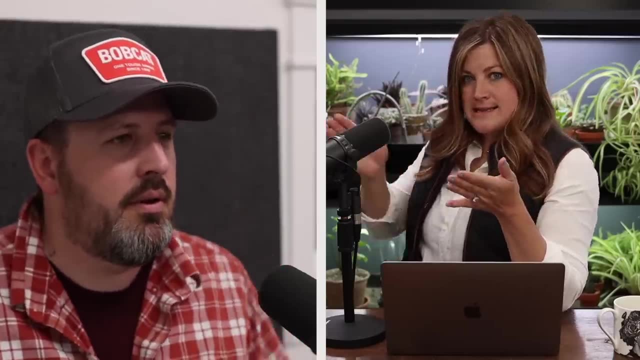 No, I like the barn. I don't really feel a need to cover it. I like the barn. I don't like that view of the barn. personally, I think the side view is the worst view. But I think Aaron on the right hand side of the lane that goes next to the barn to get back behind it. 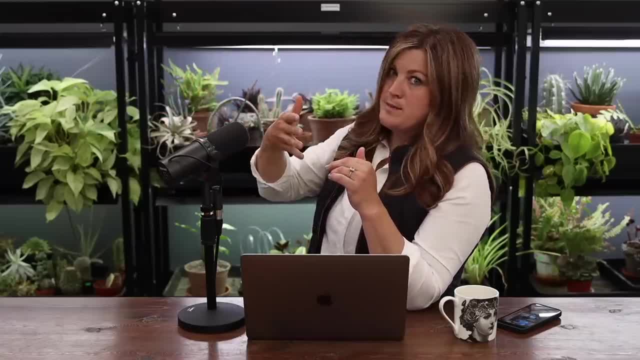 I think that's going to be so heavily planted that when you're sitting at the pond you won't see the barn. But as you go closer to the barn it'll open up a little bit more. So we're not blocking the windows. 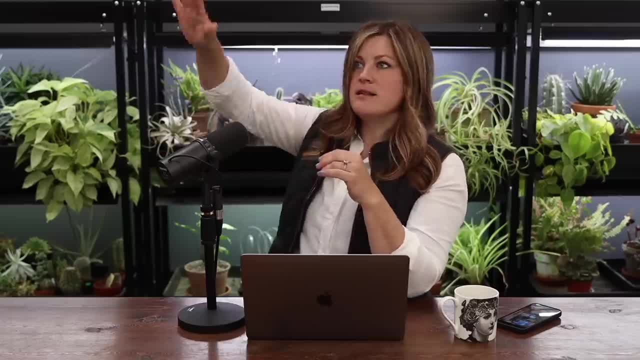 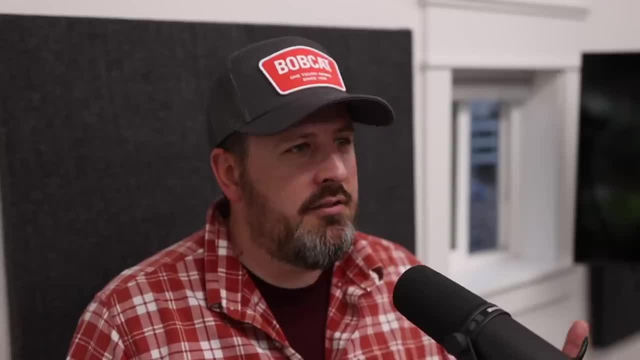 You can still see out the windows and see some beautiful things and the lane, And then like, whatever is mass planted around the stream? I don't, it's not the windows, Like I envision, It's the roof for you. Yeah, I envision like a pine. 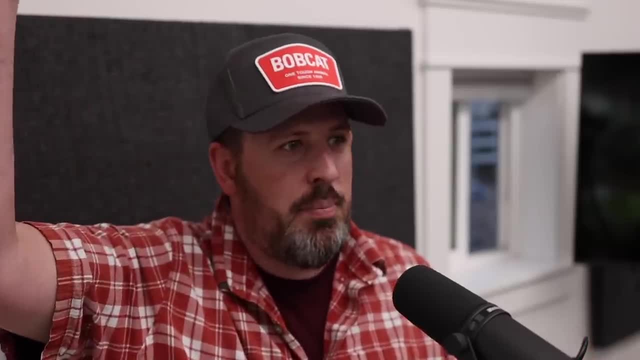 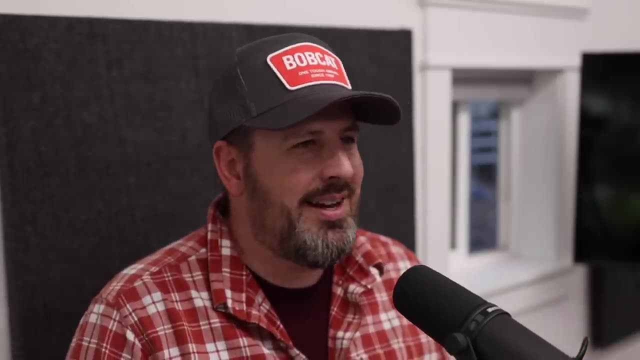 So you're going to have a trunk and then you're going to have this like 30 foot tall pine next to the barn And you'll see like the windows will be exposed. You keep thinking that the wind like it's not about the windows. for me, 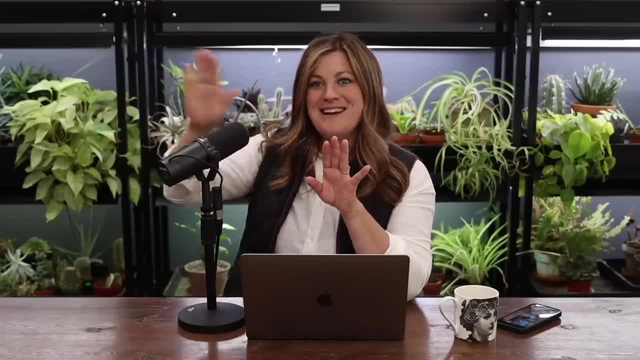 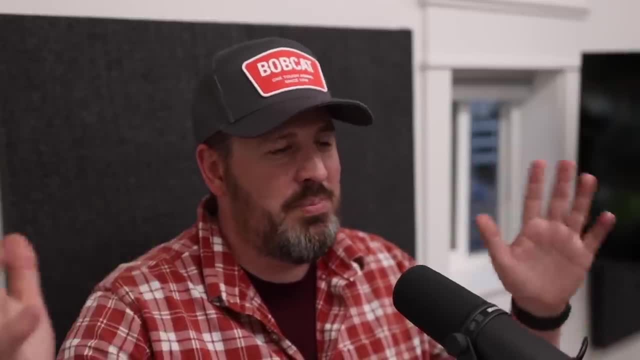 You wanted to plant a bunch of mulad trees. Well, right along the barn We can't. I know Multiple reasons, But yeah, I mean I want. I want big trees to block the barn from basically any vantage point. 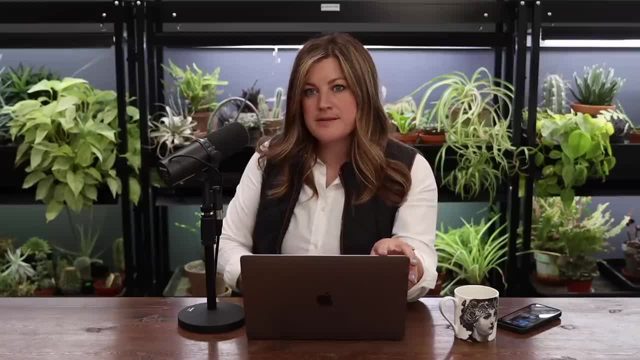 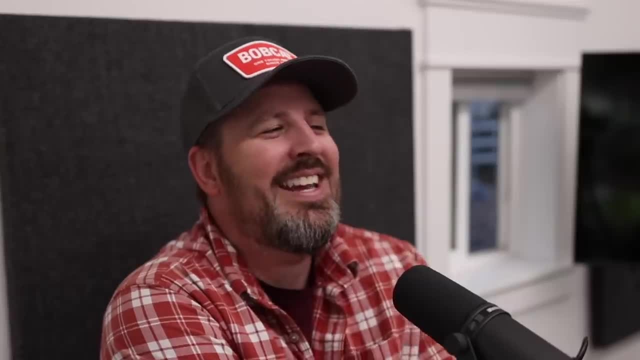 I mean on that side. Yeah, I think it will be. in the end, You can count. You're not going to plant trees. No, I'm going to plant trees. Okay, Just trust me. Okay, Why can't you just explain it though? 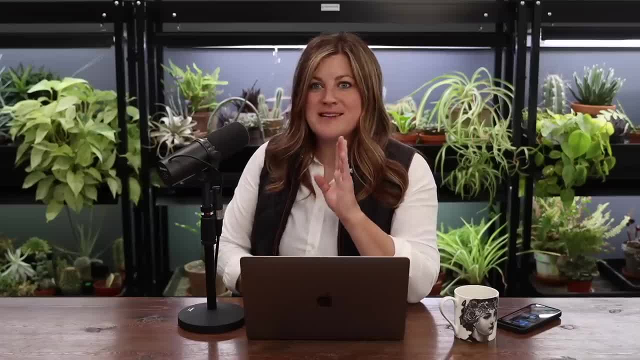 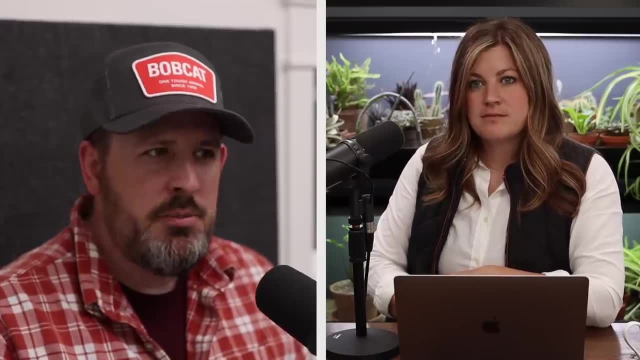 I can't, Because you and I don't, we don't. we don't communicate on the same wavelength about ideas. We do not. I don't feel like I don't feel like you do. you feel like you're communicating. 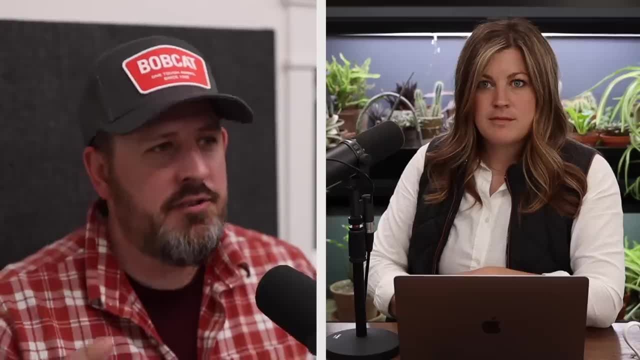 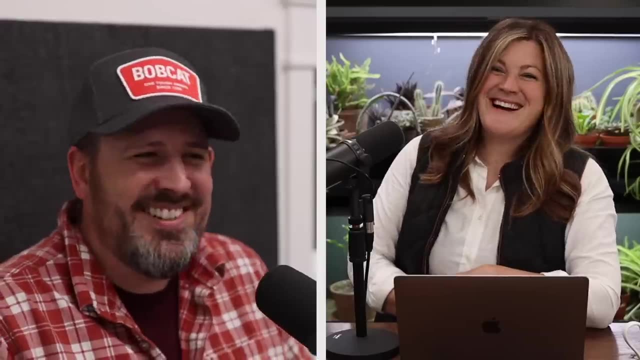 Like when you express what you want to do, do you actually feel in your mind Like I expressed that as adequately as anyone could possibly express it? Yes, Do you really? Yes, I'm always left with like you threw out a bunch of possibilities and you never. 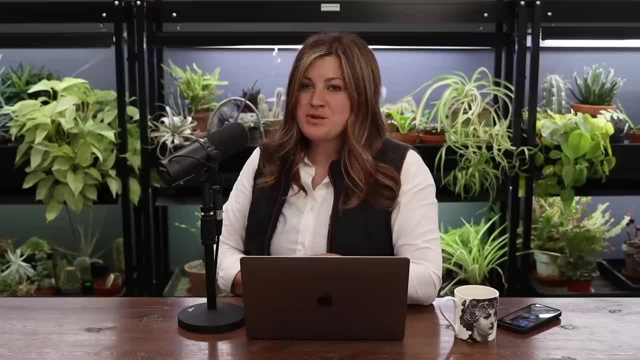 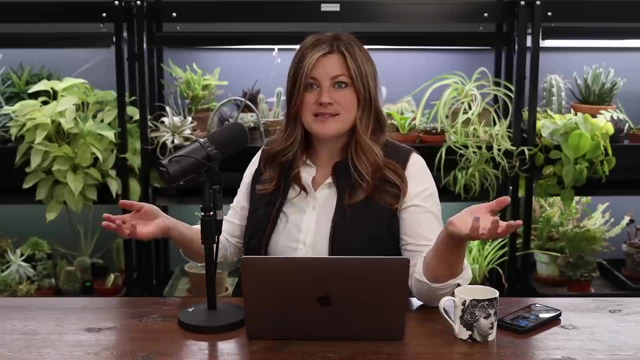 landed on anything that you actually definitively want, Because I don't do a plan. That's probably why, like in my mind, everything works out Like, yeah, just figure it out, Everything works out and it ends up being nice, and you know. 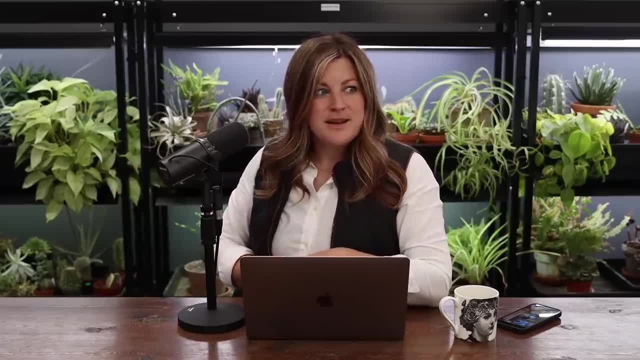 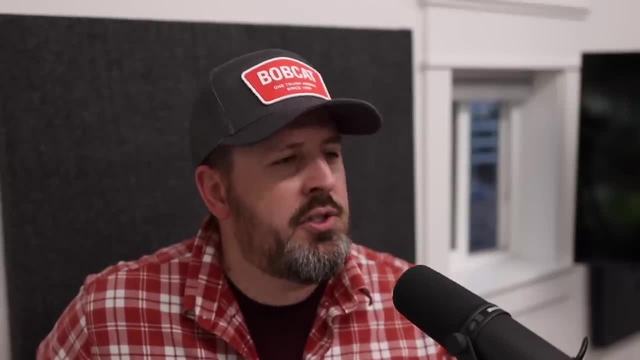 we might have to move one or two things along the way cause it didn't get it quite right, But in the end I think it'll be good. I think when I'm trying to explain, like impart a vision to someone, I want to give them the goal of what I'm shooting for, so that they can. 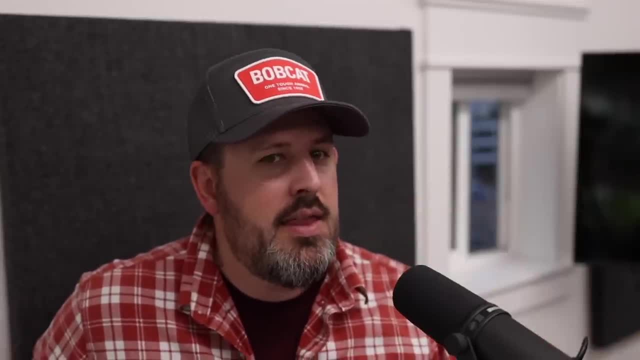 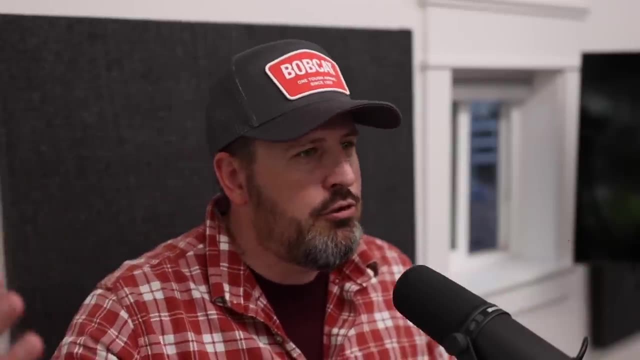 understand, you know why I'm doing something, and then like maybe I don't give it exactly definitive, but I'm like we could put a locust or a pine or a tall juniper or or weeping Alaskan cedar. I gave you a definite. 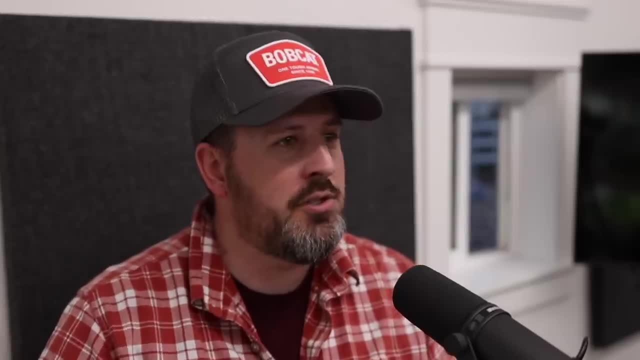 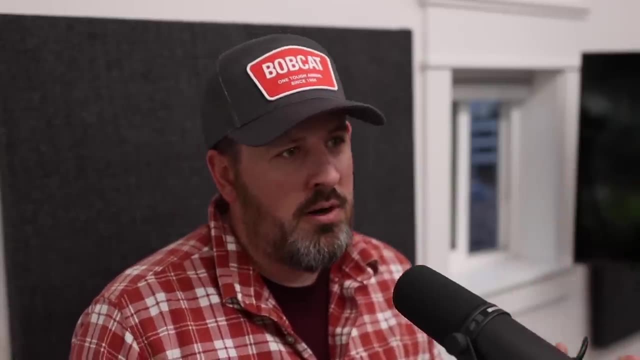 Well, that's so narrow, So it's like that, plus what other five trees are you going to plant? other things that are pretty cause. like a pine will take up a ton of space, but weeping Alaskan is going to take up like four. 15 wide. Yeah, Oh, I think you have the wrong plant. Yep, Weeping Alaskan cedar Jubilee, The one I planted gets 12, so they're wearing gets 15.. Yes, sir, I'm thinking of the wrong plant. 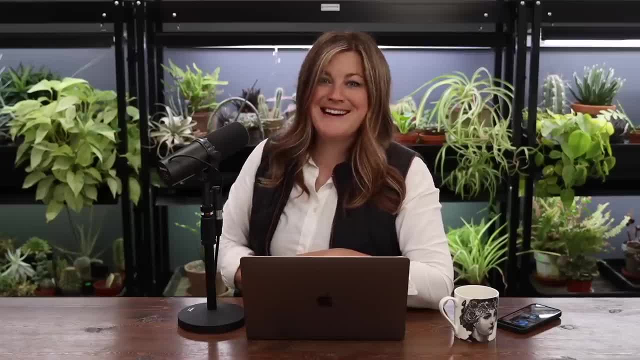 Then see, you just don't know your trees. No, I don't know my trees, apparently. How and how tall do they get 25. Do you approve? Well, okay, So what other? so 15 doesn't cover the whole thing. What other? what other three trees are you going to plant, or one or two that are big enough? I got to get my anchor plant in and then I can figure out the rest. The problem is is it takes you like three years to find your other plant. 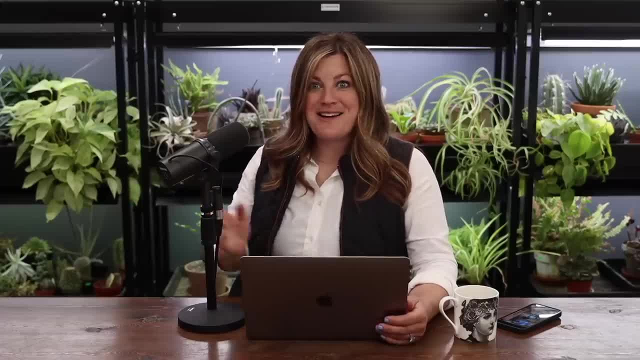 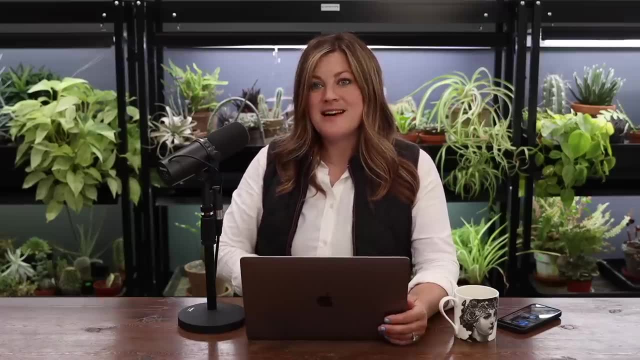 Maybe, but that is because there's so many other projects going on. I plant stuff everywhere. I mean, you guys see it right, Like there's just there's always activity. That's like not because I am not, cause you're not doing stuff. 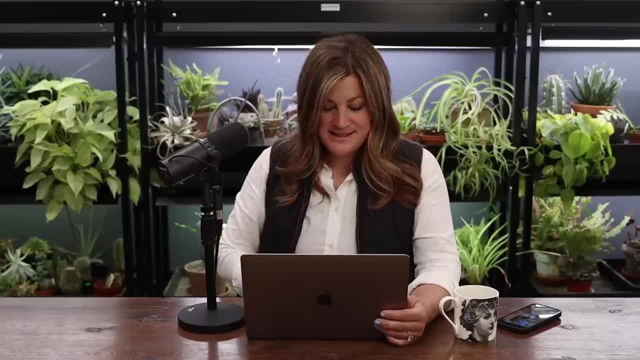 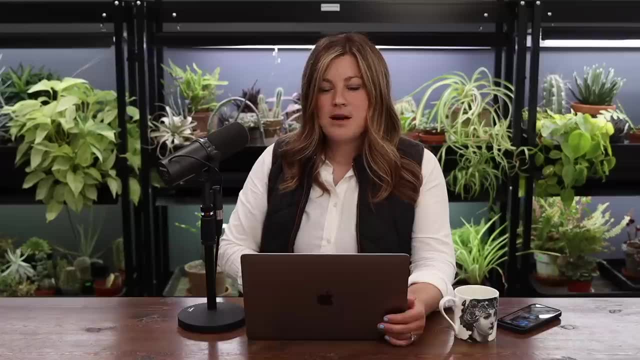 It's. yeah, You're a busy girl. Some days Hotel designer said: how many years would you estimate max tree height with, Oh geez Um, the honey locust? I don't think I can give you an average, Yeah. 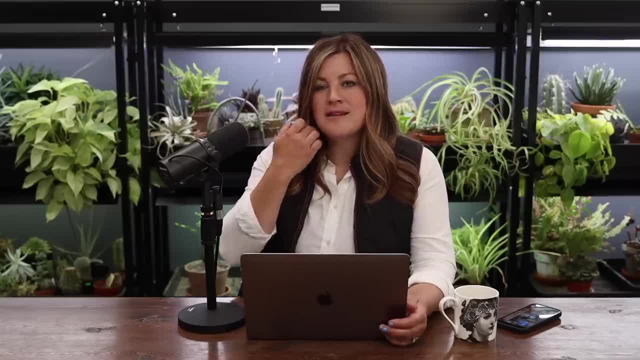 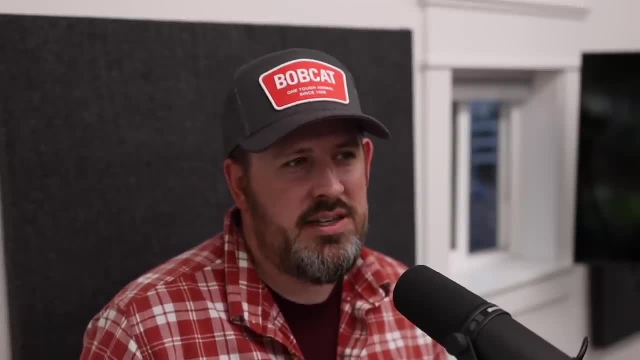 I just throw it through a year out. Yeah, I don't know I it just depends on the type of tree. I mean, if you're talking to the honey locust, it could be you probably see like pretty close to max at maybe like 15 to 20 years. Maybe it depends on if it likes it. Yeah, It's true that there's so many different factors. Is it getting enough sun? Is it getting enough water? Is it getting proper care? You know all of those things. That's a really hard question. 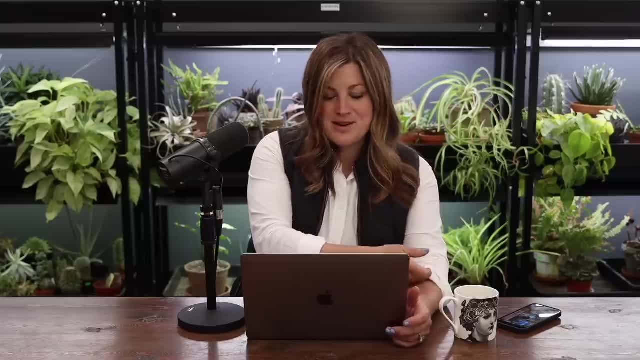 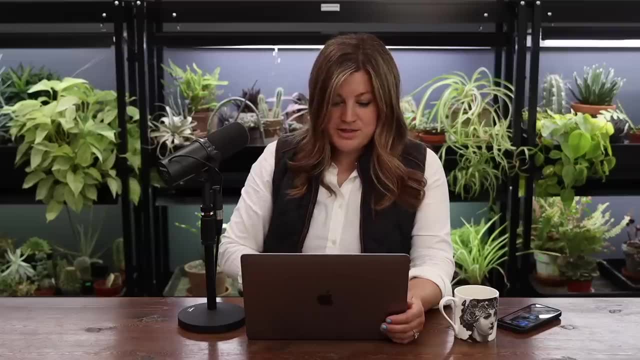 It's kind of like: how much water do you give this plant? You know it's so different for you know, depending on where you're at, what your soil composition is. two gallons every 36 hours. I wish that you could answer it that way for sure. 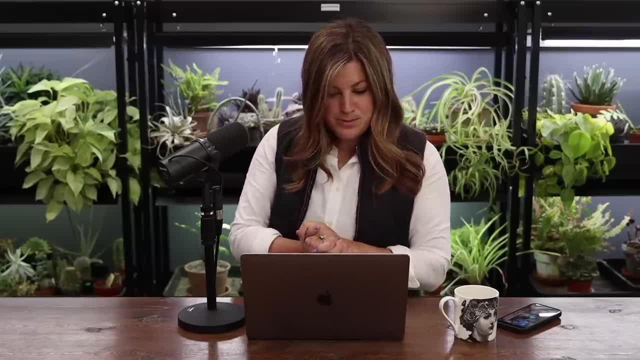 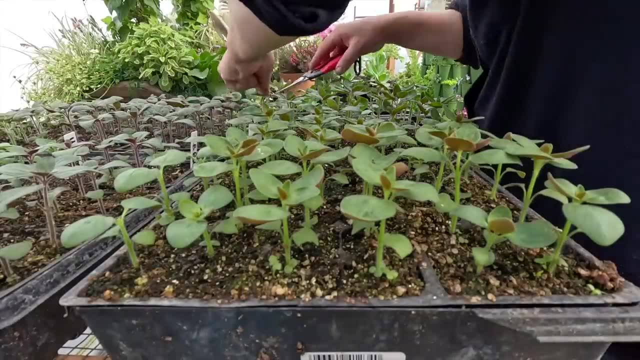 Okay, Last video is pinching snapdragons, simple spring containers and transplanting Iris. So we started at the greenhouse, We pinched our snapdragons. I show you how I do that and why we do That. we went around and filled up some containers with just pansies and I just love it. 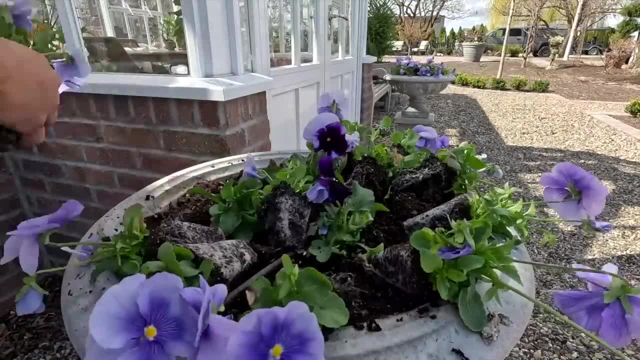 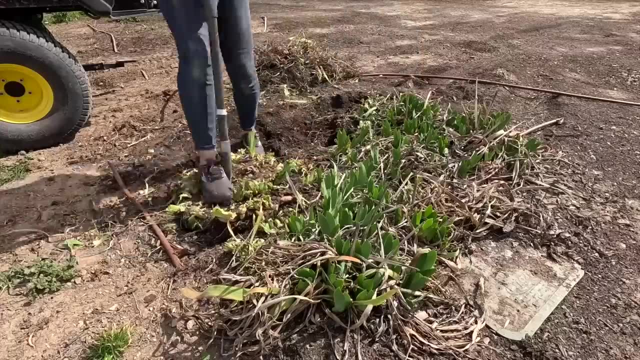 It's just so fresh and just colorful, but not complicated. And then there was a big patch of Iris right in the area where the lane is also going. So we got those all dug up and uh, Katie, uh for my friend. 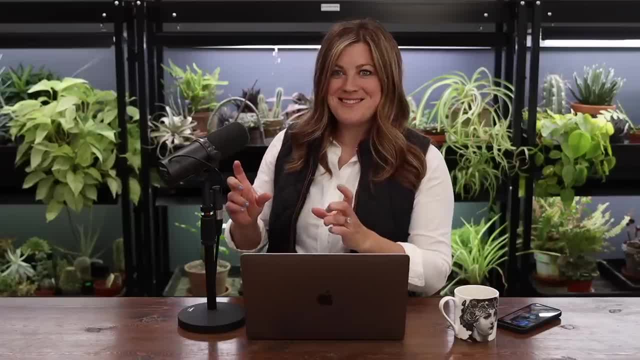 Katie texted me. She's like they are black. She screenshot, did a screenshot of the, so she was watching that video and I said I don't know. I think they're a black Iris, but they might be white or yellow. 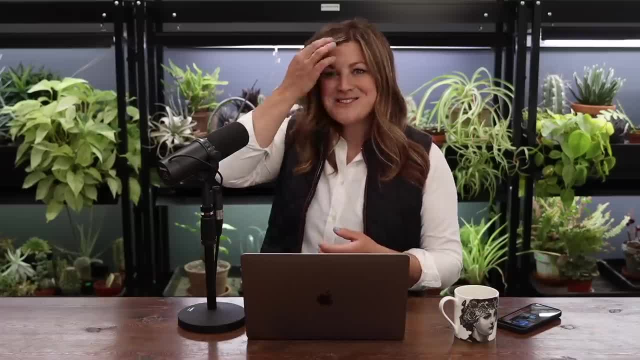 I'll have to watch a tour And she watched it and found it and took a screenshot. Yeah To send me. So they are that super, so dark purple, They look black. They're really pretty, Um, Judy Graham said. 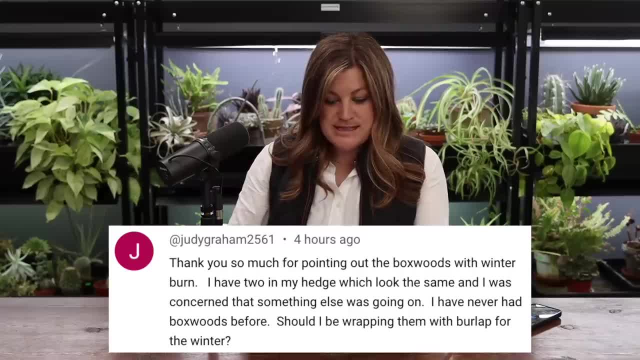 thank you so much for pointing out the boxwoods with winter burn. I have two in my head which looked the same and I was concerned that something else was going on. I've never had boxes before. Should I be wrapping them with burlap for the winter? Do people wrap burlap, uh, box boxwoods? I don't know. I think in a harsh climates they do. Yeah, That might not be a bad idea. I you know it depends on how old they are to their baby, baby ones that aren't quite as established With a good root system, that could be part of the issue. They might get too dry too, And I think we've got a lot of like boxes and containers that just stay too dry in the winter And so like the wind side. 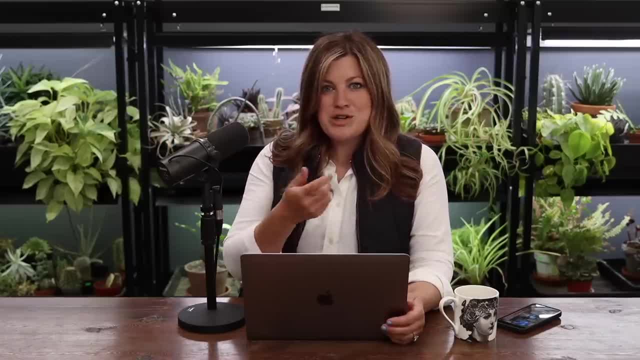 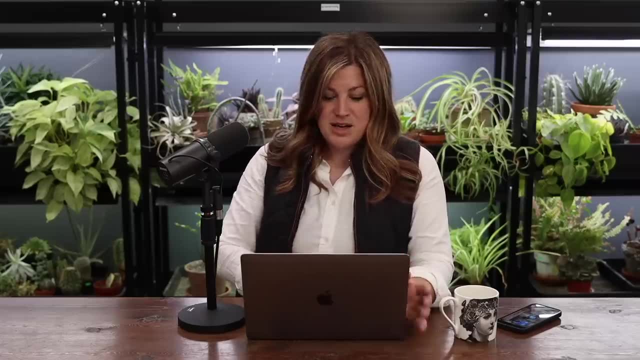 it doesn't have enough moisture in their leaves And so they're all winter like dried out winter burn on them, which, had they had more moisture in the pots, They probably wouldn't have done that. So it just there's so many different things that could be affecting that. 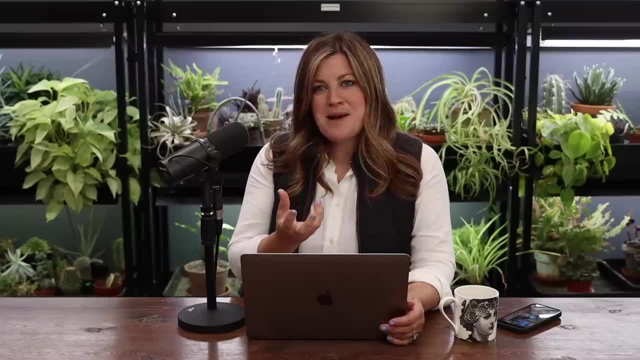 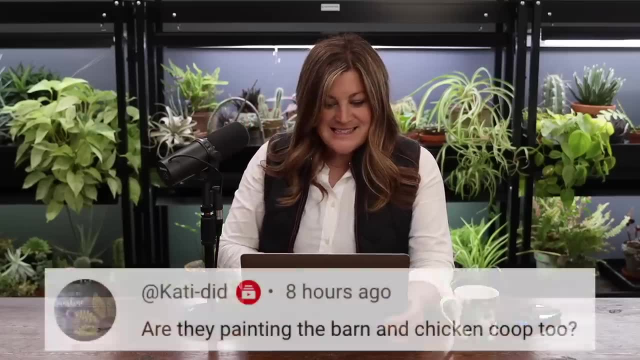 But our boxes aren't looking as bad as I thought. I think they're just like coming out of their bronze. I thought the green velvets weren't supposed to do that as much. Ah yeah, Katie did said: are they painting the barn and chicken coop too? 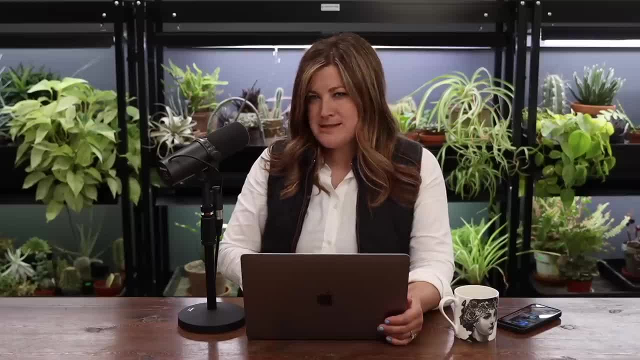 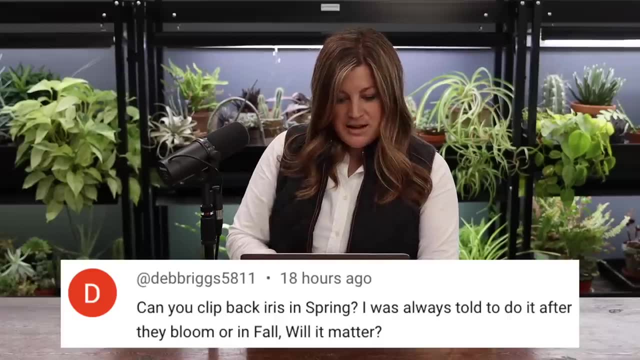 No, Um, the chicken coop could probably use a fresh coat. Um, but the barn was painted two years ago or so, So it's pretty good Same color. Deb Briggs said: can you clip back iris in spring? I was always told to do it after they bloom in the fall. 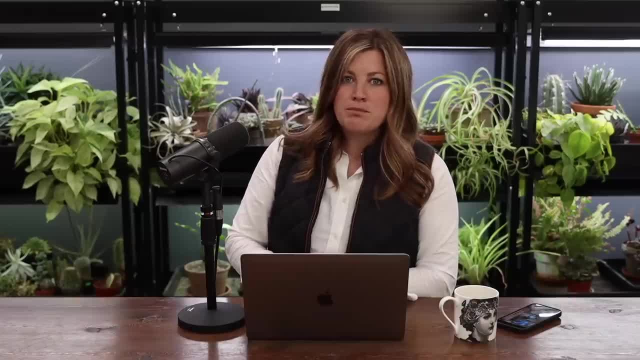 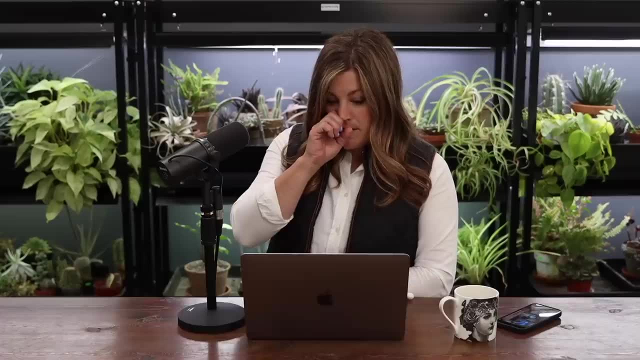 Will it matter? Oh geez. Well, I've done both and they bloom at the same time every year, no matter what Gail said. can you plant the kale by seed? Never seen any In my area. You can. there's a pretty strict grow, a growing regimen, though. 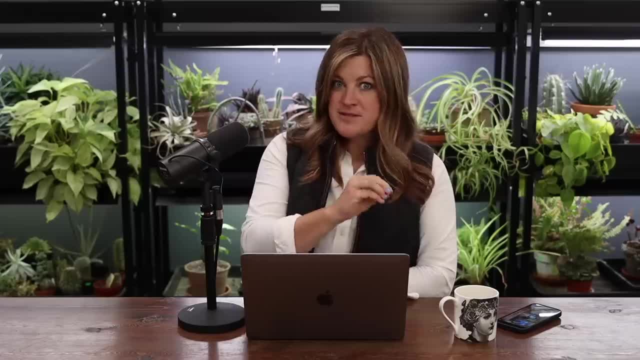 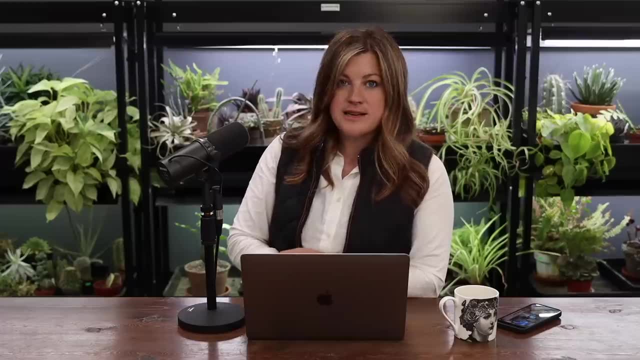 in terms of like once they germinate, and they need to be grown on at this specific temperature in order to, you know, keep that nice, compact shape. So it's something that I actually have- some ornamental kale seed um that I should get going for this. 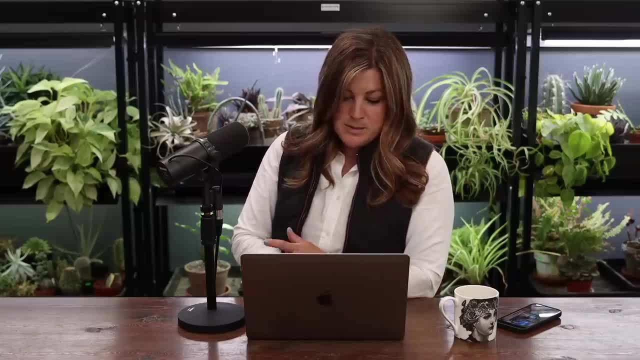 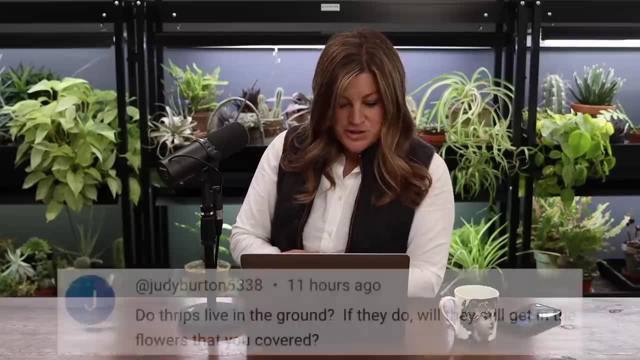 for this next fall season at some point and kind of show you guys the process that I go through, Cause I really haven't done much with that either. Um, but yeah can be done. Judy said: do thrips live in the ground? 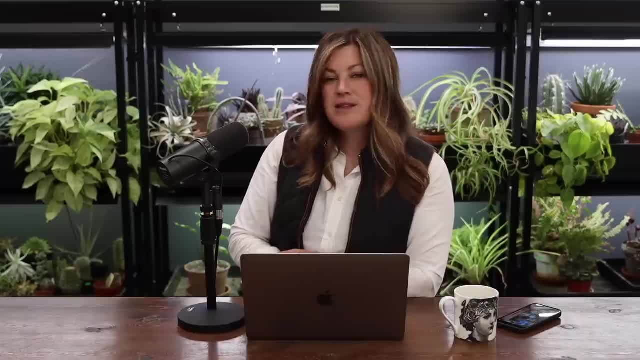 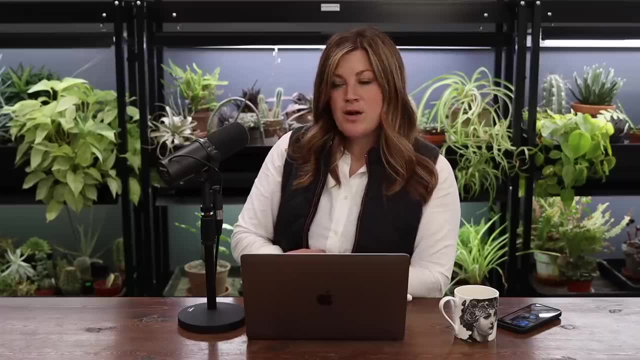 If they do, will they still get in the flowers that you covered? Um, they could. that area was cleaned out fairly well. We do have some more biologicals coming, Uh, so we're going to do another uh overhead application. 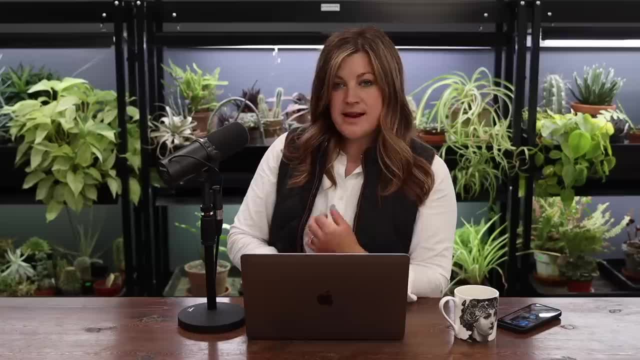 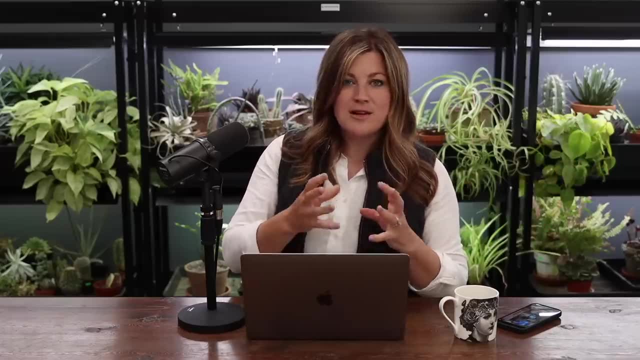 but we're also going to do some. they're packets that you hang, So I could hang them right to the um little low cat, um whatever hoops. I can hang them right inside and they're kind of like a slow release. 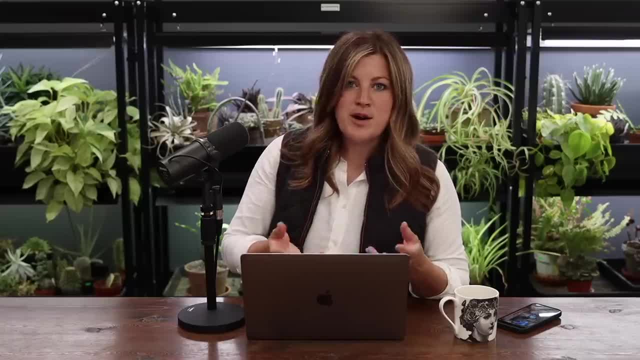 The biological, the mites come out really slow. Um, and it's not a spider mite like the type that eats your plant. They're a carnivorous, a type that eat thrips and white flies. specifically. Deb said who's having Easter dinner? 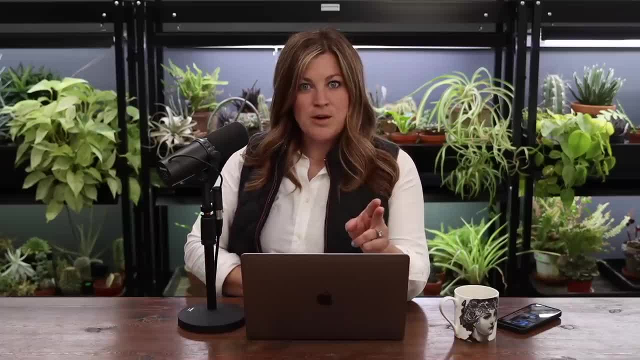 We're going to church in the morning, And then at one o'clock we're at my family's house for lunch, And then at five o'clock we're at your family's house for dinner. It's gonna be a full day and it's gonna be so fun. 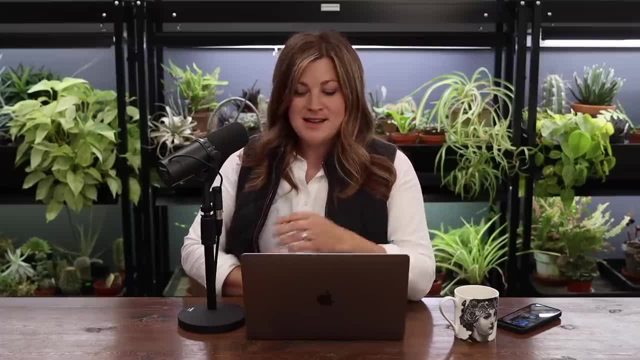 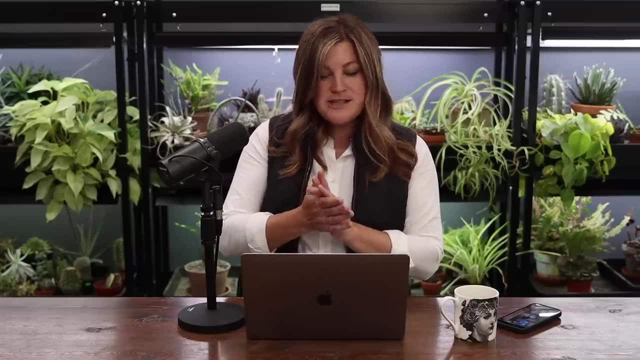 The kids will get to see all of their cousins, We'll do egg hunts at both houses and we'll get to be with all of our family. We're looking forward to it. And the very last video is spring fertilizing day. We just once a year. 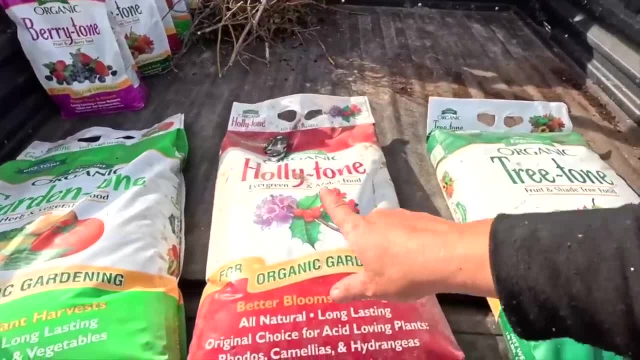 try to get a video out there in the spring When we do our big fertilizing day, just to show you what we do, We use, how we apply it. Um, and it was a. it was a group effort, Well, and Bethany came in. 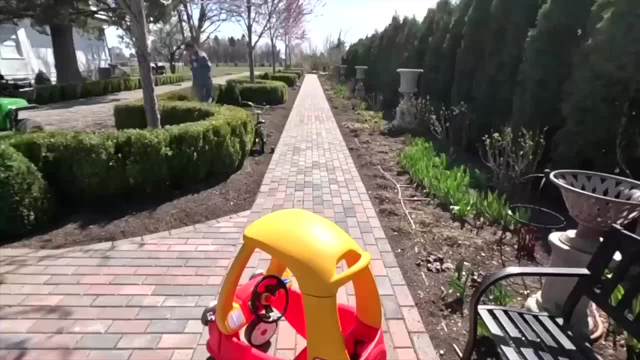 I always feel bad because she ends up coming into videos later on, you know, and I think she's going to be doing something else, but she ends up with time, And so I never say in the video, like Paul's, you know. 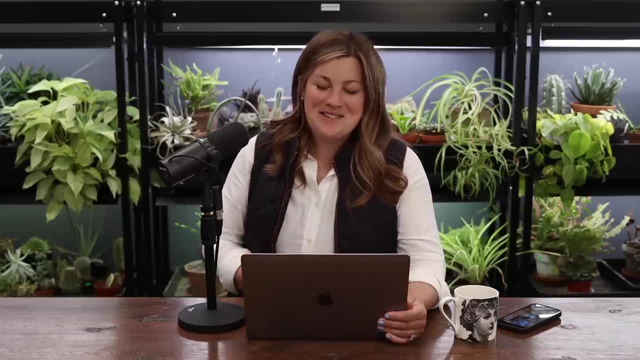 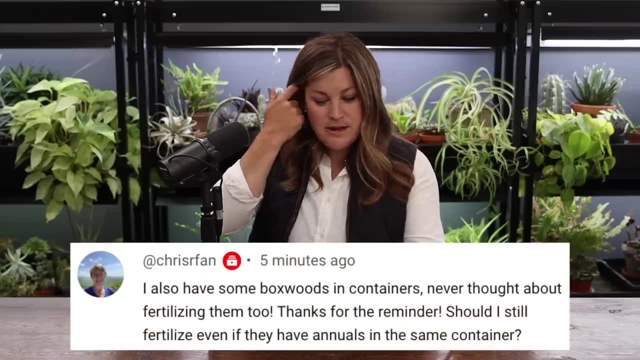 going to be helping us out instead of Paul and Bethany, but Bethany does a lot of it too. Um and so it was all four of us out there fertilizing, getting it done, Chris, our fan, said. I also have some boxes and containers. 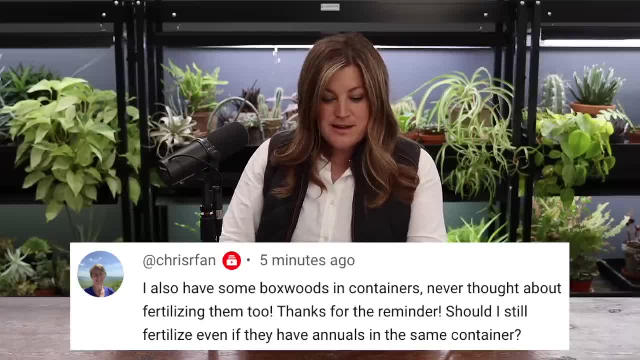 Never thought about fertilizing them too. Thanks for the reminder. Should I still fertilize, Even if they have annuals in the same container? um, I would give them a little boost right now, with a slow release And once you put annuals in there. 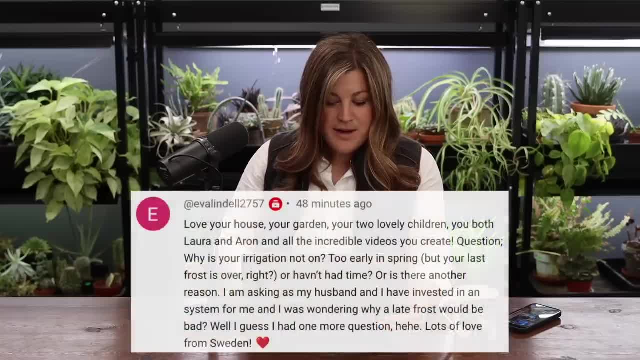 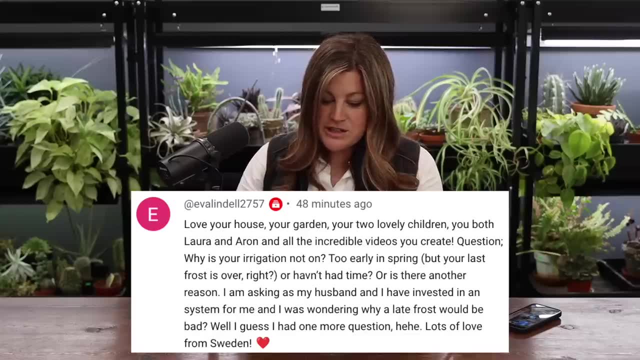 then I would do your weekly annual fertilizer. Eva said: love your house, your garden, your two lovely children, you both, Laura and Aaron, and all the incredible videos you create. That's so sweet question. Why is your irrigation not on too early in spring? but your last frost is over, right? Yeah, I think our last frost is. it's possible We could get one in April. Our average last frost date is April 29th. We haven't had a frost for a week, 10 days. at least The answer to the question is that we don't need to run it. No, not yet. We get enough rain in the spring that we can last into May, Usually without it on. it gets more difficult because we have more pots going and 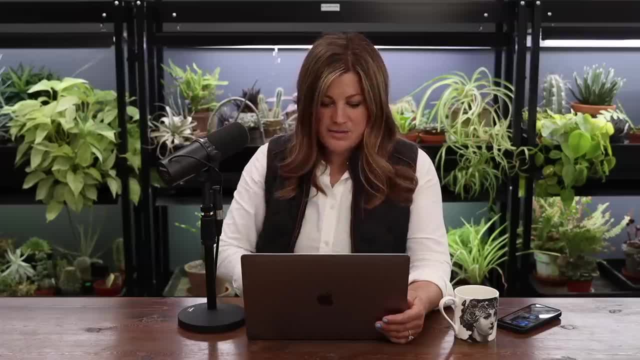 we have, you know, and it's nice to have water on So you have quicker access to stuff. There's been some years where it's been really dry, but not the last two or three. Right User said: do you never feed the daffodils or tulips? 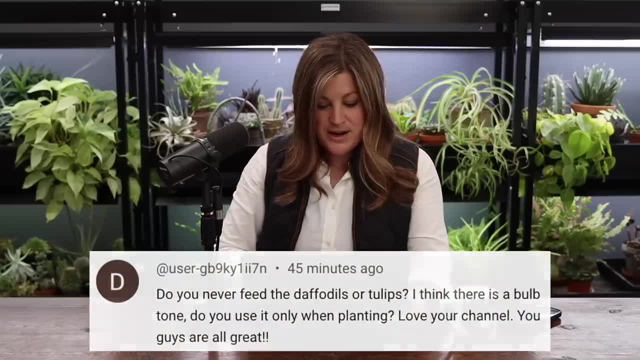 I think there is a bold tone. Do you use it only when planting? Love your channel. You guys are all great. Um, we do fertilize. I don't know that we hit it every single year, but you use bulb tone right after they're done blooming. because that's when the bulb is recharging for next year. So the foliage is still up, It's still looking green, It's still soaking in, you know, sunshine, creating that energy buildup, feeding them at that point really boost them up and get some. 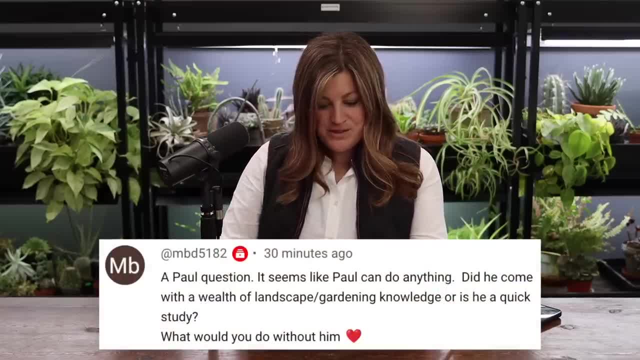 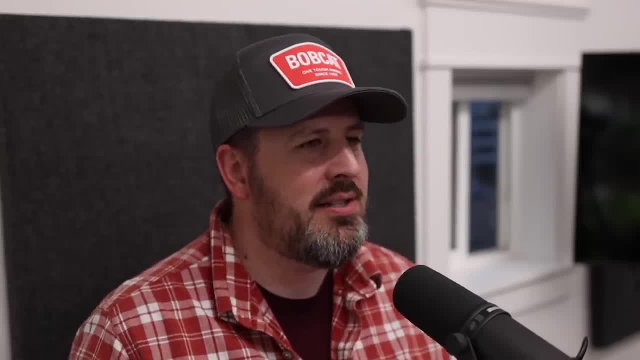 get some going. MBD said a poll question. It seems like Paul can do anything- Pretty certain He probably could. He's willing to jump in on just like. the thing I love about Paul is if you ask him to do something he hasn't done. 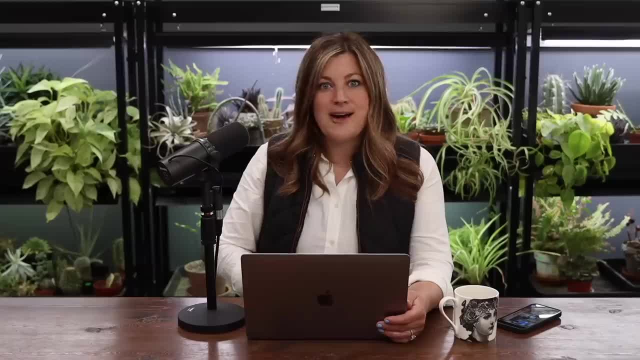 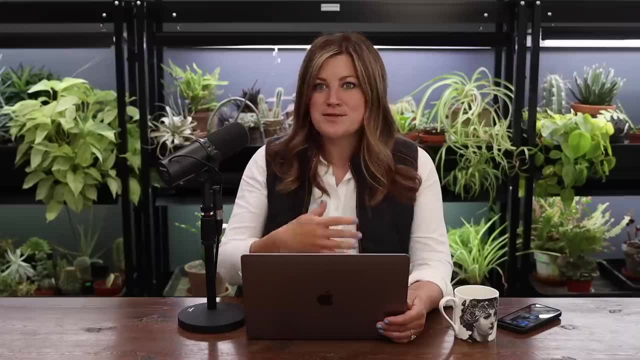 I see him go and he just like, pulls up a YouTube video, He figures it out, Yeah, Yeah. Or like he'll call um, he'll call around town, Like if you know, yeah, he's not afraid to go out there and search for. 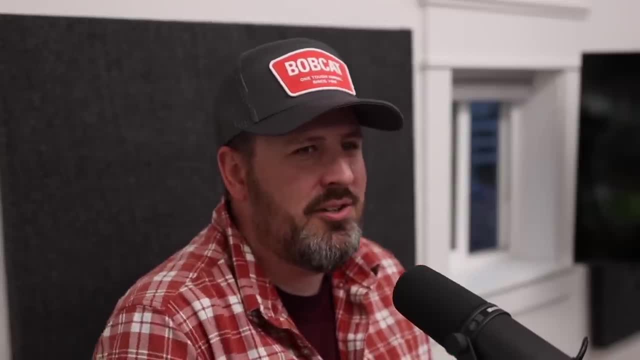 you know and talk like: Oh, we need to rent a thing, You know. it's like if you need to get something done, he'll just like, Oh, we could probably rent something to do this or that or whatever. Did he come with a wealth of landscape, slash gardening? 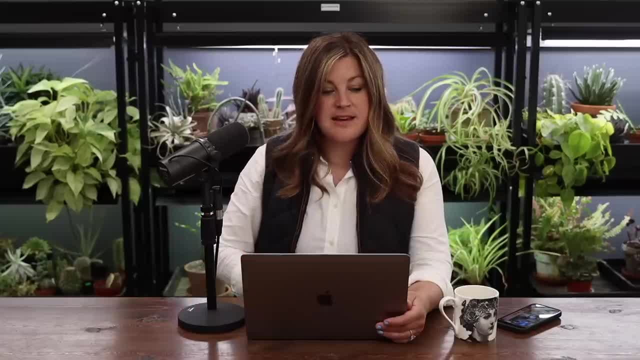 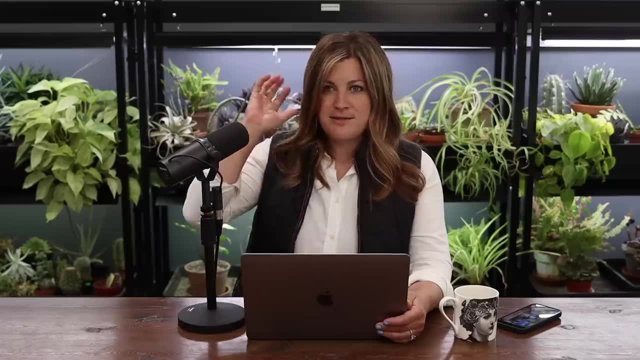 knowledge or see a quick study. He's definitely quick study. I think he came with a lot of farm kid kind of knowledge. You know when you grow up kind of doing that sort of thing. there's a different kind of mindset, a lot of common sense and just like mechanical. 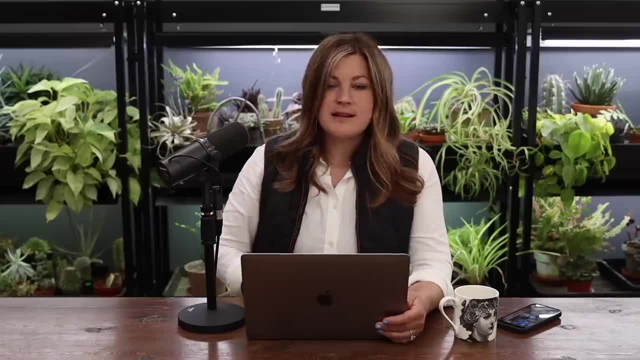 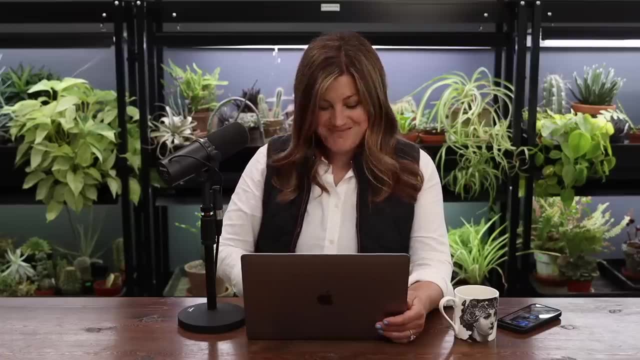 his cars are his passion, Um, and he likes like working on his cars, Yeah, And I think that's kind of how his brain works, which works out great for us. Really hard worker, Both of them. Wendy said: how come you never speak of the aroma of the?